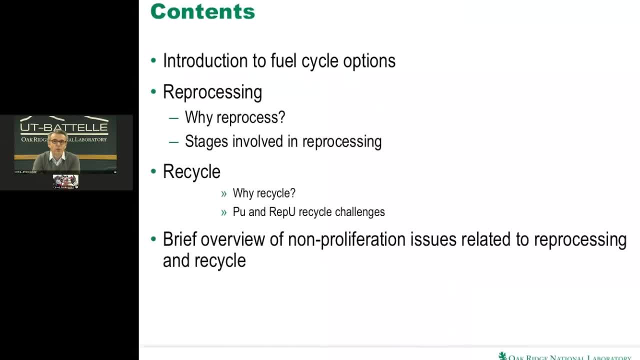 And then what I also wanted to do is just touch on some of the nonproliferation issues related to reprocessing and recycling. Again, that in itself is a huge topic that we don't have time to cover today, but I will touch on some of the elements of that and how, despite kind of popular belief, reprocessing can and is being done under a safeguards regime and there's no issues associated with the nonproliferation. 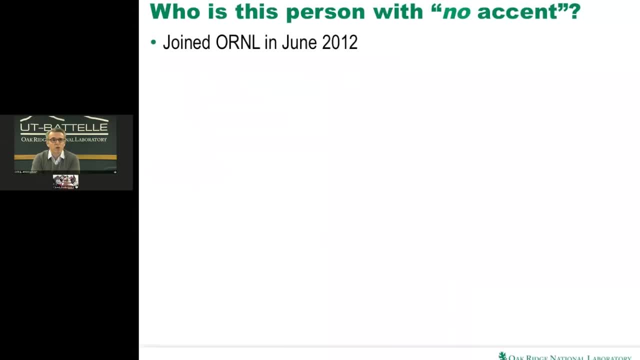 And then finally, summary and conclusions. So, despite what you may think, I have no accent. It's you guys that have the accent. So I actually have been with O&L just for the last two and a half years. Prior to that I was with the UK nuclear industry. as you can probably tell by my accent, I'm not from East East East Tennessee, I'm actually from the UK. 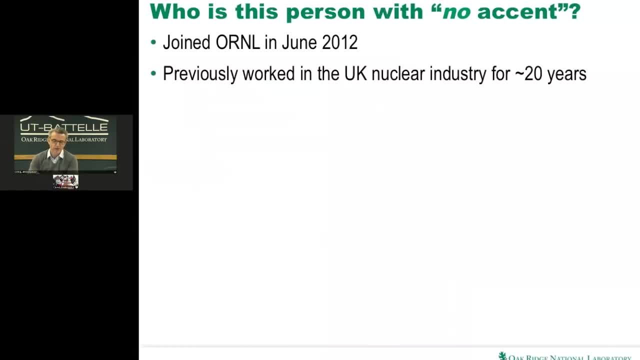 So I work for a company called British Nuclear Fuels Limited, BNFL, who actually no longer exists. So, depending on the age of the audience, you may never even have heard of them. But BNFL was an equivalent company to Arriva. So BNFL were involved in everything from fuel fabrication to operating reactors to then taking the spent fuel and reprocessing it. 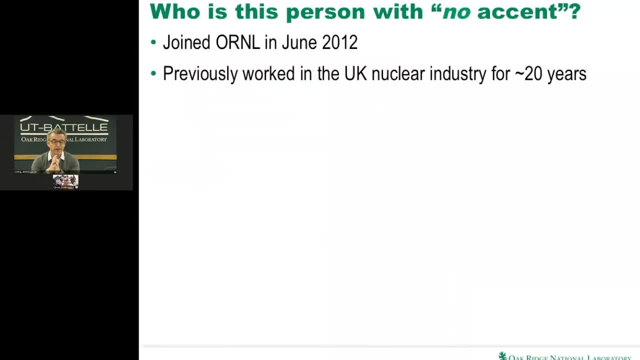 That was a commercial business For many years. BNFL was the largest earner of Japanese yen, for example, for the whole of the UK because of reprocessing and then dealing with the waste management issues and the back end of the fuel cycle and so on. 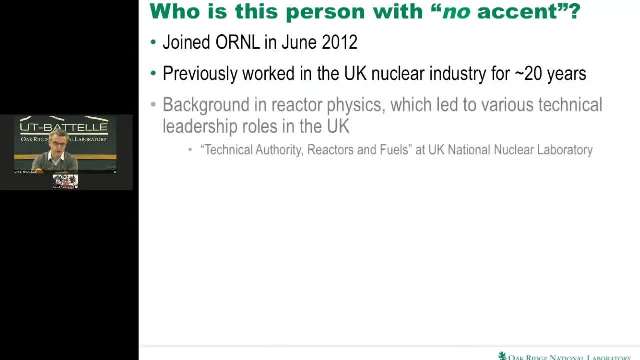 That was BNFL's business, So I used to work for that organization And in fact my background is not reprocessing or indeed anything to do with the fuel cycle exactly. My real background was reactor analysis, reactor physics, But very quickly I got involved. 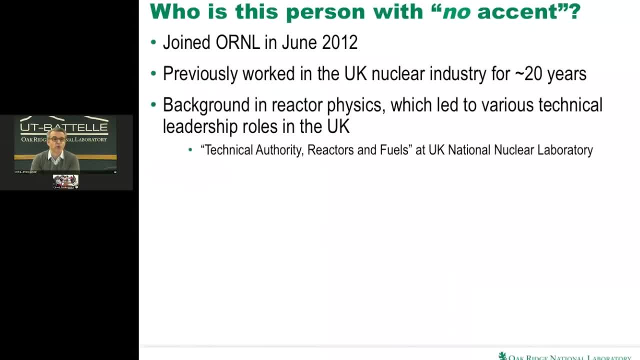 Then BNFL's broader business which was plutonium management, And as part of plutonium management and the potential to put plutonium and recycle that in reactors, which I'll talk about shortly- then suddenly you get involved in much broader aspects of the fuel cycle, including weapons, plutonium disposition and so forth. 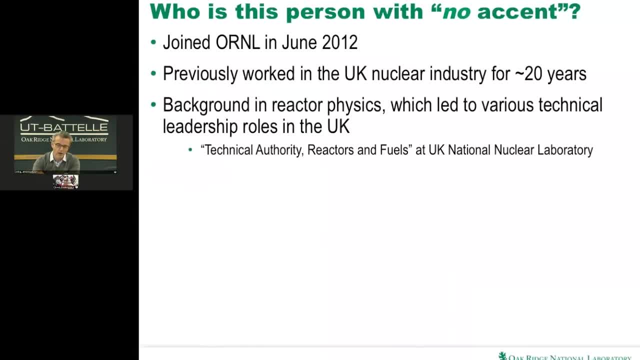 And then I spent a lot of time working my way up to eventually I was part of the UK National Nuclear Laboratory where I was the technical authority for reactors and fuels, advising the UK government on plutonium, as I mentioned, But also so a new nuclear build, advanced fuel cycles, thorium fuel cycles and a whole range of other things. 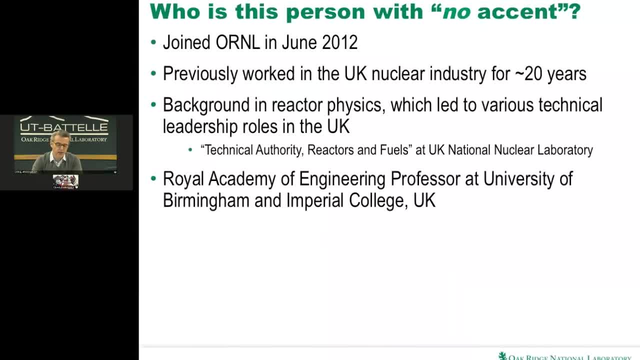 I also got involved in a whole range of academic lectures and so forth and I was a Royal Academy of Engineering professor at two of the leading UK universities. But in general my interests in nuclear are very broad and wide. I'm very fortunate that I've done everything from press my own fuel pellets. 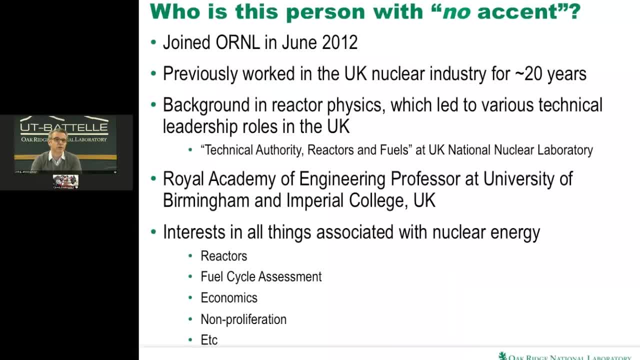 I've seen plutonium being fabricated into new fuels. I've seen commercial and fast reactor fuel sheared and reprocessed. I've been very, very fortunate in my career, so hopefully I'll try and explain some of those operations and experiences that I've got to you today. 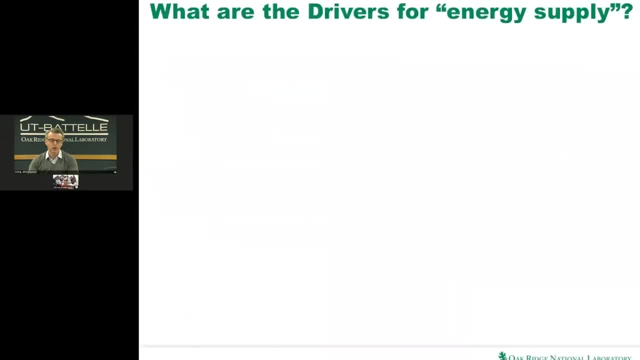 Okay, so introduction to the fuel cycles. What are some of the drivers for energy supply? If you just think for just a few minutes and put yourself in various people's shoes and look at these different perspectives, whether that may be in operating units, 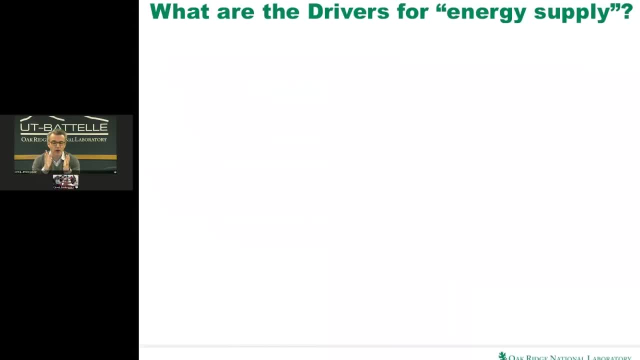 whether that may be a utility, whether that may be a government, a vendor, whoever it may be. There's a whole range of different things that you need to think about in terms of energy supply, And the classic one everybody would typically think of would, of course, be the economics. 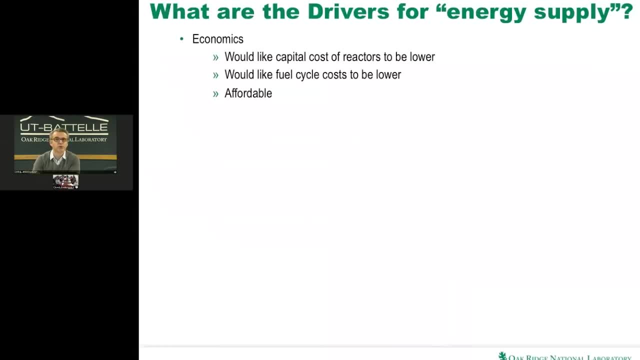 You might look at reducing the capital cost. You want the fuel cycle cost to be lower and of course, overall it has to be affordable, Otherwise you wouldn't consider it. So that's one of the drivers for future fuel cycles. 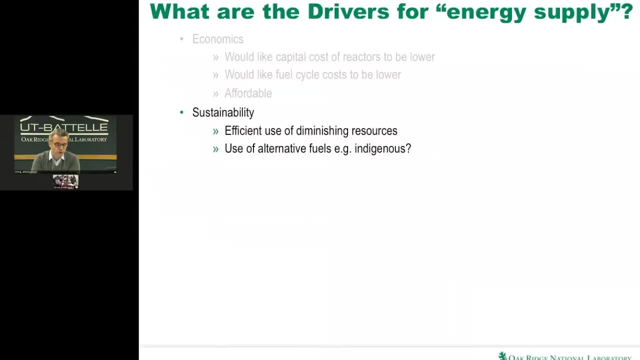 Sustainability is becoming ever important. The US is in a very, Very fortunate position that it has a huge supply of natural gas and oil. not so much on uranium: It's only produced something about 9% or 10% of the world's uranium. 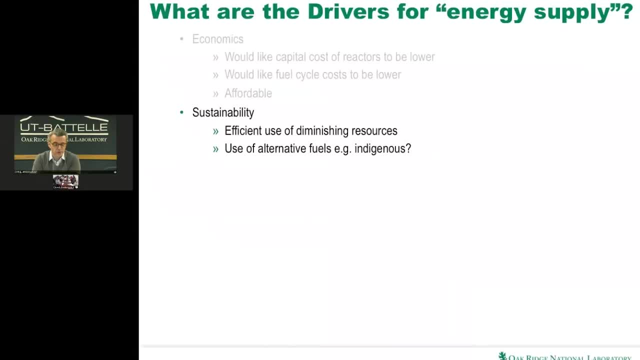 But something the US will need to think about in the future- not too distant future- is sustainability and coming up with future energy options, including nuclear, that are sustainable, And I hope we all agree that we need to do more with the resources we have. 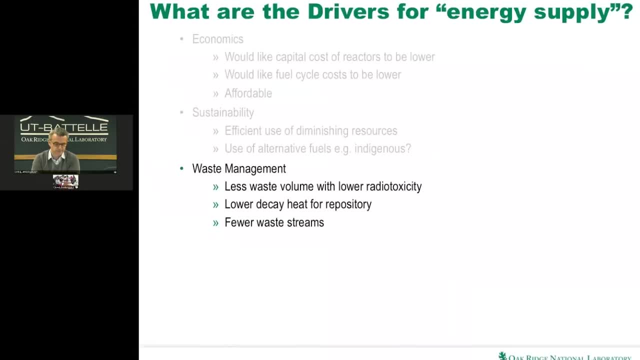 rather than just waste them just simply because we have them at our disposal. Waste management is something that everybody always talks about with nuclear, and quite rightly so, And I'll touch on some of the details later. But some of the drivers for future energy growth from a nuclear perspective are things like repository performance. 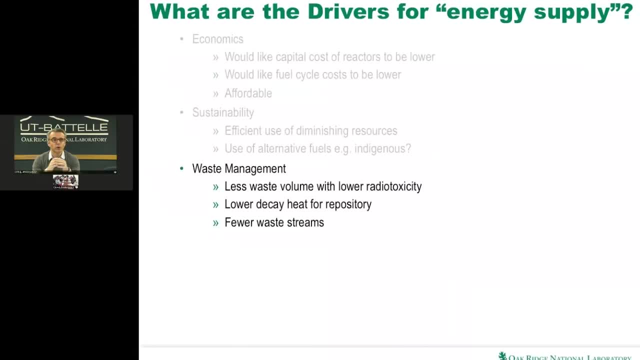 making sure something like intergenerational equities It's called- we don't pass on our problems of this generation onto future generations. So dealing with the waste is incredibly important and how we fix that. Of course, safety is really important, and that includes not only operational safety for the public. 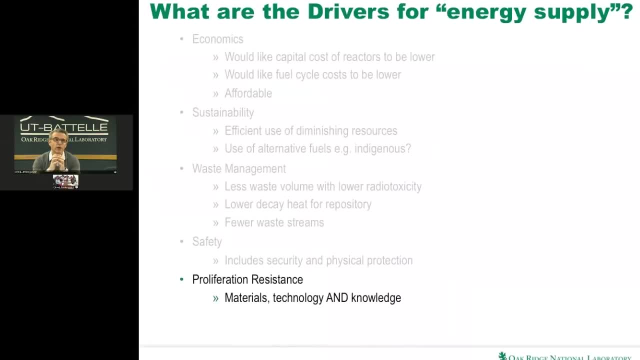 but also security and physical protection. And of course, it wouldn't be right to talk about these things without thinking about proliferation resistance. But also, what does that mean non-proliferation? Well, it means making sure bad guys don't get the materials, but also they don't get the technology that they can misuse. 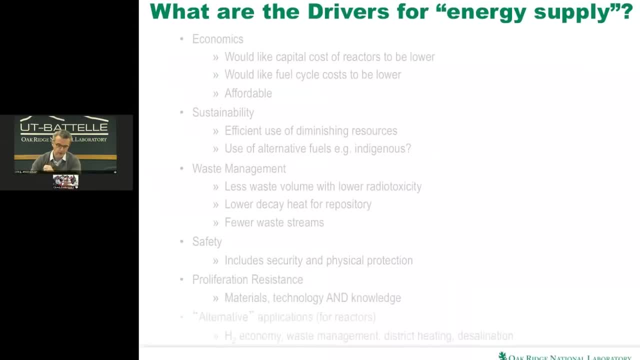 and also the knowledge that they can misuse. We have to protect all of those. And then the final thing we need to think about with energy supply, particularly again, for the role of nuclear is broader than just electricity, And again, this is something other parts of the world are desperately thinking about. 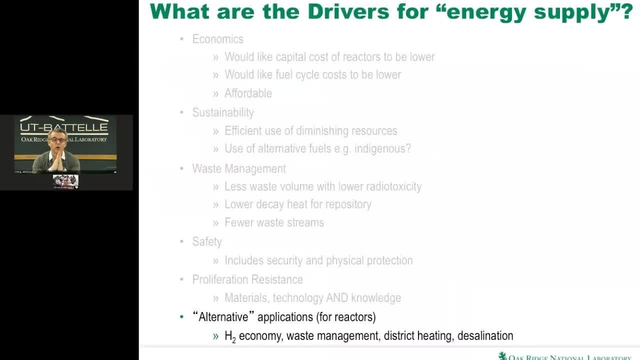 For example, if we look at the water demands around the world and the ability for potable water in Africa, it's a very, very small percentage of people who have the access to clean water. So things like nuclear for desalination is incredibly important, not for electricity generation. 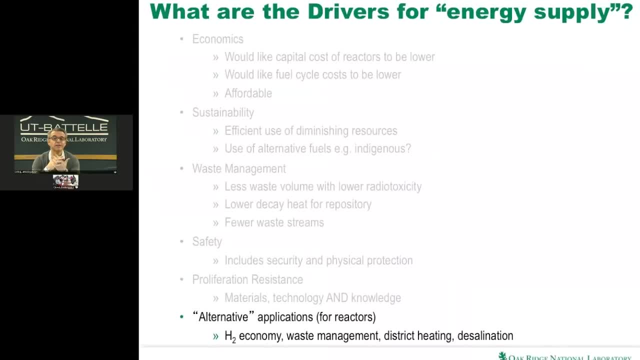 In some parts of Europe, in the Baltic states, district heating is incredibly important, And also things like hydrogen economy, even for transport. So all these things are broader concerns, questions, challenges we have to address When thinking about nuclear, And what that means is when evaluating and considering a fuel cycle option. 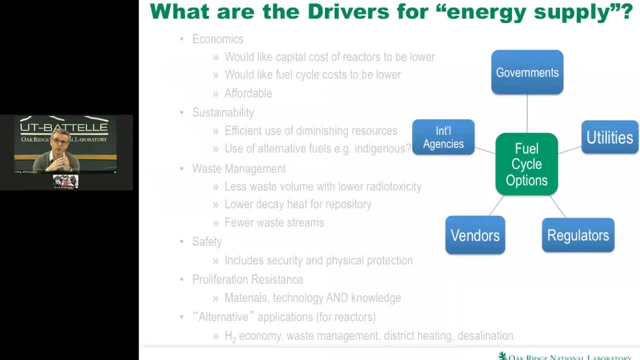 we need to think of it from all these people's perspectives. As I said, the operators, the governments, the international agencies like the IAEA, but also regulators, vendors- you know that people want to make money out of this as well, as you know- for the good of mankind. 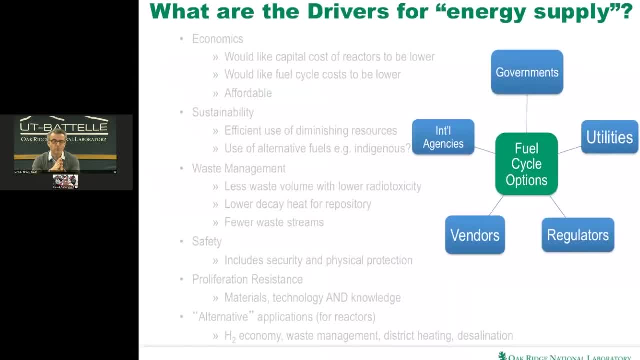 So the reason I mention all of that is that if we're not careful, what we end up focusing on is: oh, what's the most technical, what's the best technical solution- not necessarily the best economic solution, or we don't necessarily think about it broader in terms of how else this nuclear fuel cycle can have benefits. 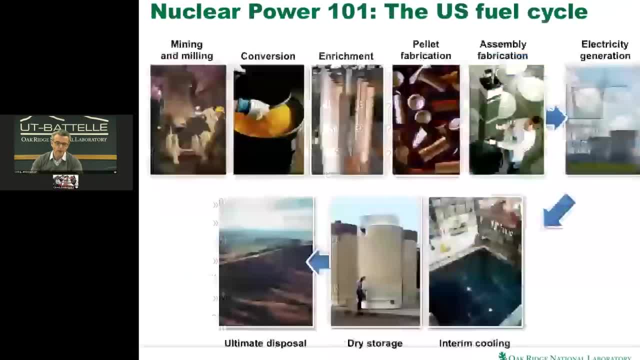 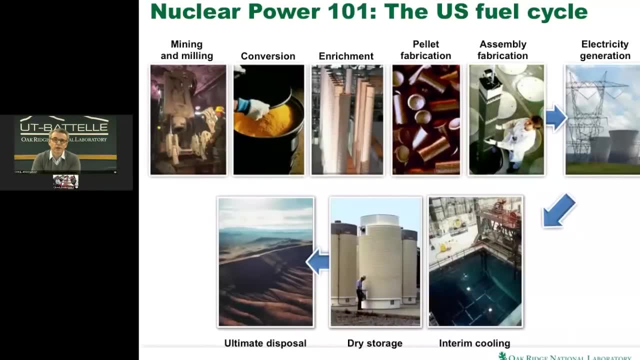 So that's why I wanted to mention that upfront. So I'm sure most of you probably have already seen something like this before, but I just wanted to make sure we were all on the same page. If you look at the current US nuclear fuel cycle, it's pretty much what's known as a once through fuel cycle. 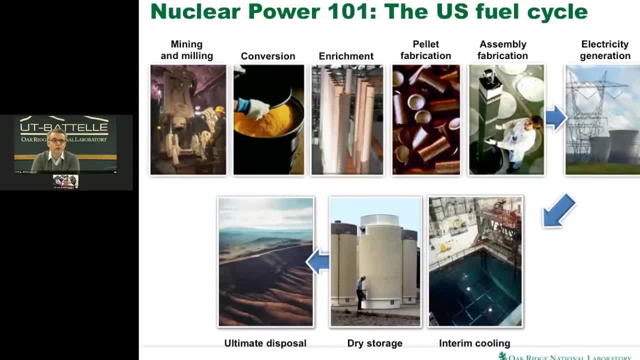 So, starting from the top left, we mine and mill the uranium Or we then convert into a powder that we can then turn into a gas to enrich from the natural U-235 of 0.7 percent, typically enriching to something like four and a half five percent in most current commercial light water reactors. 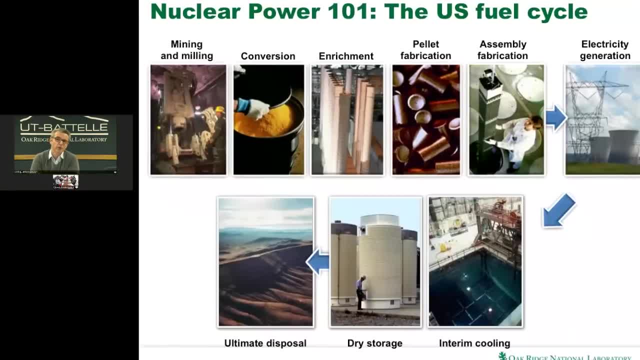 We then make that enriched product into fuel pellets and then we put those into assemblies, generate electricity, And then this is where the fuel cycle kind of diverges. at this point We have two options that I'll start talking about. But in the US the direct. 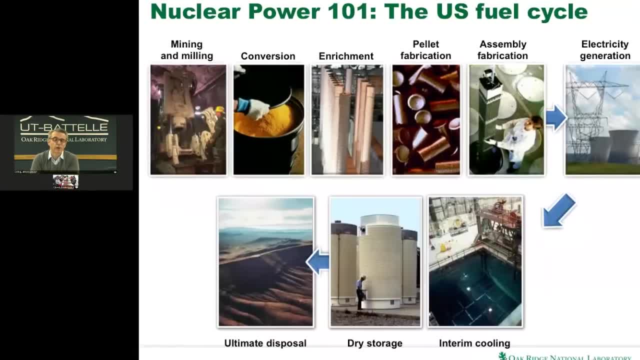 route currently is store the fuel for a period of time in interim cooling at the reactor sites in pools and then potentially have to dry store that as we fill the fuel pools up at the reactor sites And then finally ultimate disposal in something like Yucca Mountain. 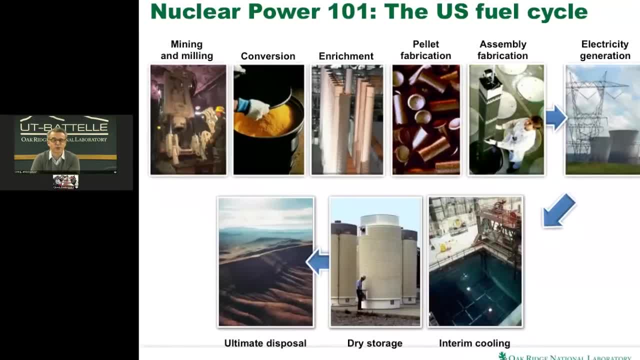 And again, that's a whole other topic of what Yucca Mountain or alternatives look like, but that's not subject to today's talk. But the key thing here is just to bear in mind that when you look at the once through fuel cycle, 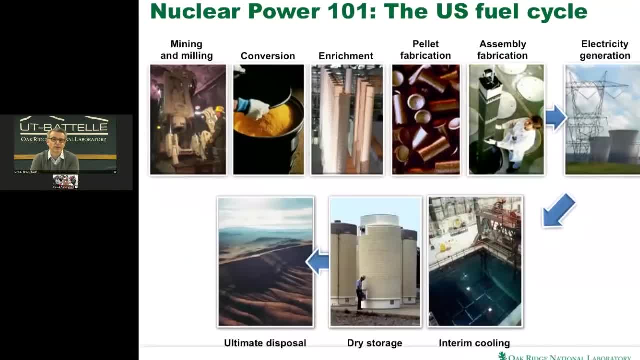 everybody thinks of that as being complete. Well, in fact it isn't. We as an industry, as a nuclear industry, haven't yet even demonstrated a once through fuel cycle, because we haven't yet done the ultimate disposal part of it, which is one of the major challenges for nuclear. 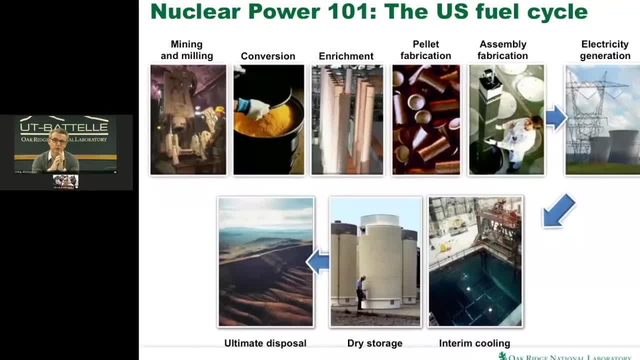 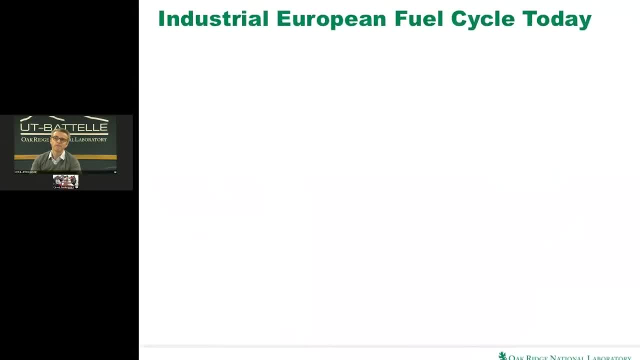 So when people start talking about reprocessing and all these facts in future fuel cycles, you would also have to bear in mind that we haven't yet done the once through fuel cycle completely either. So there's still plenty of challenges there. So if we compare and contrast, then that 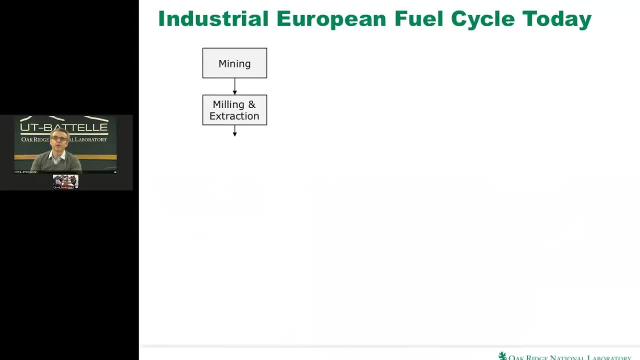 So I just talked about mining, milling and extraction, converting to uranium hexafluoride enrichment, then on to making fuel and then all the way through to reactors. What we call that is the front end of the fuel cycle. So anything from leading up to the reactor is typically known as the front end of the fuel cycle. 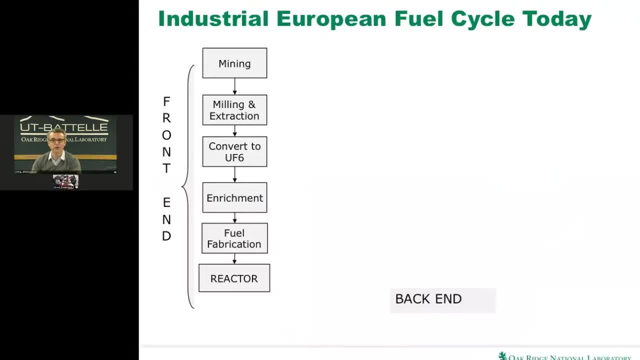 If you have a front end, then of course naturally you have a back end of the fuel cycle, And this is where the options kind of diverge. So what we can do is we can We can reprocess or we can store indefinitely. 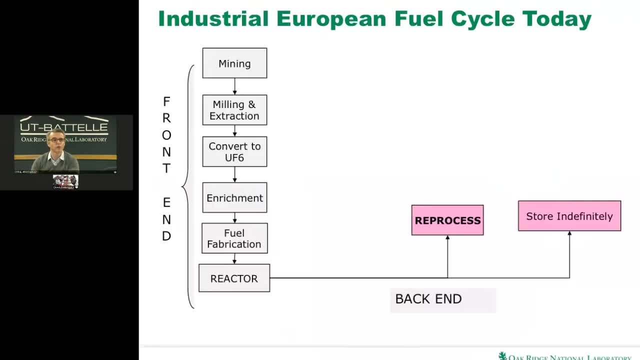 And, as I just illustrate on the previous slide, the store indefinitely is the current, once through fuel cycle, the US fuel cycle. If we're to reprocess in Europe, we typically have generated three levels of waste streams, known as low level waste, intermediate level waste and high level waste. 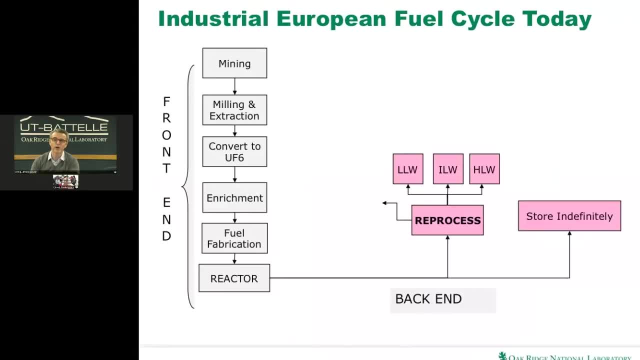 The classifications aren't so important. I just wanted to demonstrate. there's a whole range of waste streams, And if one of the two of the major byproducts we get from reprocessing, though, which we can do Something else with subsequently- I either recycle part of it- is we generate uranium and plutonium from the spent fuel. 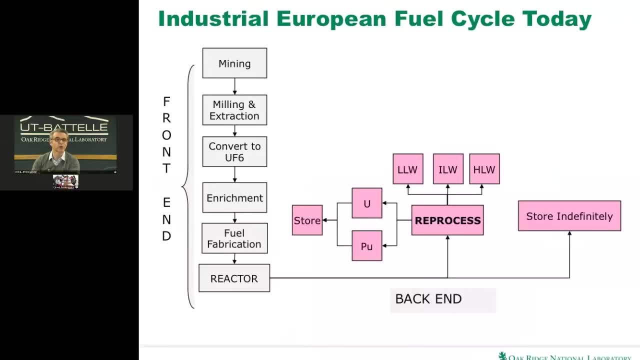 And typically we can store that And that's what's been happening, for example, in the UK has been storing that. But alternatively we can take that uranium and feed that back into the uranium fuel cycle and re-enrich and so forth. 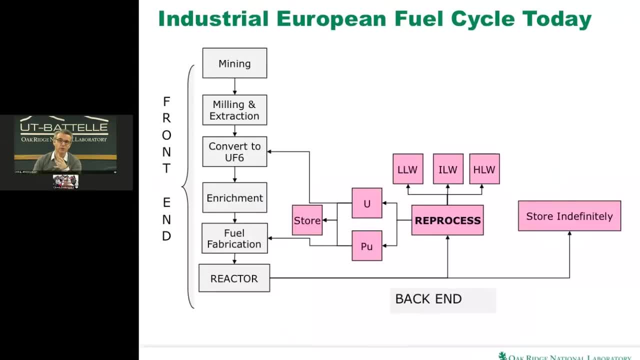 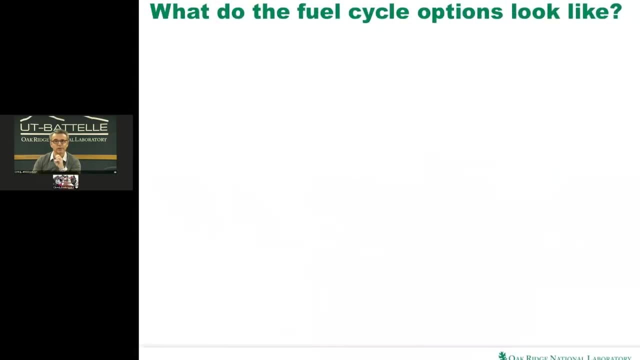 Or we can take the plutonium and make that into what's known as mox fuel- mixed oxide fuel of plutonium and uranium- and directly put that into a fuel fabrication process and back into the reactor. So, And those are the stages I'm going to go through in a little more detail, but I think it's worth giving you an idea of what that layout looks like before we start in the details. 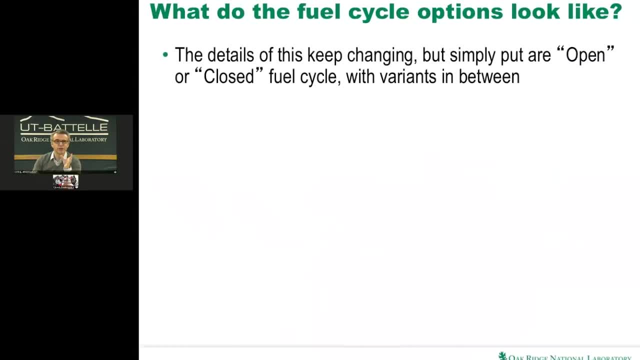 So There's a couple of different phrases you sometimes hear with fuel cycle options. Simply put, they're either open or closed is the two options. So the open fuel cycle or the one through fuel cycle, as I said, is the US basically take the uranium ore out of the ground, make it into fuel, put it in a reactor, put it down the hole in the ground. 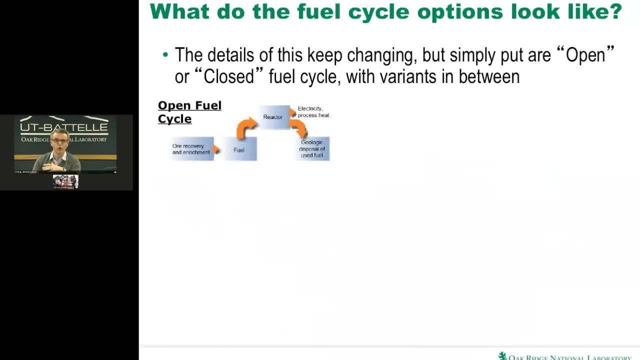 So the open fuel cycle or the one through fuel cycle, as I said, is the US basically take the uranium ore out of the ground, make it into fuel, put it in a reactor, put it down the hole in the ground. That's known as the one through or the open fuel cycle. 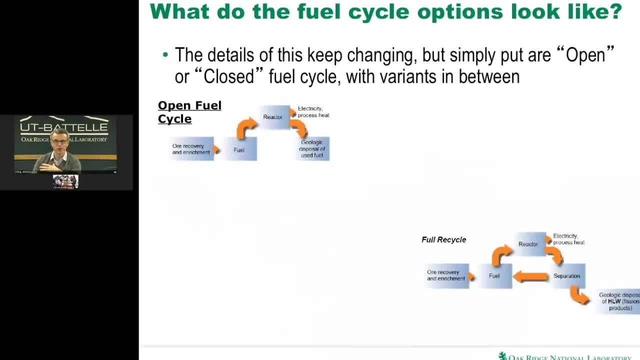 The full recycle option. But this isn't where we are today. This is where you need fast reactors and these fancy future reactors. is we again do the same thing: Recover the ore, make the fuel put into a reactor, but now we? we then recycle. 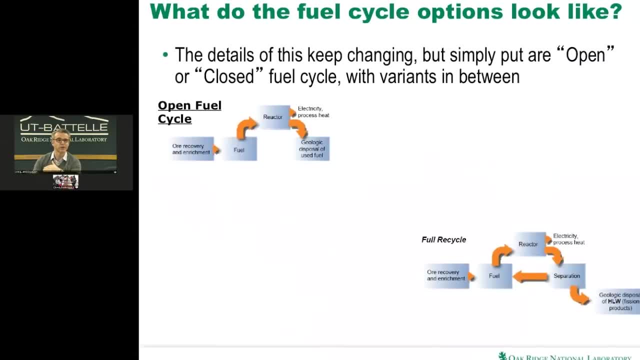 We separate first of all the good stuff and the bad stuff. the bad stuff, we don't want, put it down the hole in the ground and in the repository. the good stuff, we recycle its fuel And that's known as the closed fuel cycle. 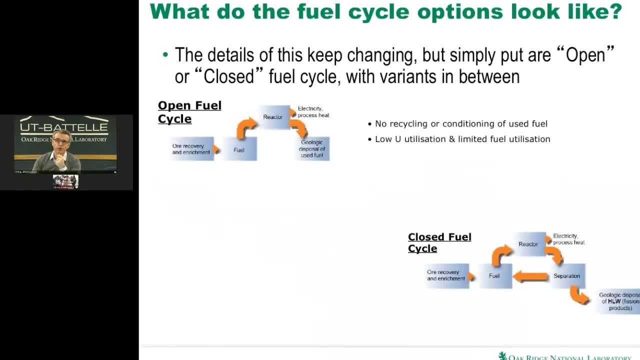 fuel cycle. So the open fuel cycle, no recycling or conditioning of the used fuel, which really means low uranium utilization. On the other side, though, the closed fuel cycle is, we can multiply, reprocess as many times as we can the materials and also transmutate the actinides. 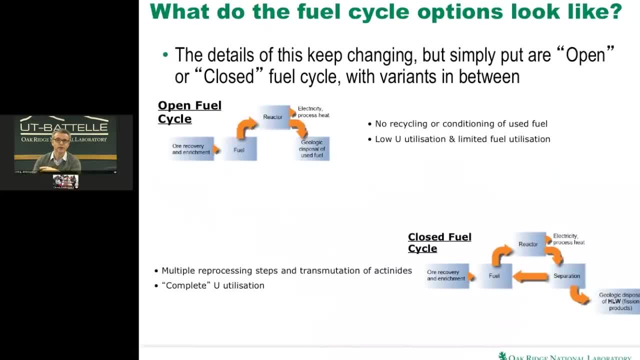 the minor actinides, as I mentioned, is one option and that's a complete uranium utilization. It's as much as we can possibly do And, just for your complete understanding, there are stages in between, which is typically called the modified open fuel cycle or limited recycle, as it's also. 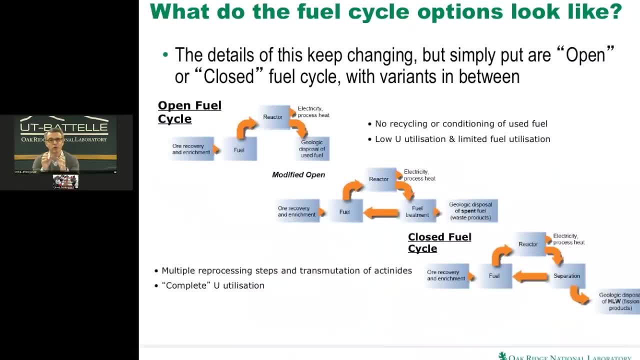 known, And that's pretty much what France is currently doing. France is right in that middle one, in the modified open, because what they're currently doing is they're taking the plutonium and the uranium and recycling it, but not to the extent where you can do that infinitely. 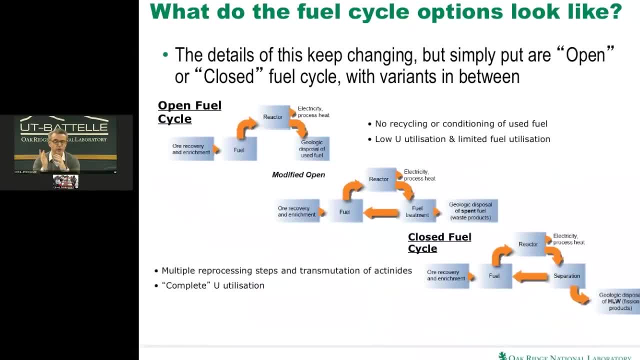 They're only doing that in light water reactors And again I'll touch on some of the details later. but you can only do that once or twice because of the fissile quality of the material you're recycling. And then the minor actinides and the fission. 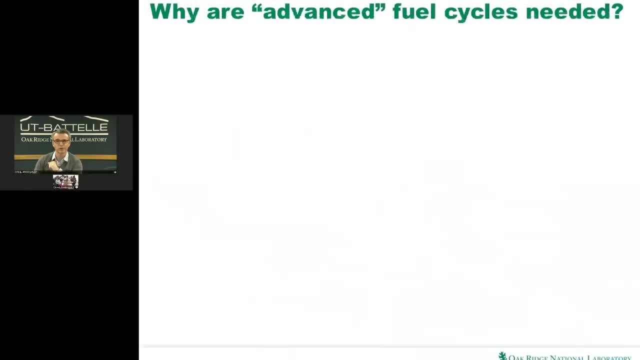 products are then disposed of directly, So that's where it's modified. So some of the drivers that are being considered right now are things like: we need better utilization of limited resource, despite what people say that there are only finite resources out there for uranium. 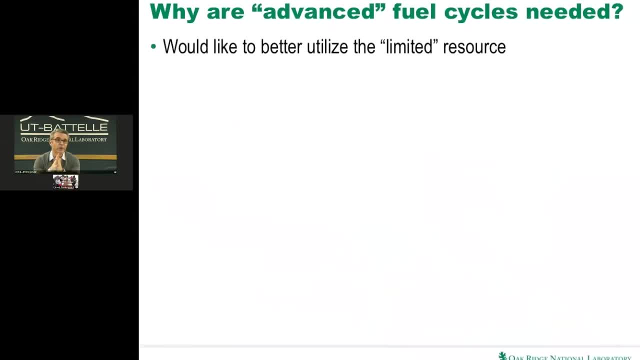 just like oil, gas and whatever. If you look at the OECD and the IAEA, they quote something like 60,, 80, maybe up to 100 years of known uranium resource. that's available today, based on a certain growth scenario for nuclear over the next few decades. But the important thing, 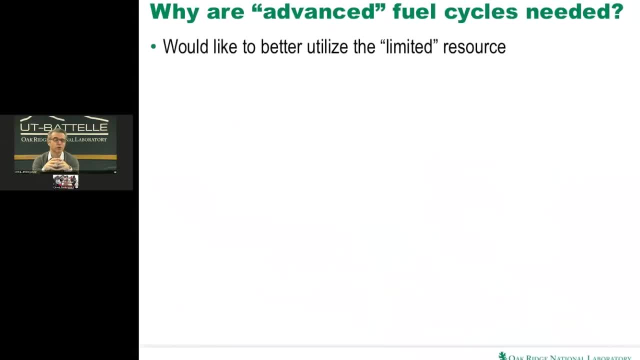 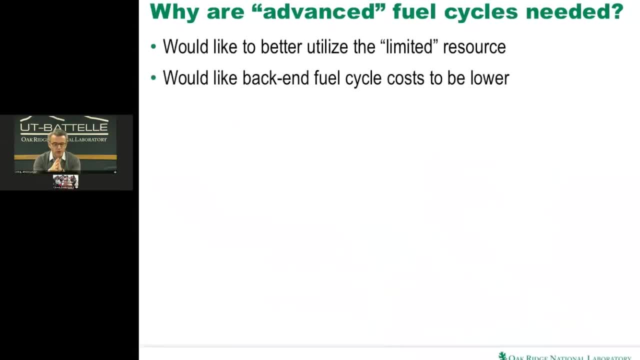 And you've got to take advantage of the commodity, The second driver for these advanced fuel cycles. we want the back end fuel costs to be lower, Things like the waste and so much that I'll touch on shortly- and impact that may have on repositories and the cost that drives. 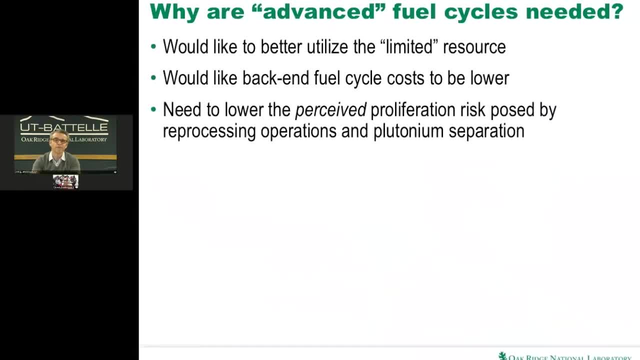 your repository. there's a plenty of good reason why you want to recycle. There is a lot of perceived proliferation risk posed by reprocessing and plutonium separation. I say perceived because the risk really is there for sure, but it's not a greater. 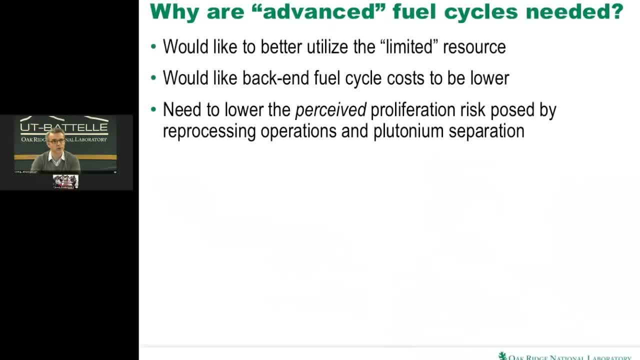 the perception that you have of the risk is greater and the perception that you have of the is almost that that's a greater risk than other fuel cycles. and again, i'm not going to go into it in detail now, but if you google or look up work by a guy called charles bathke, then you will see. 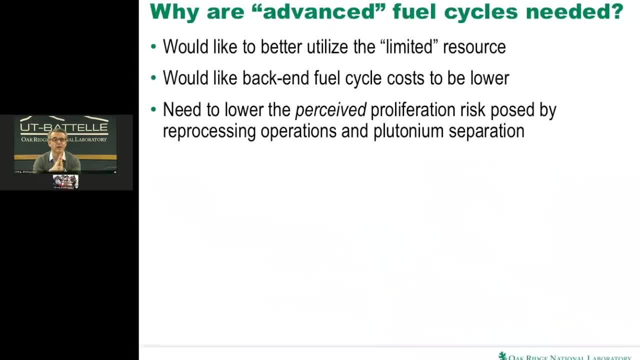 things like material attractiveness, figure of merit, where, basically, their analysis by people like los alamos and the other weapons labs illustrate that all fuel cycles, all of them, generate material that is potentially bomb grade material, weapons grade material. what that simply means is, therefore, every fuel cycle needs safeguards and security, so that's not to say 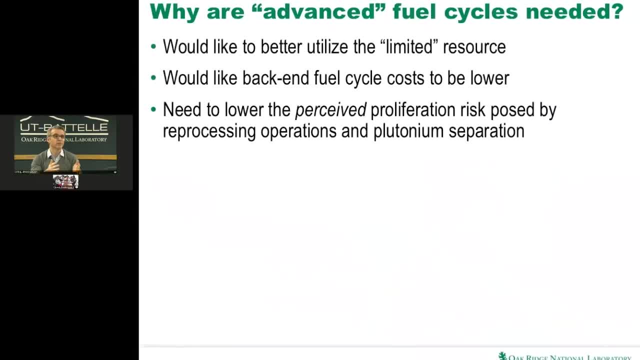 plutonium is any worse than anything else. for example, in the uranium fuel cycles of today around the world, where plutonium is not separated, we still have to have safeguards and security. so just to illustrate, there is not a great game changer there. we're also trying to simplify. 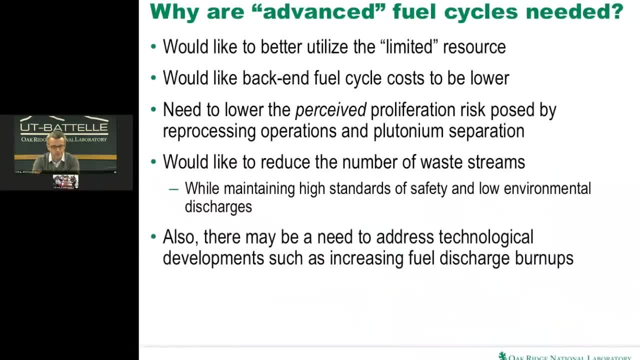 the number of waste streams and reduce the impact on the environment, and also, in the meantime, trying to maximize the benefit and the improvements we have in the existing fuel of today. one point to bear in mind, though, is that, for these ultimate, long-term future fast reactor fuel cycles, and all these, as i mentioned, these- 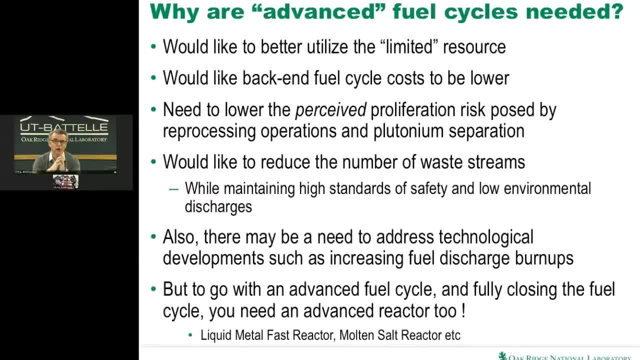 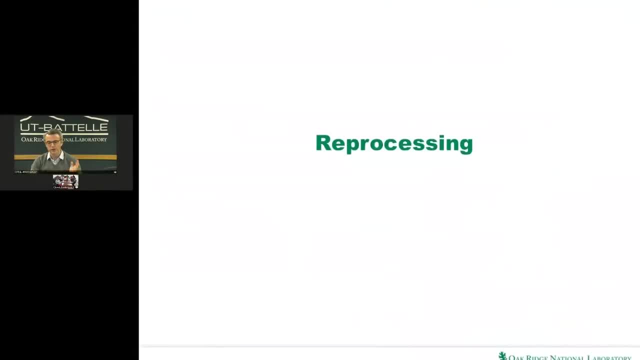 completely closed fuel cycles. you do rely on not just a fuel cycle technology but new reactor technology. so there's an awful lot of research, development and commercial case to be made. so things like developing future fast reactors or molten salt reactors are part of that. okay, so 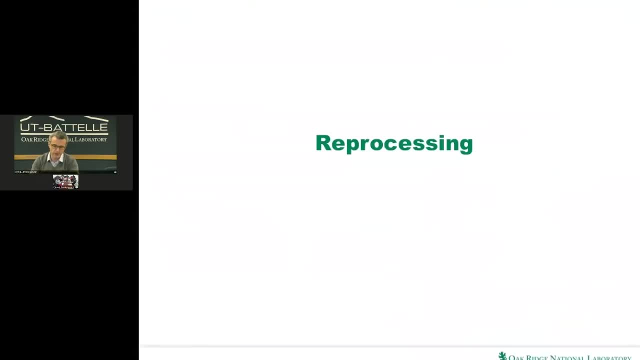 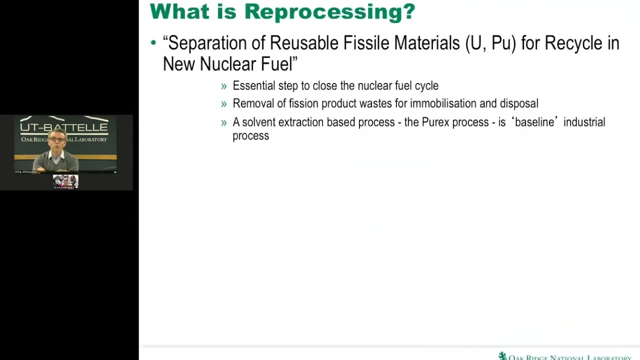 that's just trying to set you some of the scenes from the language, and i'm going to go now into the more detail and to talk about each of the components of reprocessing and recycle. what is research? what is reprocessing? first of all, well, reprocessing is the separation of the reusable. 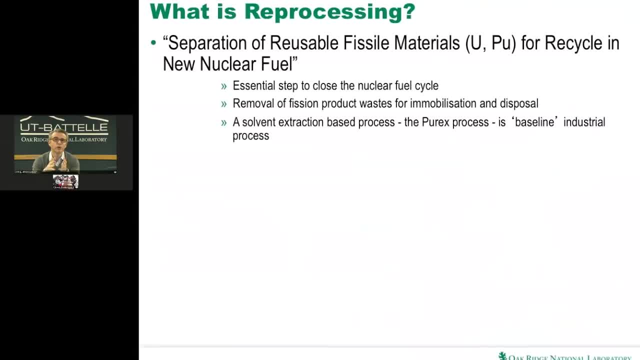 fissile material, typically the uranium plutonium, and the reuse of that, the recycle of that in new nuclear fuel. in many ways this reprocessing and recycling nuclear is no different to the way we hopefully all at home, recycle our garbage and extract the good stuff, the plastics, the bottles- from the traditional household waste. 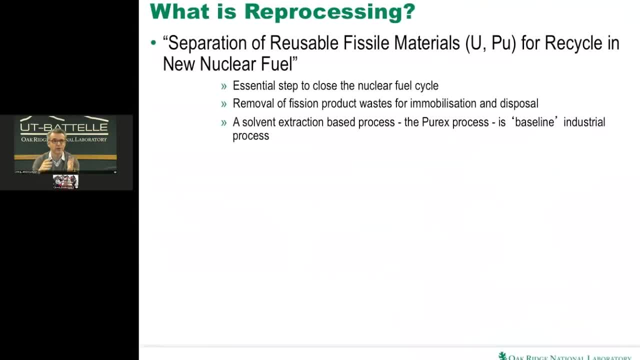 This is very similar. It's just taking the good stuff out, separating the good from the bad and recycling the good stuff. So this is what's essential: to close the nuclear fuel cycle. You have to have reprocessing, Of course, if you fission fuel, uranium or plutonium in a reactor. 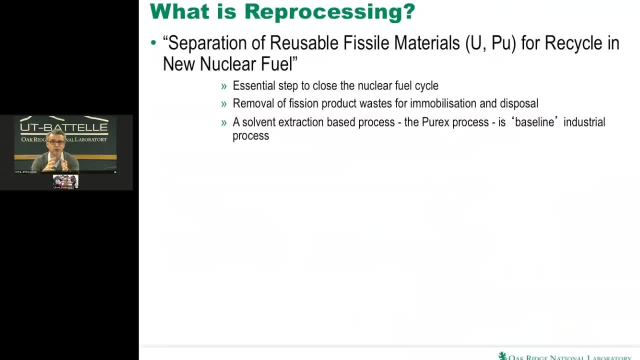 that fission process generates fission products and we want to get those out of the fuel. We don't need those anymore. They're definitely a waste product. We get those out, We immobilize and dispose of that And all of that. that separation process is all based on solvent extraction. 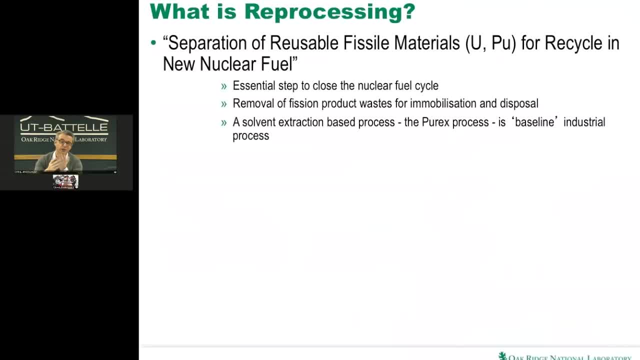 a chemical process known as PUREX, which basically stands for plutonium and uranium extraction, And that's the baseline industrial process of today that's used in the UK, in France and many other places. There are other options other than PUREX. 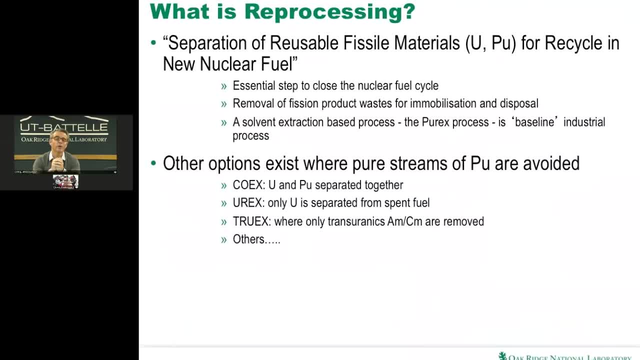 and again I'll touch on those later. but things like COEX means the co-extraction. So where there are concerns that maybe plutonium plutonium could be diverted for a weapons program or some other mission, then future fuel cycle options are looking at co-extraction of uranium and plutonium together. 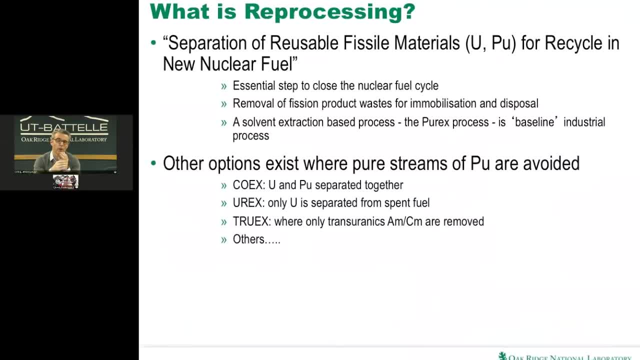 so that you don't generate pure plutonium, And also looking at things like where the plutonium is kept with the minor actinides and the fission products under a UREX, and there's a whole range of other things, And again I'll show you some of those later. 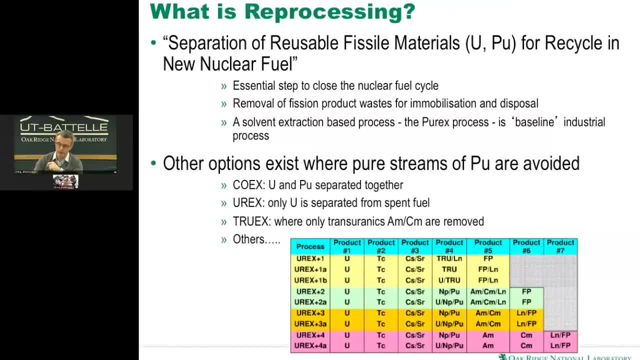 And this is just to demonstrate the complexity of the various product streams. I'm not going to go into that, but you can read that at your leisure later, just to show you the different options. And there's all the subtleties of UREX, plus one and all the various other things. 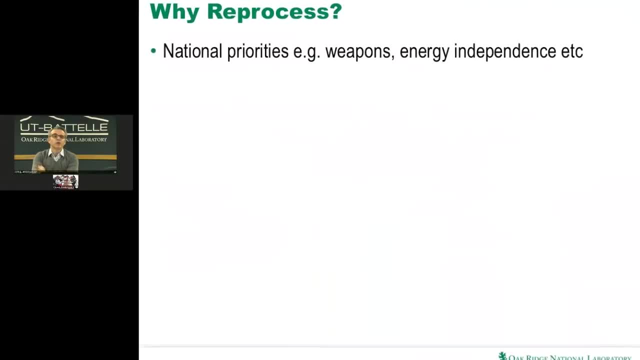 Again I'm not going to go into. So why bother? reprocessing is often a question we hear, because not every country does it. and why would they? Well, the first thing is, historically it's typically been because of the weapons program. 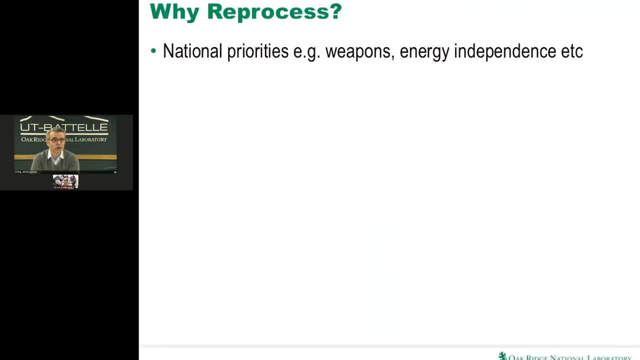 If you look at the US, the US has reprocessed historically, primarily because of to extract the plutonium for the weapons program. The UK also did exactly the same thing: was all about reprocessing to get the plutonium out of the fuel. 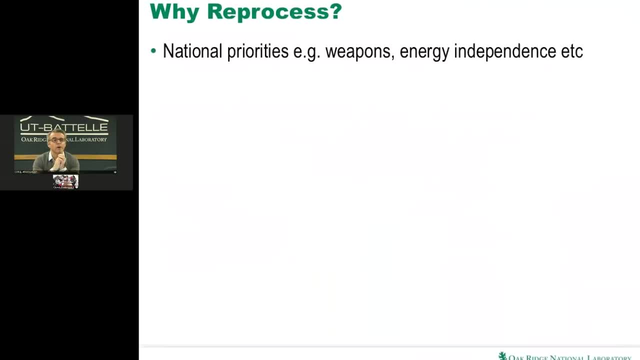 for the weapons program. So that's part of it. But on back to where I started the talk with regard to, and that's kind of, energy policy and energy supply, One of the things that, for example, Japan faces is that Japan has no indigenous oil or gas or coal. 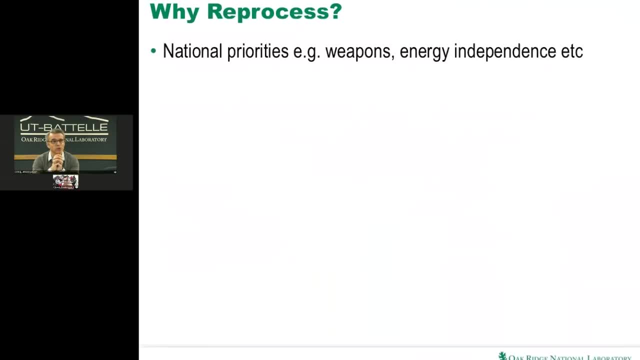 So it has to do something to to ensure energy independence, And that's why Japan is focusing very much on reprocessing and recycle. When they buy their uranium, they want to maximize the use of that uranium, and things like reprocessing enables them to do that. 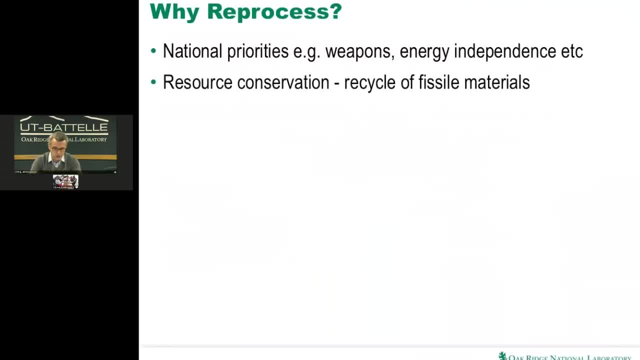 maximize their resource. I've touched on this one already: resource conservation and recycling for some materials. Reprocessing, in fact, does have some proliferation resistance benefits, with regard to either the burning of the actinides in one sense, but also if you have separated plutonium for all sorts of reasons. 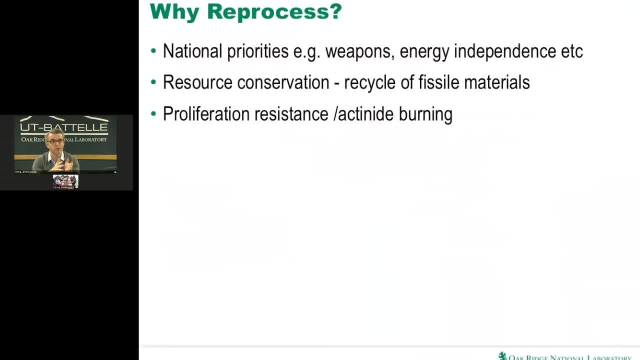 then you can reprocess and recycle that to destroy that plutonium too. So that's another way of looking at it. You actually are destroying the plutonium. Something I'll touch on and show you a couple of graphs shortly to more detail, is you can use reprocessing to minimize the volume of waste, volume of material. 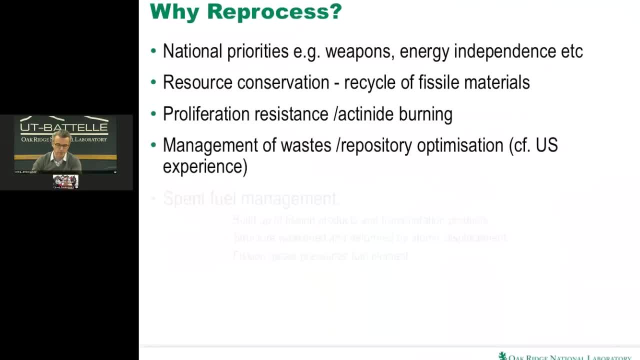 that you're going to put down the repository for ultimate disposal And then, similarly, spent fuel management. you end up with in spent fuel, you end up with a lot of fission products and potentially the weakness of the spent fuel. So, potentially by reprocessing, 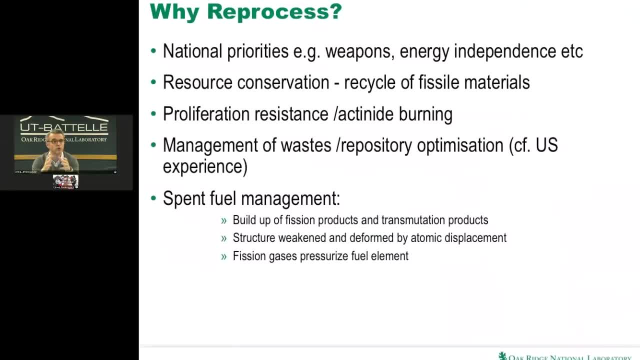 you remove that, those fission products, you remove that weaker structure, the fuel pins and fuel pellets, and you then kind of recondition in a sense into a repository condition And then, with somebody like the UK, one of the reactor options they have was the Magnox reactors. 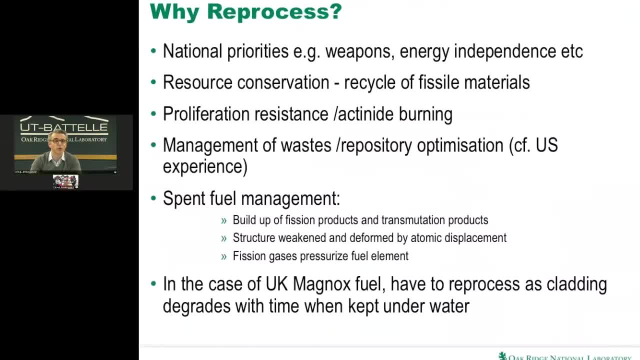 the old graphite reactors and in fact they have to reprocess that material because the cladding that surrounds the fuel is actually a magnesium alloy And it has to be kept under water because magnesium would be probably all done in high school class. try to light magnesium ribbon: it burns tremendously. 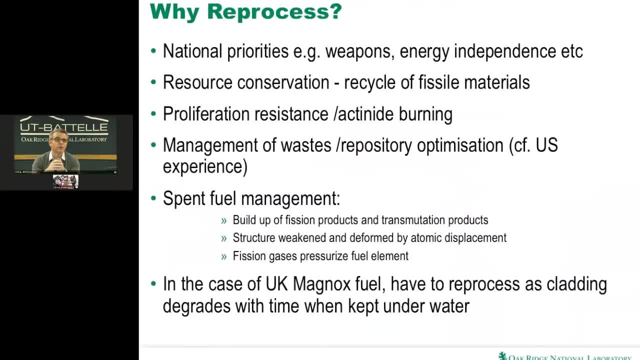 That's not exactly a reaction you want to see in a nuclear fuel. So what that means? you cannot allow it to be exposed to air, So you have to keep it under water. Unfortunately, when you put magnesium alloy under water, it dissolves in water. 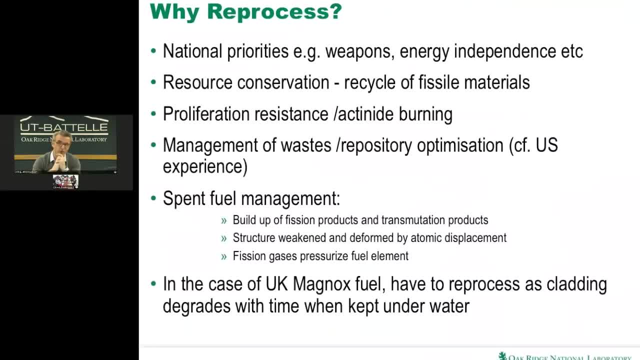 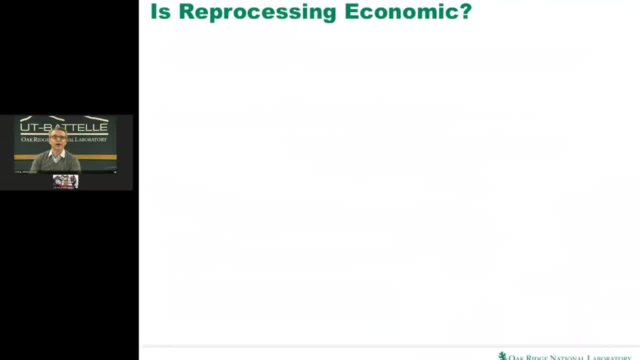 So therefore, that's also not a good condition. you want your fuel to be dissolving in water, So that's why they have to reprocess to put it in a much more stable form. So there's some of the drivers outside of economics, so the obvious ones to answer. 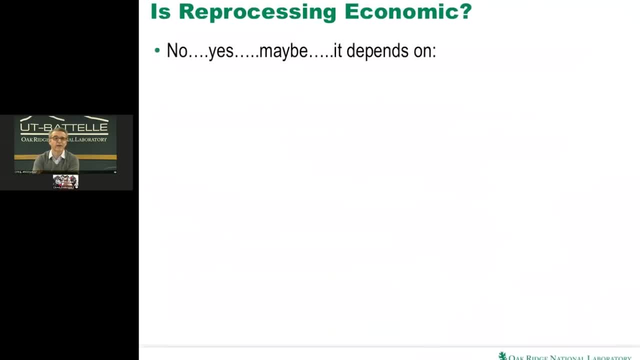 then, well, is reprocessing economic? And the answer is no? Well, yes, but the answer is: maybe It depends on so many different things. It's not easy to say for sure, And that's why some countries have gone down that route and others have not, as well as the drivers, based on country policy. 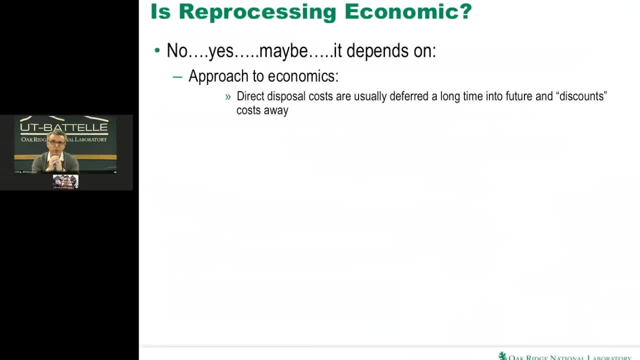 So it depends on a whole range of things. Often the approach to economics is one of the drivers. The problem with a lot of economics- for anybody who's done any- is particularly for nuclear economics. you get this thing called discounted cash flow analysis, And what that really means is that anything out in the long time. 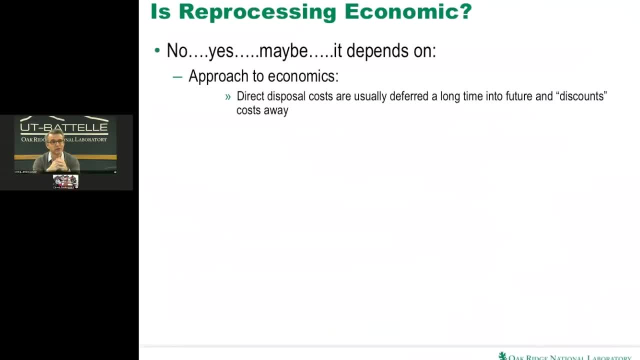 in the future, the value of that money is discounted away. So what happens is if you have an outlay in the future of, say, $500 million for a decommissioning project or a repository is needed, what happens is if you put a small amount of money aside today, 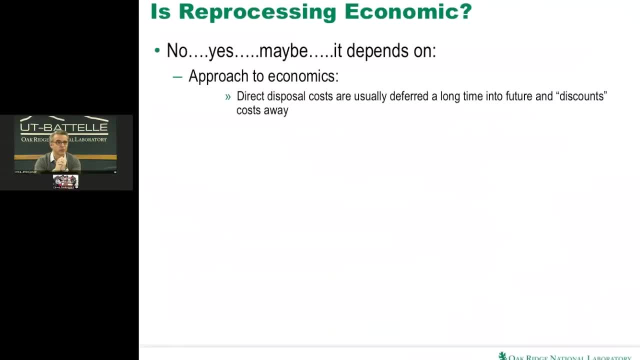 that money will grow by putting it into the banks or investing it and so on, And so you don't need to put your $500 million in the bank today. You just put a small amount of money and watch it grow over the next 50 to 100 years. 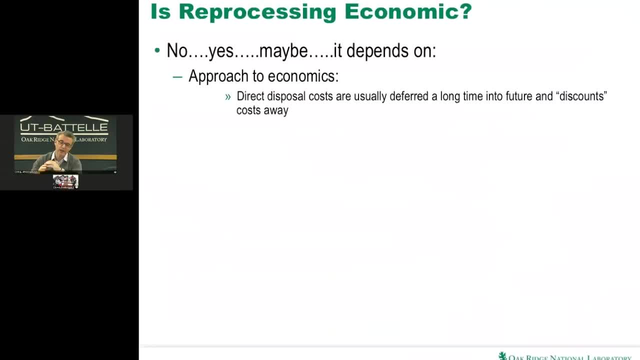 That same approach is applied here. Well, what happens is that all the direct disposal costs are put off so long in the future that it discounts all the actual costs away. The costs kind of disappear. The other thing that drives the economics of reprocessing is a yes or no is the price of uranium ore. 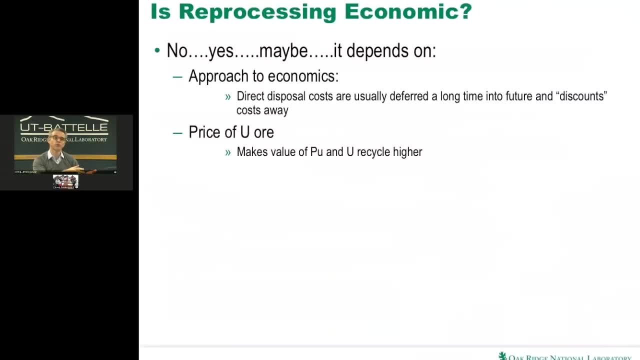 If the price of uranium is very low, which usually coincides when there's lots of uranium around- then if the price is low, then why recycle? We don't need to be so concerned with the availability of that resource. but if the price of uranium goes up, then suddenly the value of that reprocessed uranium and the value of plutonium also goes up to recycle. The other thing as well is that you can achieve higher burnups in light water reactors. What you tend to find is that if you need to get more energy out of your fuel, you need to put more fissile material in there. 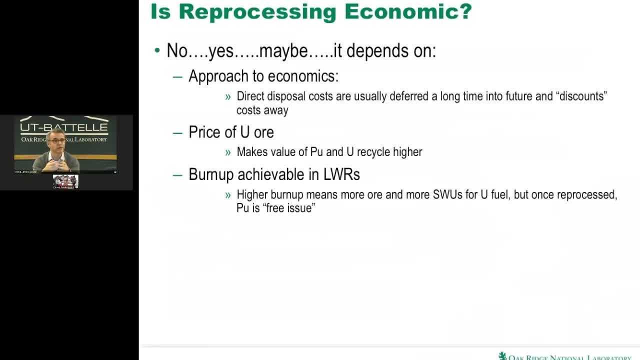 In the case of uranium, you have to pay for that by enriching it. The more you enrich, the higher the cost and that goes up exponentially. Whereas with plutonium, if you've already made the decision to separate that plutonium out, plutonium is free issue at that point. because it doesn't matter, when you manufacture a fuel with plutonium fuels, whether I put 1% plutonium into that fuel or 10% plutonium into that fuel. it actually doesn't increase the cost of that fuel production at that time. 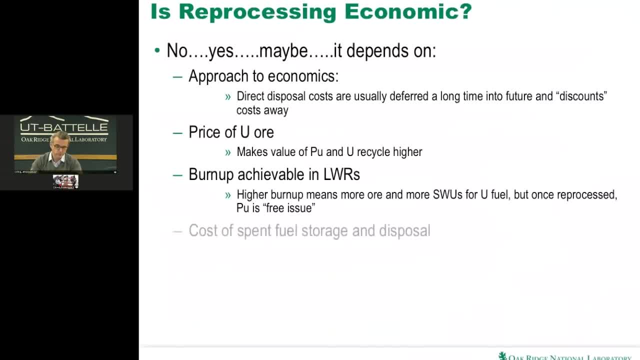 So what it means is I can get more energy out by doing that Cost of spent fuel. that obviously drives things also, But in general the cost of the two- keeping irradiated fuel in the repository or the cost of reprocessing- they're comparable. 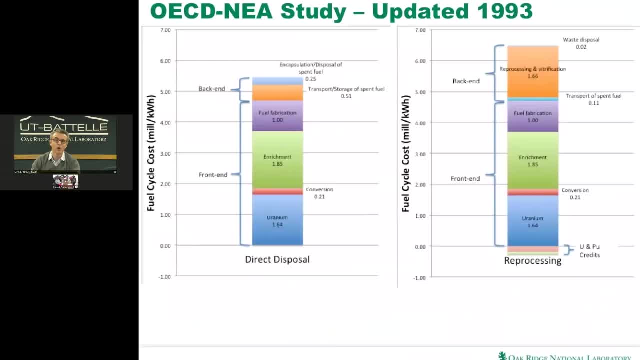 And this is something again. I'm not going to the details here, but this is some studies from the OECD and I just updated some figures from 1993.. But this just shows and compares the direct disposal on the left with reprocessing on the right. 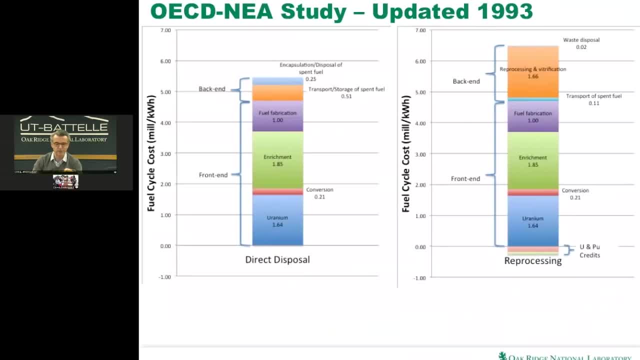 Of course, all the front end of the fuel cycle components are exactly the same. It's only the pieces at the back end, at the top of that histogram, that changes. What you find is that the front end costs dominate. about 80% of the overall fuel cycle cost comes from fuel costs. 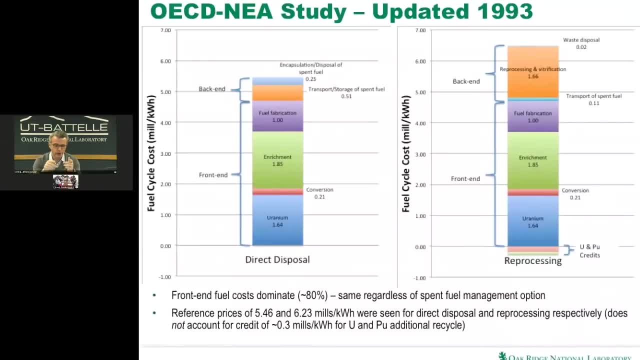 Regardless of which option you choose, And if you look at these two examples, we've got a comparison of about five and a half mils per kilowatt hour versus six, As you can see on the left and the right What the chart on the right takes. no. 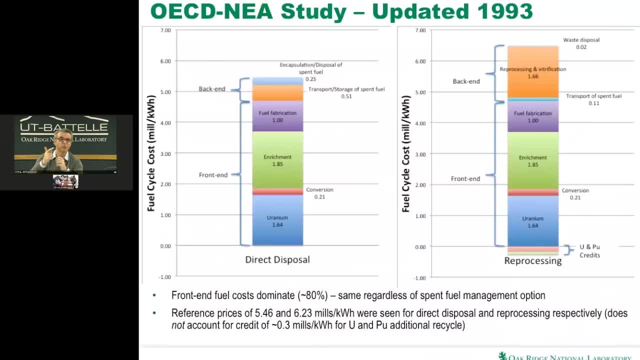 account of, though, is that the material that comes from reprocessing the uranium and plutonium. we can recycle and reuse that, and therefore that's an avoided cost of us having to buy more uranium. That's not in that chart And that equates to about 0.3.. 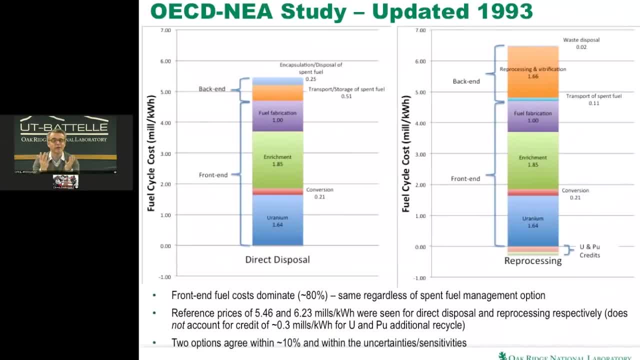 So when you look at the value overall they're pretty comparable within about 10% of each other. And of course the things on the left can go up or down, Things the right can go up and down. So within uncertainties they're pretty much equivalent. 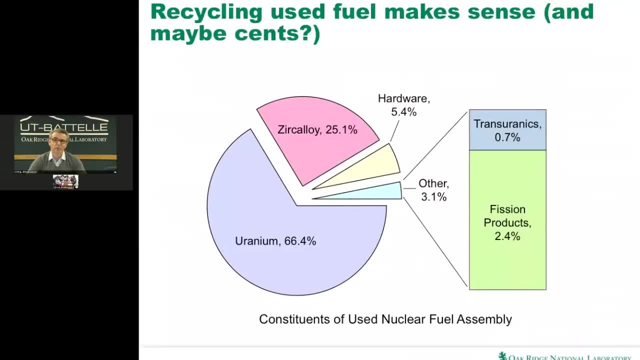 So, when we talk about reprocessing and recycle, which bits are we talking about recycling and which bits are we talking about throwing away? Well, in fact, more often than not, what's typically been talked about is just reprocessing and recycling the fuel pellets themselves. 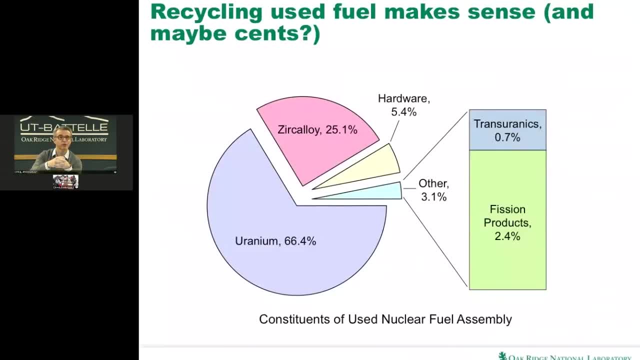 The actual fissile material and the pieces that are inside the mechanical hardware of fuel. But in fact here at Oak Ridge, working on the US Department of Energy program, one of the things that's also being looked at is in fact recycling the zircaloy, the actual cladding that's in the fuel and the hardware, and actually 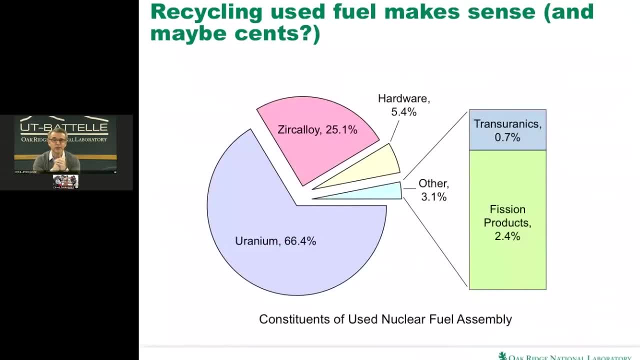 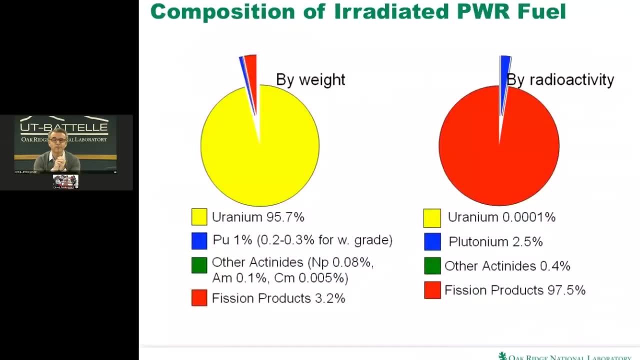 recycling the metal as well as the fuel inside those metal components. So that's something else to bear in mind. It's not just necessarily recycling and reprocessing from a material of the fuel. But to me this is probably one of the key takeaways from the message about the value or purpose of reprocessing versus. 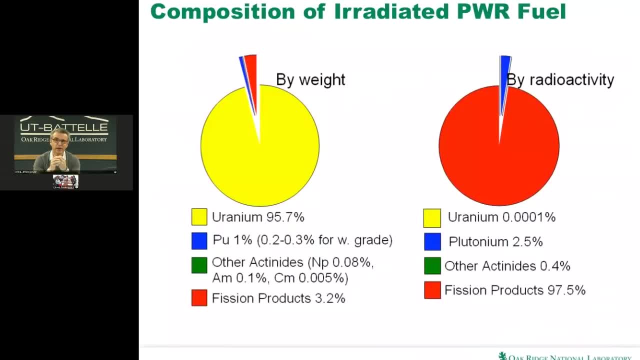 direct disposal. just forgetting the chart on the right hand side, For now just construct the one on the left by weight pie chart. When we load fuel into a reactor, of course it's 100 percent uranium, But when we discharge it after it's four. 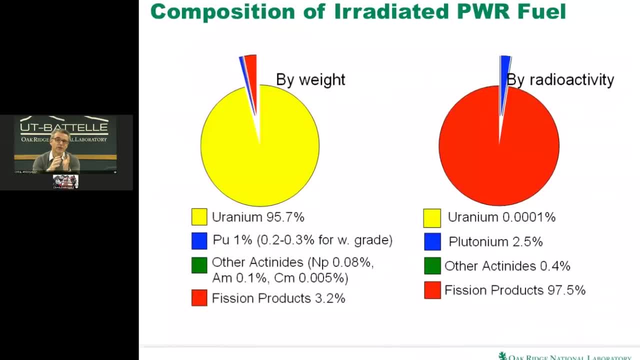 five, six years in a reactor, after it's been cooled, and so on. what we see on the left hand side is then what the weight fractions are of those various isotopes of various elements. So uranium still makes up the vast majority. Typically, 96 percent of the 100 percent is still uranium. 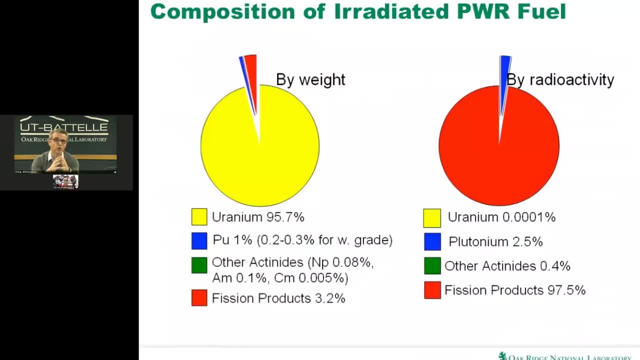 Then we've generated about 1 percent plutonium in that fuel. We've produced other actinides like curiums and so on. But of course what we've done is we fission that uranium And so we've got fission products, which makes about 3 percent. 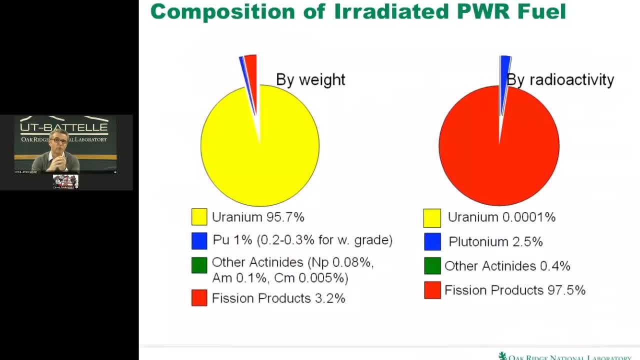 The chart on the right hand side then shows you not what their composition by weight now is, but what the composition by radioactivity is. Now, why is that important? Well, it's radioactivity. You can consider either as the the dose to an operator, or the dose to the public, or the dose to the repository. 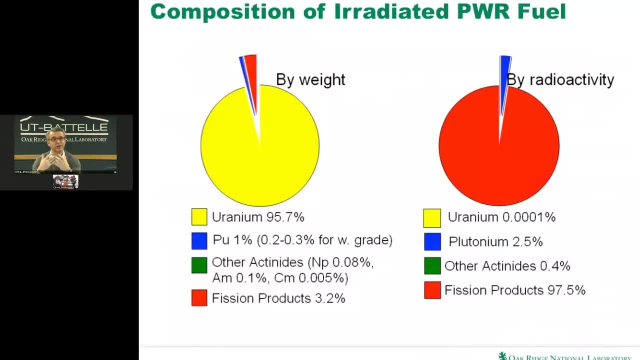 Or, alternatively, you can look at that as meaning the decay heat, the amount of heat that that spent fuel is generating. What you find is that the vast majority of that material in that spent fuel is actually producing hardly any of the decay heat or radiation in that fuel. 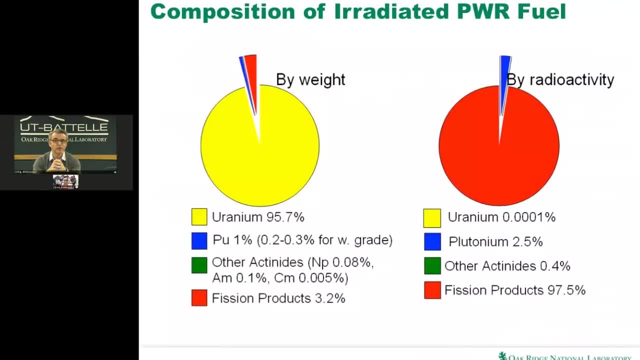 It's in fact the majority- comes from the fission products. So if you can therefore separate out those fission products, ie the very small volume, and concentrate that down now you've got a much, much smaller volume to put in your repository. 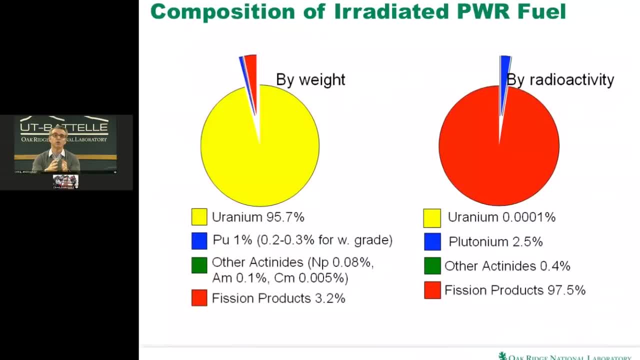 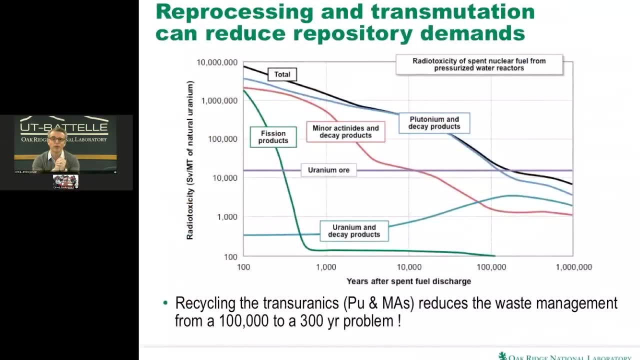 And therefore the demand on the repository is much less, Whereas if you were just to put the whole fuel assembly down there, you're actually filling a lot of volume for very little benefit, And so this is slightly more complex chart. but if you bear with me, 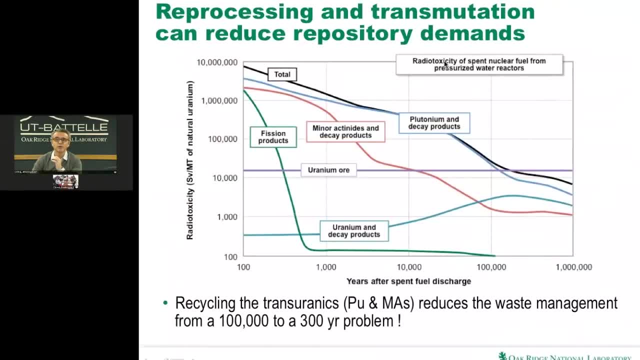 you'll see where this becomes important is if you look at the. hopefully you can see the arrow on here, but basically if you look at the total radioactivity. So what we're doing is we're plotting radioactivity on the X axis, Y axis, sorry, versus time on the X axis. 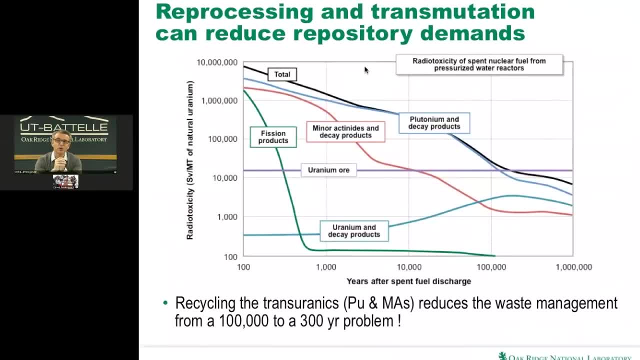 What you see is that, over time, it's actually the plutonium and the decay products that are kind of the long lived things that stay around for a long while, And therefore they're the ones that can have a long term impact on your repository. 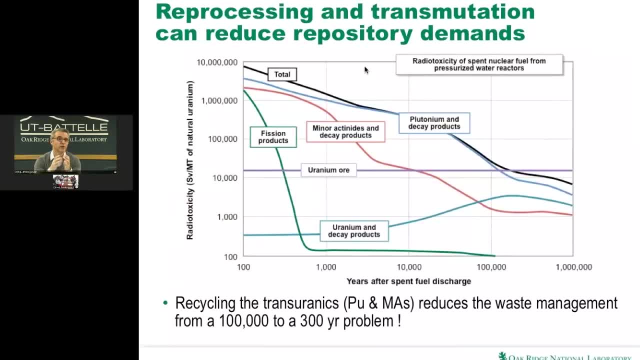 So if you can remove those from your fuel and therefore they're not going in the repository, and you can remove the minor actinides and decay products and do other things with that, what you end up with is, instead of being a 10 to 100,000 year problem you actually can now reduce this way. 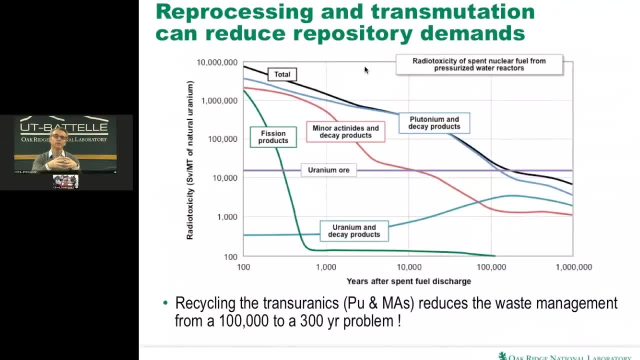 way over to the left hand side, where all you're actually doing by putting concentrate on your fission products is you actually now got a 300 year problem because after about 300 years you're now back to that uranium ore level, where you're back to that kind of background level of uranium ore. 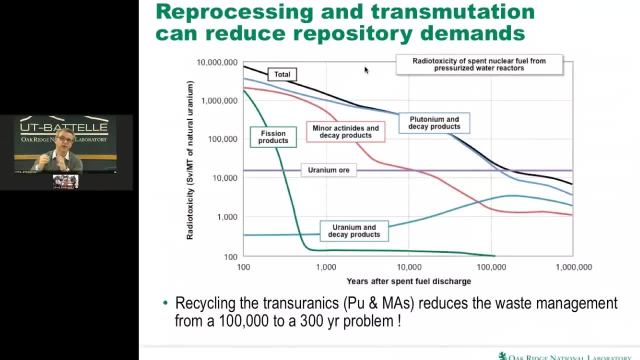 radioactivity, whereas if you didn't do that, it takes you 100,000 years or more before you get to those background levels. So that's what that graph just shows. It's kind of showing what I said earlier in a slightly different way. 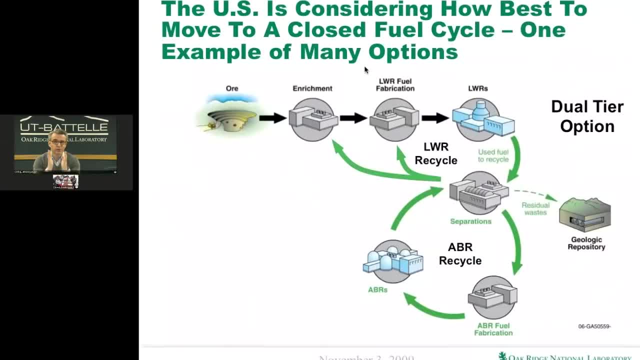 So the US is considering how to move to one of these advanced fuel cycles. today, One of the programs of work that's been taking part within the US Department of Energy is something called the Fuel Cycle Options Campaign. So we're looking at a whole range of fuel cycle options. 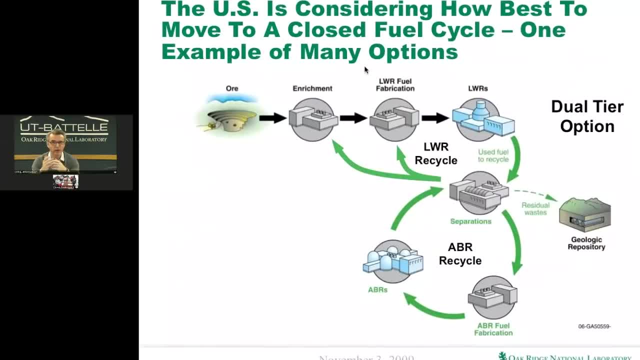 whether that's with fast reactors or thermal reactors, with thorium or with uranium and a whole range of other things. And again, you can find that, those reports and that those studies, on the web. But The key thing here for the US is those options are being considered. 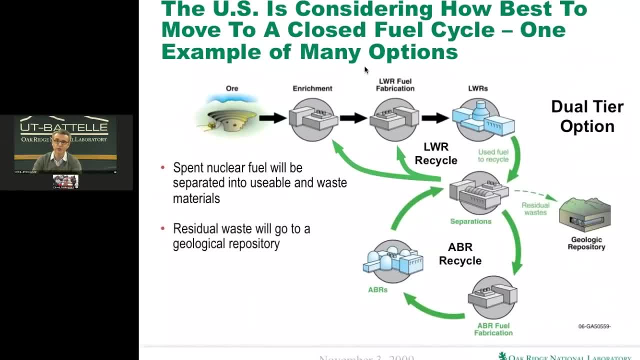 The once through fuel cycle is still the, the fuel cycle of choice. It produces, you know, 20 percent of electricity in the US. So at the moment there's no point to move away from that. Again, I'm not going to go into any detail, but just want to let you know. 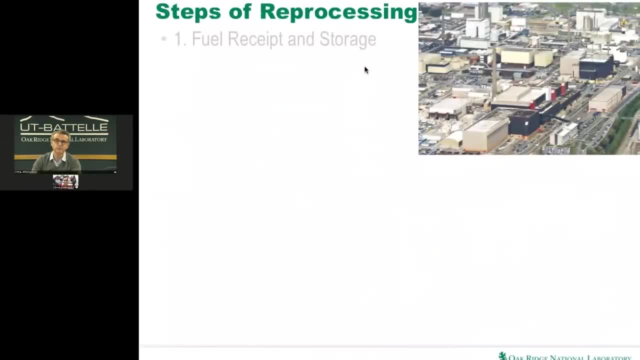 there are other options out there that the US are considering today. So just to demonstrate some of the steps in reprocessing- and again I show you some pictures and some diagrams to bring some of this home, I hope The first thing is- and what you're seeing on the right hand side is a picture- 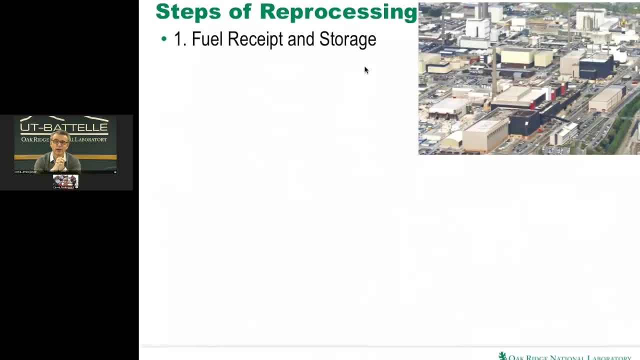 of the Sellafield reprocessing plant in the north of the UK. So you're seeing the building right in the centre there with the kind of red chimneys- the red side actually sides of buildings and not chimneys. That's the side of the building. 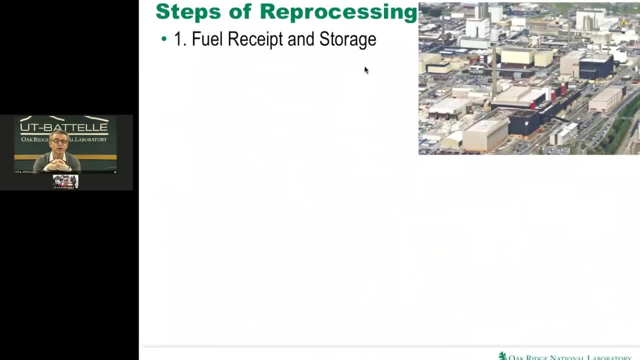 That's the thermal oxide reprocessing plant known as Thorpe. That's in Sellafield in the UK. So at the bottom of that picture you see a kind of a square building. That's where the fuel is received and stored. OK, so that's. the first step is receipt and storage. 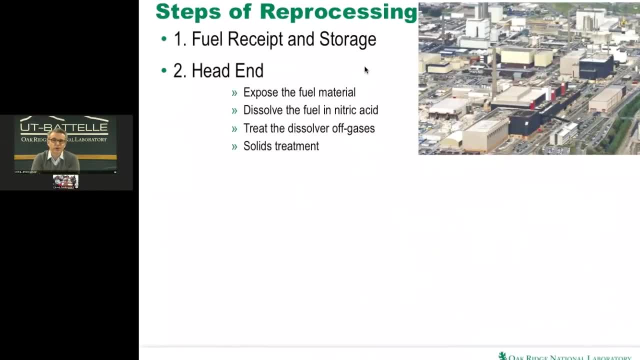 The second stage after that is what's called the head end process, And I'll show you some pictures and some schematics in a second. So the the the first step, after it's been received, the material has been received and stored, is then to expose the fuel itself, the pellets themselves. 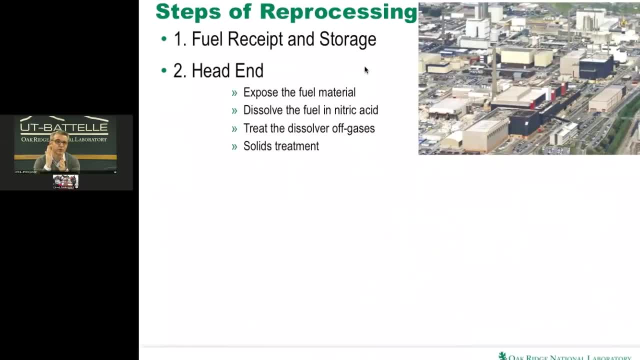 from with inside the cladding. So the first thing that has to happen is we have to expose that fuel by shearing it and basically shaking out, removing the fuel from the inside. We then dissolve those fuel pellets in nitric acid And of course by doing that we generate some off gas. 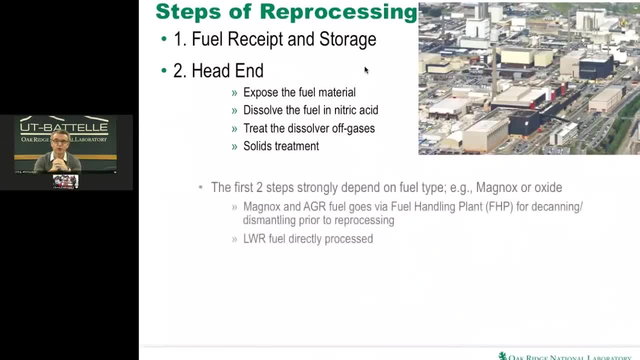 We have to treat the off gas and then we dissolve and treat the solids. The first two steps- that receipt and storage- and head end. the steps are usually the same. in terms of that they happen, but depending on the fuel type or reactor type there may be some additional steps. 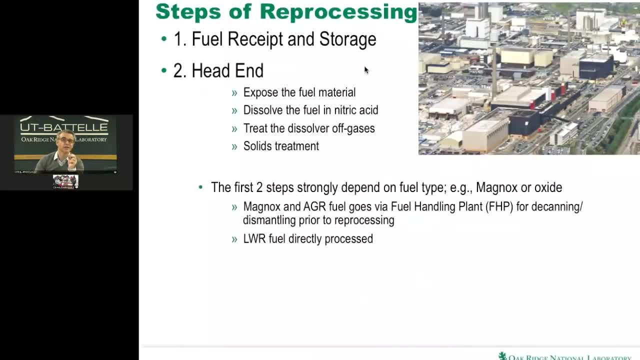 And again, I'm not going to go into that, but I just wanted to flag that. what you'll often see is, if you talk about reprocessing fast reactor fuel, the receipt and storage and head end processes will differ from what I'm about to describe now. 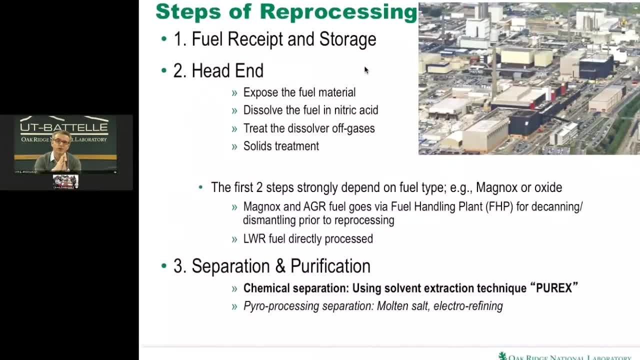 Similar processes still needed. The third stage- after you've received the fuel, you've dissolved, you've chopped it up- is you now need to chemically separate all those elements that I described and then, once you've separated them, they need to purify them, to put them in a form that can be reused if appropriate. 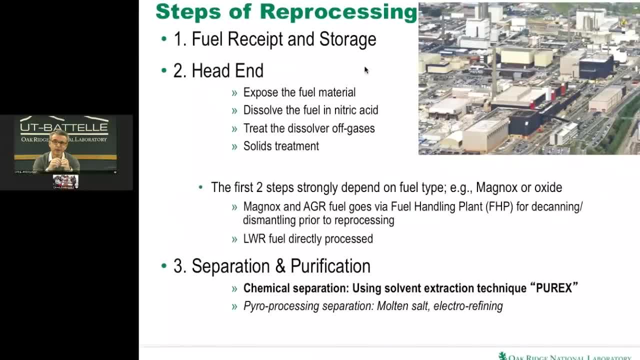 And typically that's done using the purex process, as I mentioned earlier, using solvent extraction and that's with chemical separation. But again, just a little marker here. There are alternatives for things like fast reactor fuels, which is known as pyro reprocessing, using something like a molten salt or electro refining. 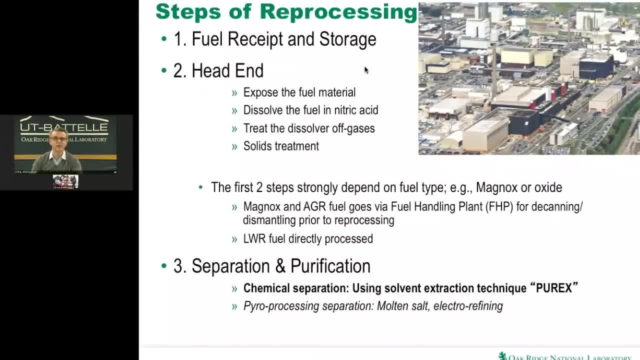 And again, I'm not going to go into that today, but just to be just to flag that there are alternatives. And then, once you've gone through all that, then you might, you'll need to store that material for potential future reuse and the material that you're no longer. 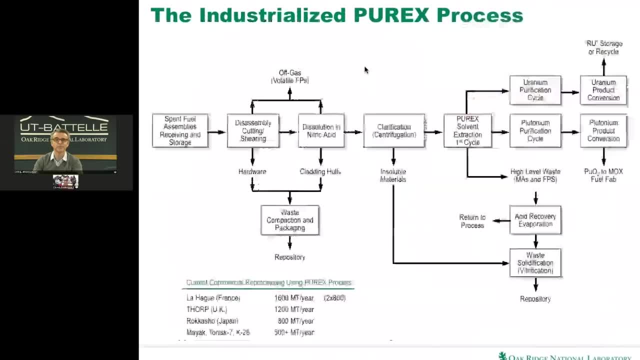 going to use. you then have to do something with waste treatment. So this is the flow sheet in a little bit more detail, starting from the left hand side, going through spent fuel assemblies received and then you cut and shear them and you see the off gas kind of goes upwards. 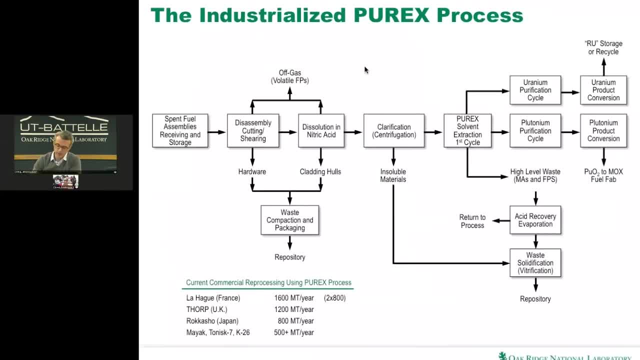 And so I'm not going to go into that in detail, just conscious of time, And I've got some other figures that kind of illustrate that a little bit more. But again, just towards the bottom of that chart you then see some of the other reprocessing commercial facilities around the world, in France. 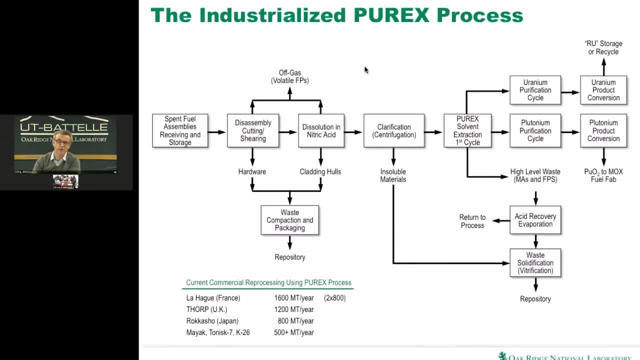 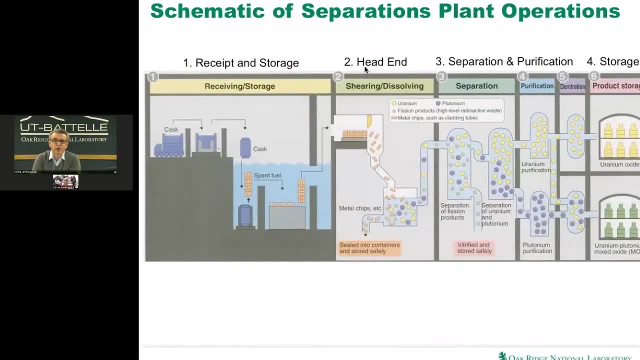 the UK of what you mentioned, Japan, which is going live kind of imminently almost, and then in Russia. So this is just again to show you kind of some schematics and I'll show you some things in a second of what this thing looks like. 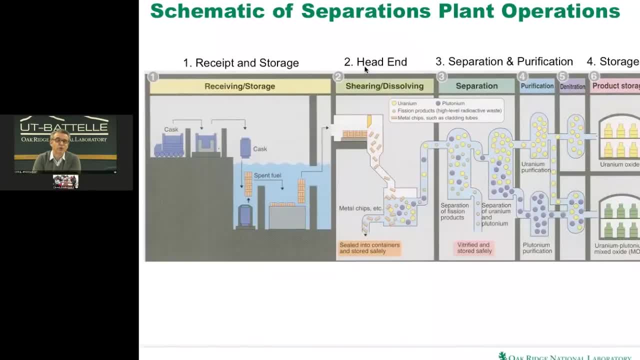 But again just stepping through receipt and storage just where the fuel is brought in from overseas or from elsewhere, from the reactors, brought into the reprocessing plant, the cask is then loaded into a spent fuel pool. The pool then provides that radiation barrier and the heat barrier. 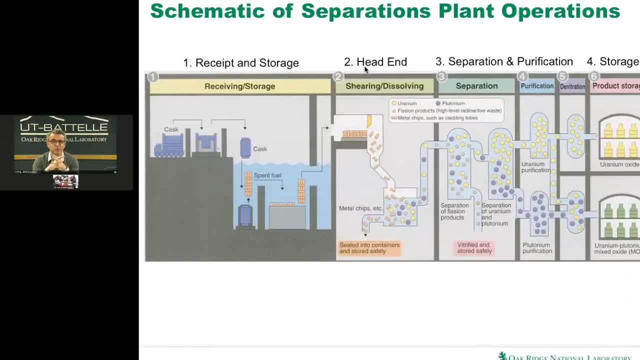 Then the fuel is removed and stored until it's ready for the reprocessing plant, And then that's then lifted up to where it can be sheared, chopped up, And I'm going to show you some photos of that shortly- Then the chemical separation takes. 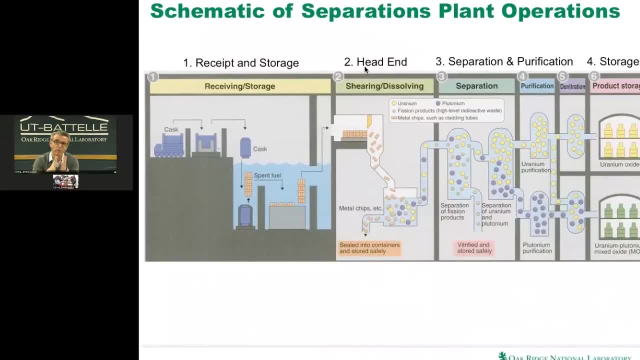 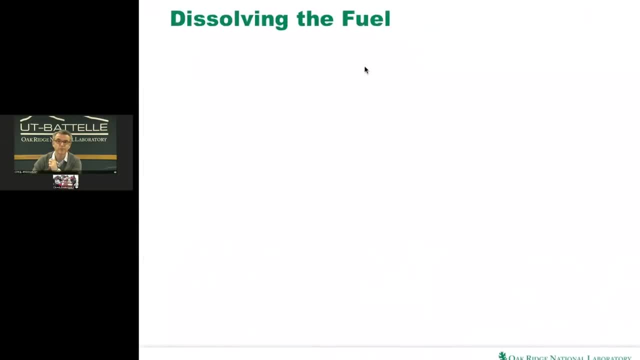 place in stage three, there, then purified, because the uranium goes one way, plutonium another. then it's purified and then stored if necessary, And then the waste products go a different direction. So, in terms of dissolving the fuel, as I said, once you've actually chopped, 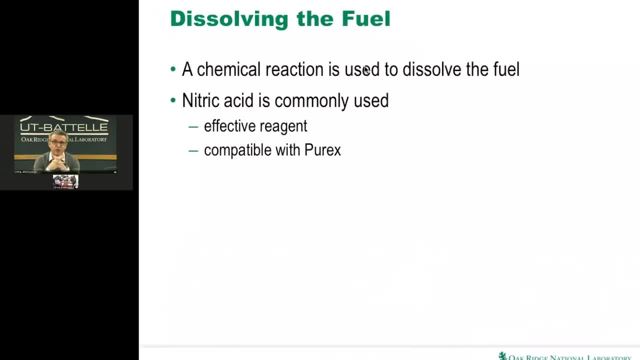 the fuel up and you've now exposed those pellets. it's a chemical reaction that's used to dissolve the fuel, and it's typically nitric acid, And when you look at some of the chemical processing that's involved in reprocessing, you realise just how. 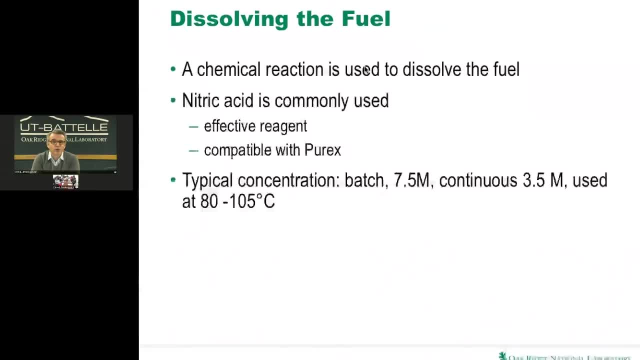 difficult this whole process actually is. You've got something like seven and a half mol and nitric acid used at typically up to 100 degrees centigrade in a very, very, very strong radiation field. So all of this is done behind tremendous shielding. 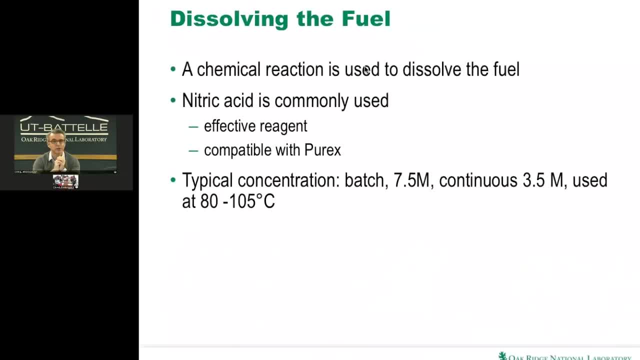 And so when you start thinking about the heat, the dose, the chemical interactions, there's an awful lot to take into account from a safety perspective. There's also a potential risk of that material being concentrated and going critical, So they actually do things like put. 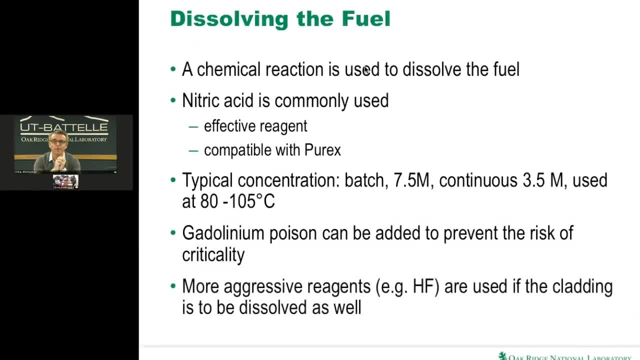 bad linear poisons in there to prevent the risk of criticality And in fact for other reprocessing options, for example like the thorium fuel cycle as well. there are other chemical reagents that may come into play, something as strong as hydrofluoric acid, which is particularly corrosive. 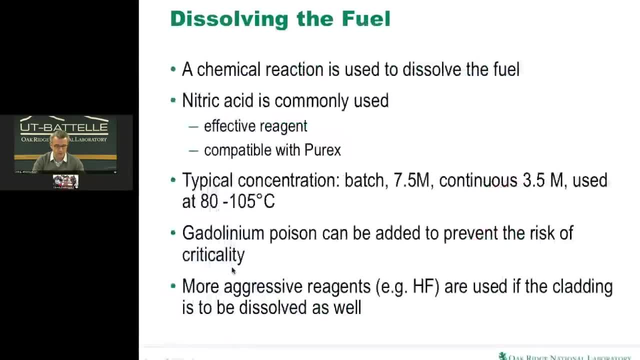 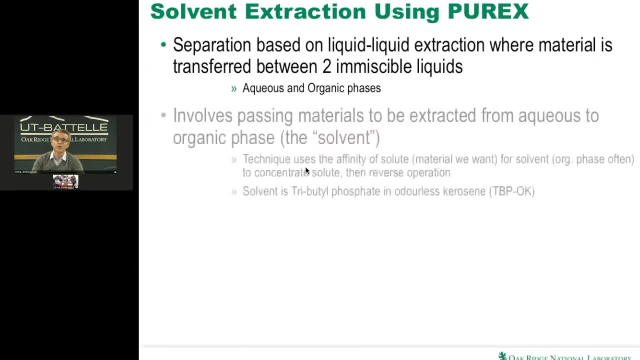 So again, oops, excuse me- You can particularly again see that some of the challenges that you can face in a reprocessing facility. So the way this actually works is again it's easy for me to show you in a diagram but how this whole chemical process works. 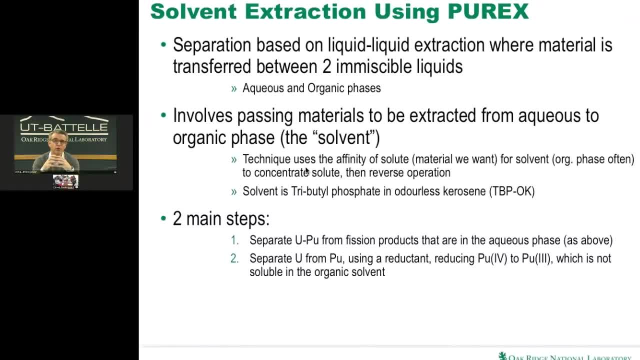 It's a liquid-liquid extraction process where you've got two phases and those two phases being immiscible. It's that then the material after kind of gets transferred across from one phase to the other phase towards the solute with the material that we want. 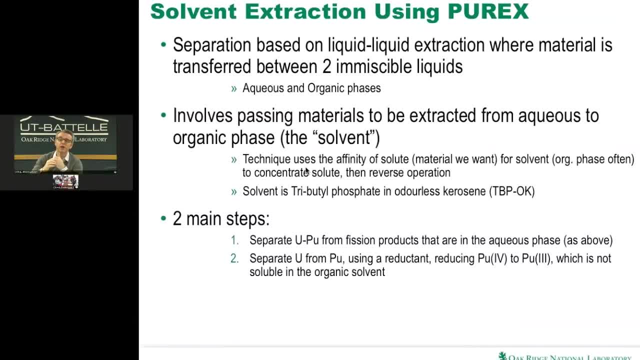 And again I show that in a picture in the schematic. It's much easier to see. But the first thing is that we we first of all separate the uranium and plutonium material from the fission products and the minor actinides. So they go one side, one way and you'll see that in a second. 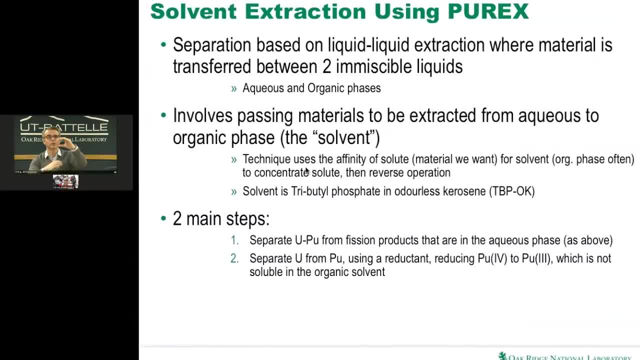 And then, once we've done that, we've got these two kind of bulk materials, We're then able to concentrate on the separation of the uranium and plutonium from each other in the next stage of the process. So again, the easiest way to see that is in this process here. 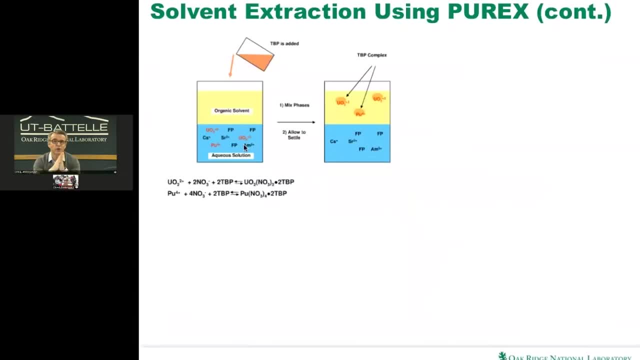 At the bottom we've got the aqueous solution, the nitric acid and the fission products and the uranium and the plutonium, the minor actinides, all mixed together And then you add to an organic solvent on top, something like tributylphosphate. 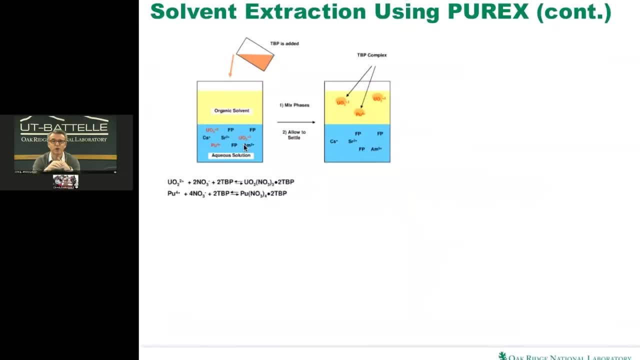 tributylphosphate and odalis kerosene are the two typical chemicals that are involved in this, And what you what then happens is, by then those two being mixed, you get this, this solvent extraction process, where the material that you want, the uranium and the plutonium- is drawn across into the upper phase, therefore leaving the fission. 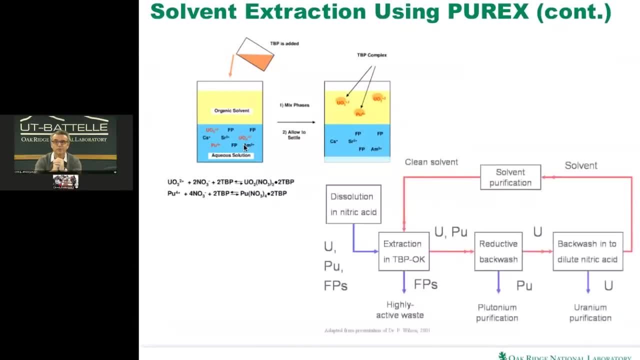 products and the other materials behind in the in the lower half. So that's what you see. And again here, just again to reiterate the extraction in TBP: OK, where the uranium plutonium goes one way, the fission products go another. 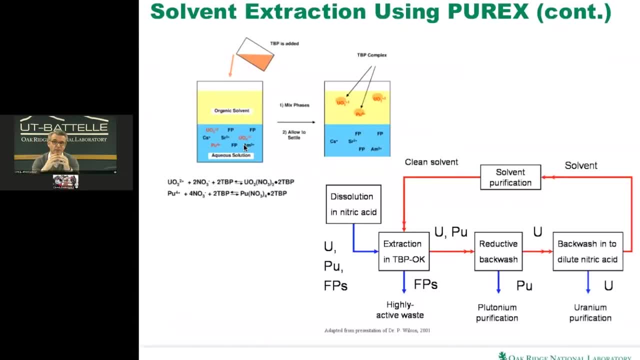 Then what you can then do is then change by changing the acidity of that, of that separation material. You can then have the uranium go one direction, The plutonium drops out of that, and then you can purify. And again, I'm not going to go into the details where you can just see, hopefully, 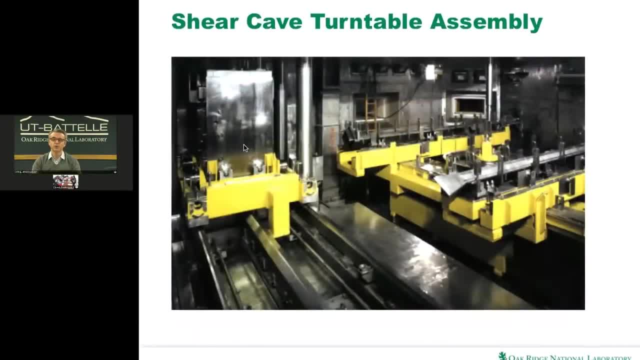 see the various stages. But this is. I just wanted to show you some of the pictures inside of one of the reprocessing plants, the Thorpe reprocessing plant in the UK. So this is what's known as the Shear Cave And hopefully you can see on the right hand side what appears to be a kind 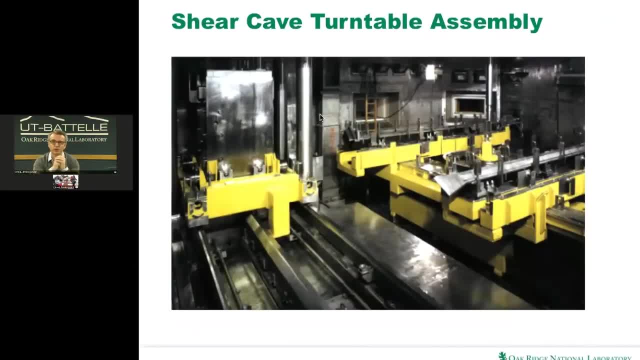 of a V shaped kind of guttering that goes off into the distance, But what happens is the fuel assembly is brought up from the spent fuel pools down below, brought up and then lowered into that V shaped, that V shaped gutter That holds the fuel assembly in place, for it to then turn to then face the shearing blade. 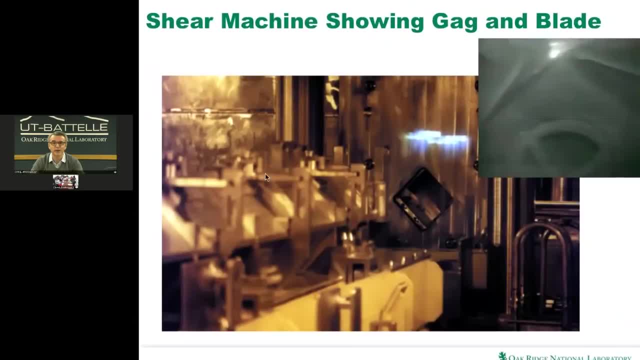 So what you then see here is the fuel assembly in that, now, in that gutter- that was just describing that holding position, and it's now being lined up ready to be faced and pushed through that, the hole on the other side where the shearing blade will come down and begin to chop the fuel. 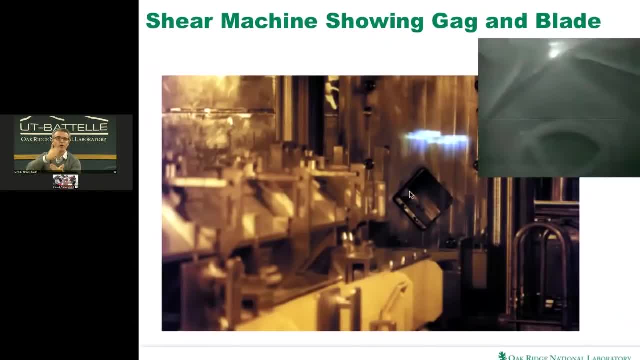 Now, what's interesting is usually when I always visualise chopping, I think of something quite kind of quick and harsh like that. but if you think this is, that in fact is more like a knife through butter. it's more like where it's a continuous pressure being applied. 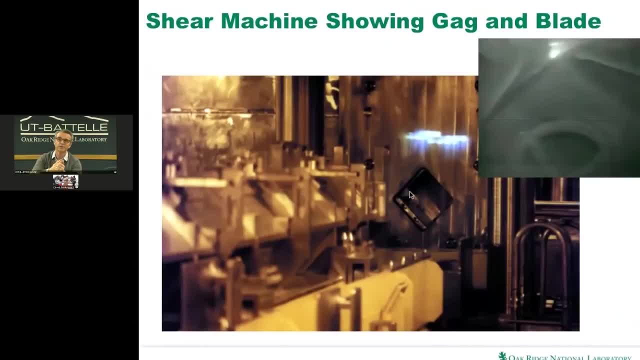 to slice through the fuel. it's not a big chopping mechanism And what you see just about, I hope, in the photograph on the right hand side- you hopefully can just about make out a fuel assembly here- And that's the blade coming down to begin to chop the fuel. 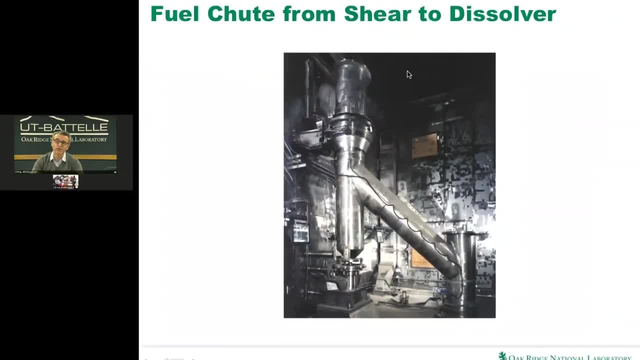 So, at the top of this shoot up, here is where that fuel is being chopped into, typically one to two inch pieces, and so that will then fall down from the above down into the collection basket at the bottom, and that's where the dissolver is waiting. 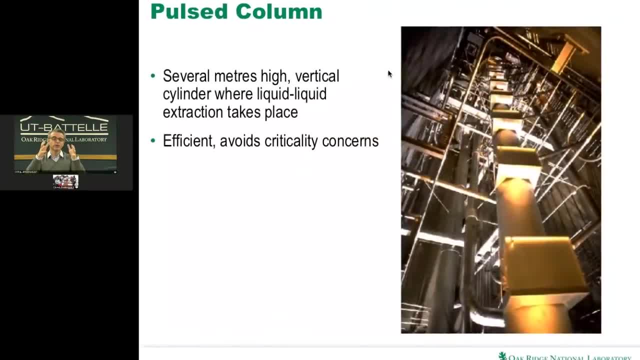 And the dissolver- just again just to illustrate- is almost like basically a stainless steel basket, of which that is immersed in nitric acid And so when that, when that's loaded into nitric acid, the material, the fuel is dissolved and comes away from. 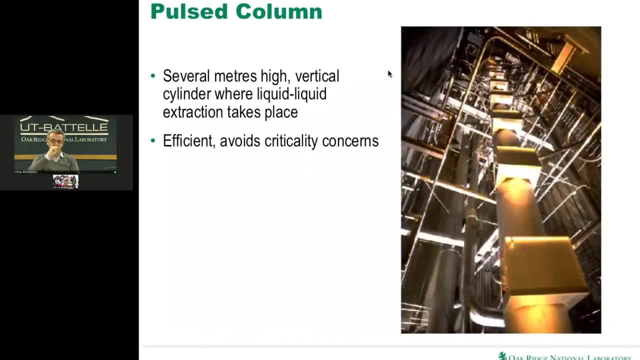 the cladding pieces, the elements, the holes, as they're called, excuse me. And then that's dissolved up And then when you lift out the basket, the holes, the cladding is left behind in the basket and in the liquor that's behind then is your uranium plutonium. 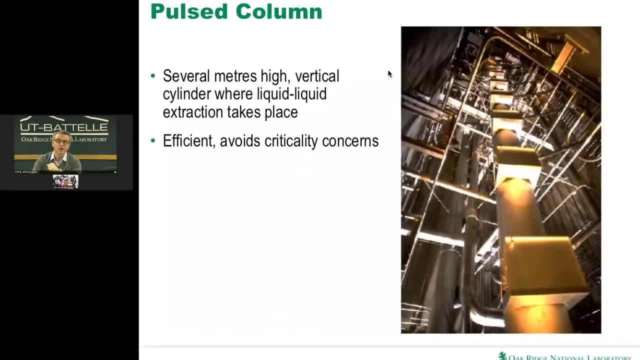 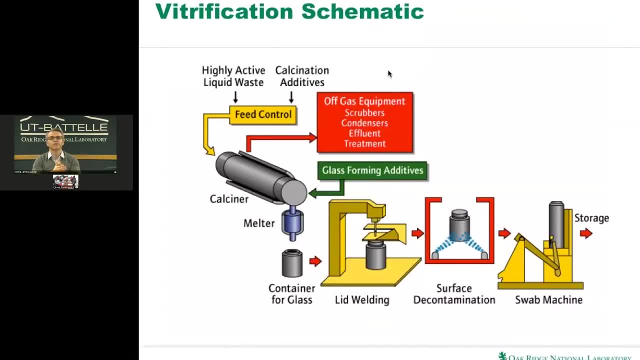 minor actinides, fission products that are all dissolved. So once you've then taken your plutonium and uranium one in one direction, you've cleaned those that you're going to purify those for future Use. you've then got all the other material that you know no longer need. 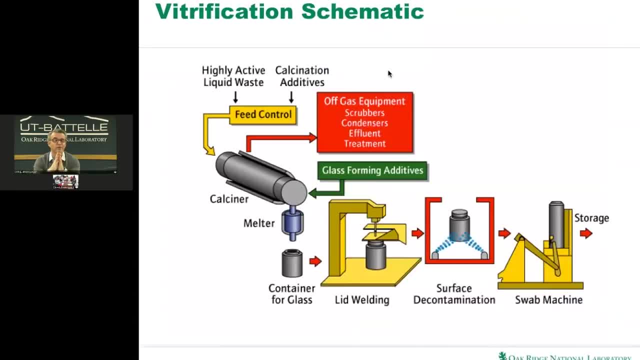 things like the minor actinides and the fission products that you then vitrify in a glass. you basically mix them with a liquid glass and that will then be put into a container, sealed up and then decontaminated, And then that's the material that eventually goes down into the repository. 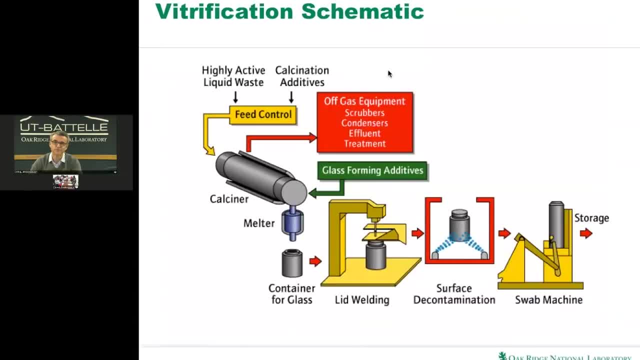 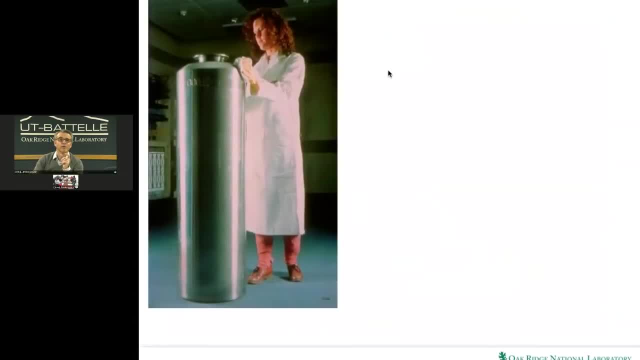 rather than the full fuel assembly, this new dissolved up set of material- And again that schematic there shows what I just outlined there- And the high level waste, as it's called, those minor actinides and fission products go into a container. 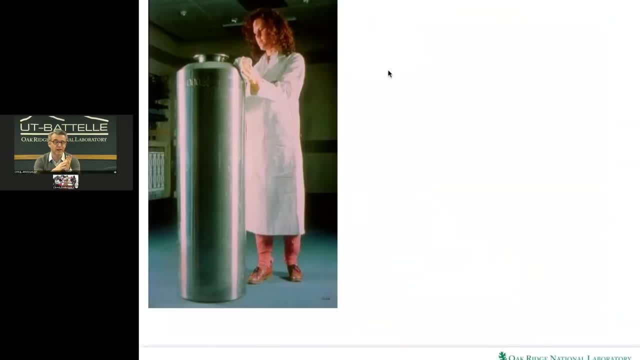 Typically. again just to illustrate size, just to be 100 percent clear, if that really was high level waste, she wouldn't be standing next to it. It's incredibly active. She would be dead before. I think people say: if you run from an 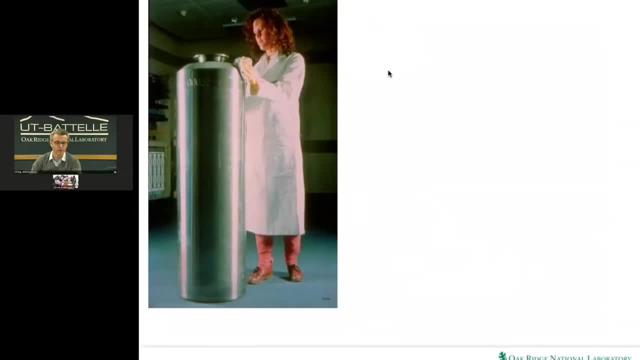 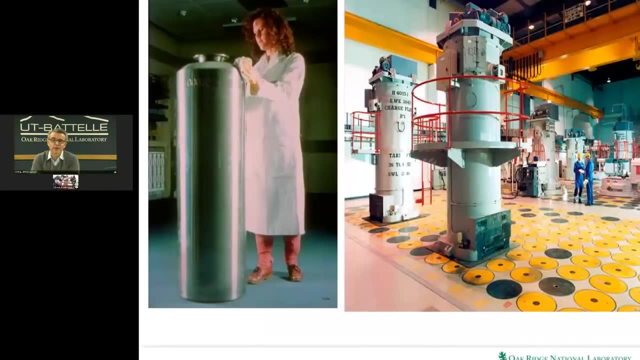 infinite distance. by the time you get to it, you'll be dead anyway, So clearly something not to be messed with. But what's interesting, though, is that, if you look at the picture on the right hand side, that's actually the high level waste store at Sellafield. 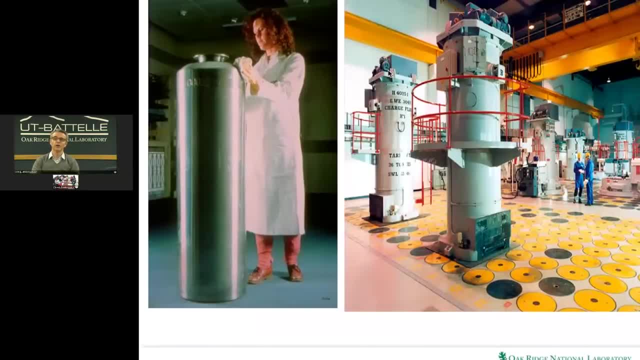 And I've actually stood on top of that on two or three occasions during my career And that below your feet there is as though those canisters stood on top of each other. I'll show you a picture in a second And again. but the radiation field because of concrete barriers and so on. 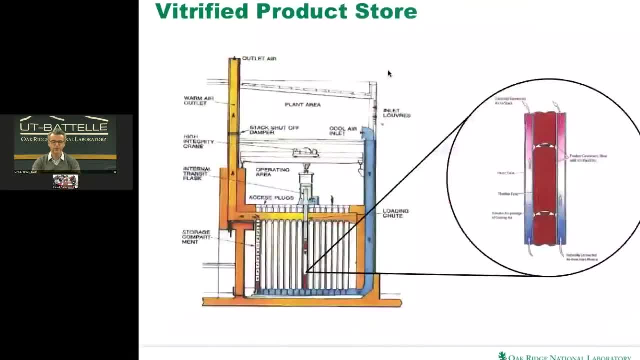 are perfectly fine. you can stand on top of that area. So here is a schematic of what you've just seen. So this is the level where those people were standing up here on the top in the plant area, And then below them are those individual canisters that I just showed. 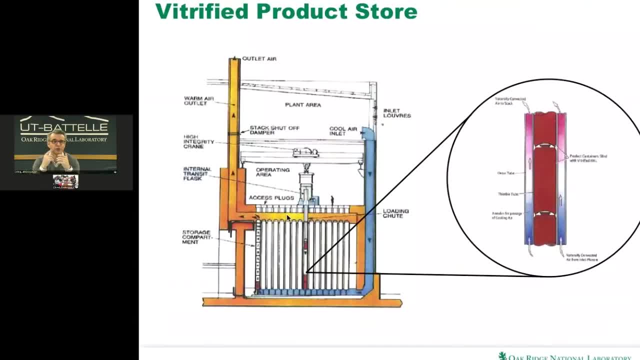 And they're stacked on top of each other, as shown on the right hand side, And that's just natural. air circulation is used And at Sellafield there's something like 50 years of high level waste sitting there from not only UK reprocessing but from reprocessing around the world. 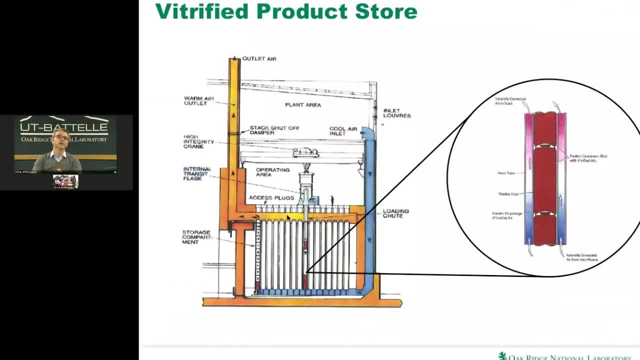 But the spent fuel volumes are incredibly small. The estimates is. you can do the calculation yourself, But the estimates are that if all of your electricity energy demands came from nuclear, the amount of high level waste that you would generate in your own personal lifetime would fit inside a small paint canister. 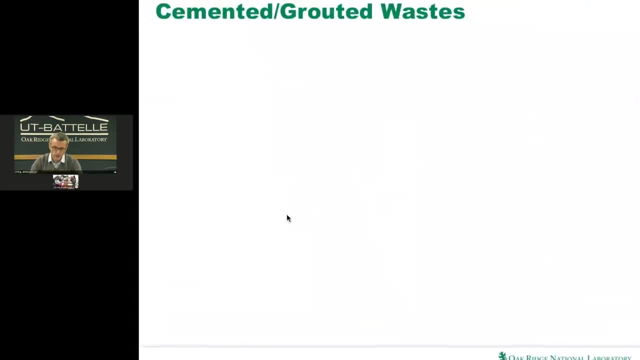 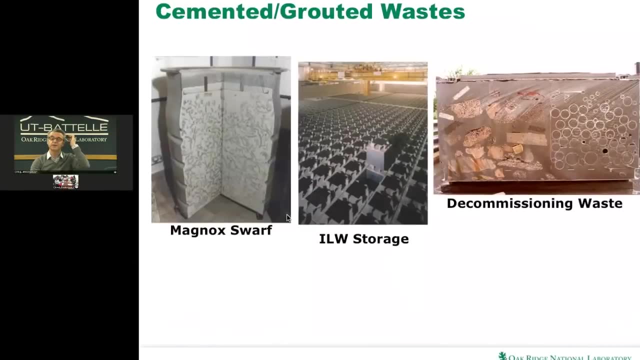 So that's why it's such a small amount of volume. But, as I mentioned, there are other wastes that come from nuclear, and so there are other processes needed to deal with the other wastes, whether that's decommissioning wastes, the intermediate level waste. 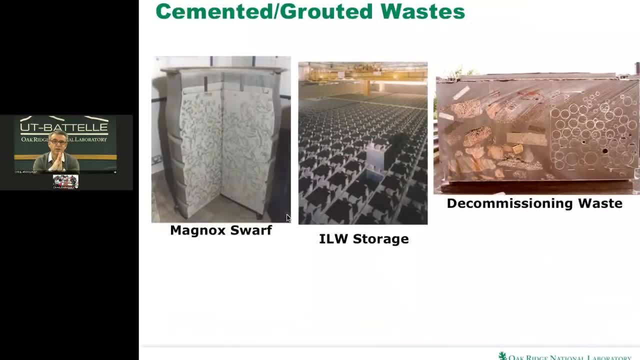 which are these, these holes, these material and mechanical pieces- And they're typically just overpacked with a cement or a grout- and then again will be sent for ultimate disposal. But still again, you still need that repository, And one thing I'll underline at this point is it doesn't matter whether you are 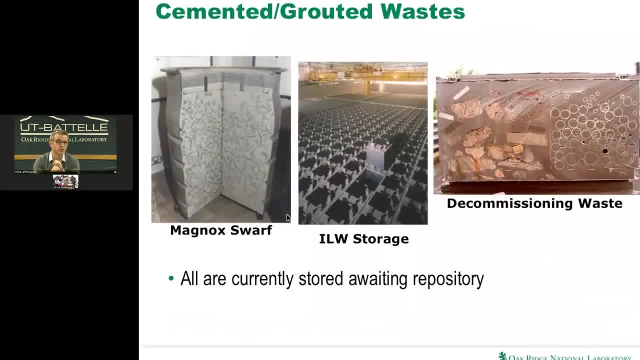 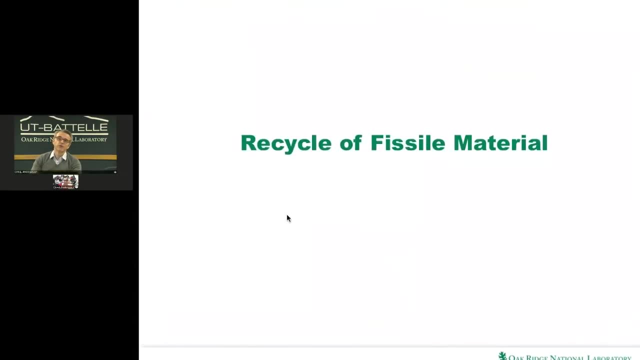 going through for a once through fuel cycle or a reprocessing fuel cycle or the ultimate, best ever fuel cycle you can think of, You will always need a repository. The only difference is how big that repository will be needed. So that's a kind of introduction to the 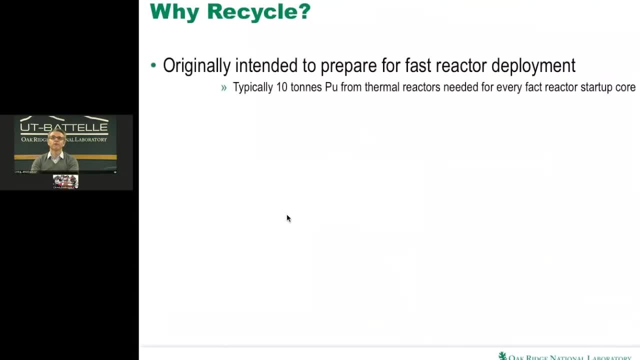 reprocessing side. So I'm going to talk about the recycling side. Typically, I think I've touched on most of these already. but you know why recycle? because we want to get the fissile material, And this really hops back to the 1970s in the oil crisis. 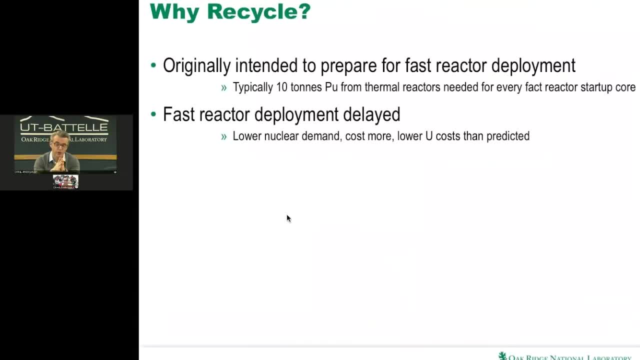 There was a big push for nuclear and a big push for nuclear and therefore a concern about demand on uranium ore, And so the concern then was: well, how are we going to address that? And fast reactors and recycle was the main driving force towards that. 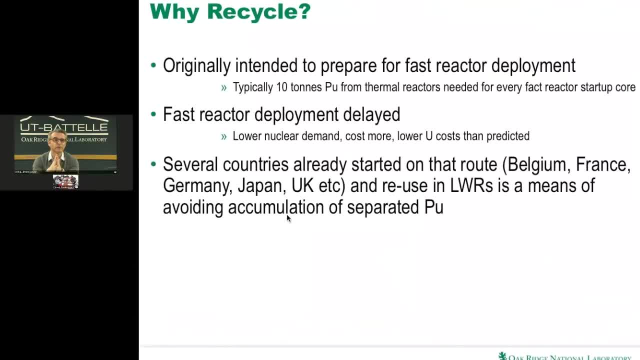 And despite the oil crisis never quite coming to fruition as everybody expected or feared it would do, several countries did start out on that route: Belgium, France, Germany, et cetera- And so they are now looking at, or actually are doing, particularly in those 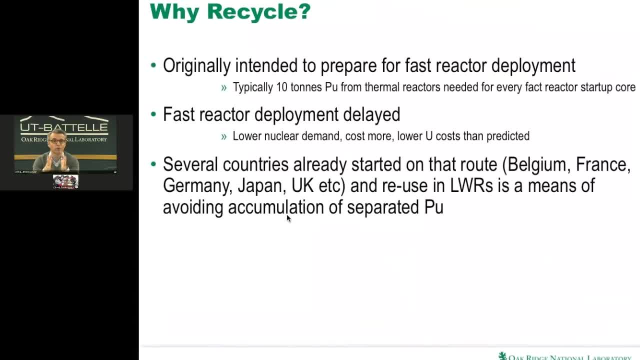 countries have looked at and are recycling their plutonium from that interim kind of reprocessing stages. They're reprocessing and reprocessing and recycling that plutonium in existing reactors. So that's that modified open fuel cycle limited recycle states that I mentioned earlier. 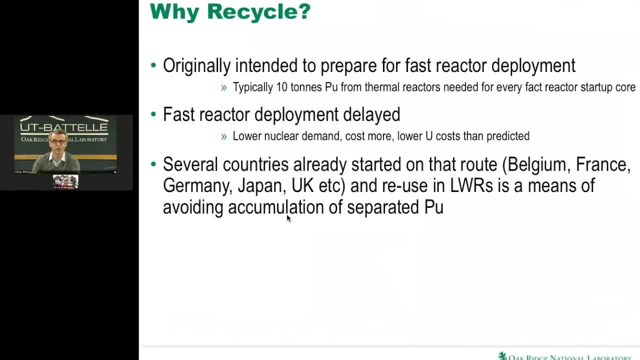 And again, the UK has something like one hundred plus tons of separated plutonium, with nothing currently planned, apart from- hopefully they'll put it in future reactors. Important point to note here, though, is that if you only recycle the plutonium and the reprocessed uranium in light water reactors, you will only see about. 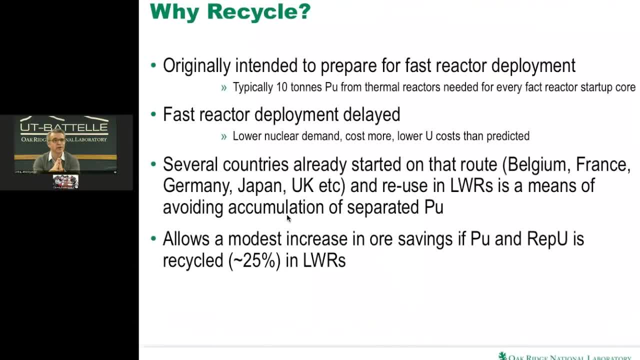 20 to 25 percent improvement in your oil savings. to get that huge, tremendous improvement You really do need to go for full, multiple recycling fast reactors. That's why that isn't quite getting to the full potential. The other thing just bear in mind is that on the current uranium markets, 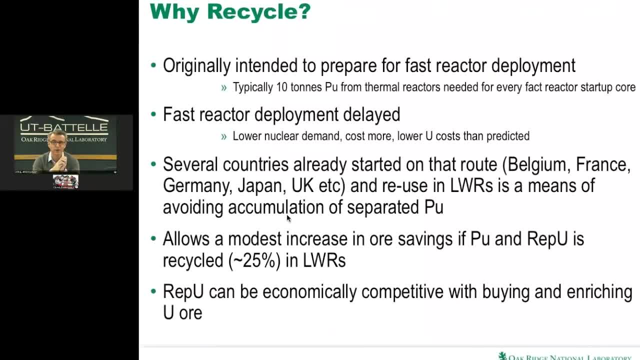 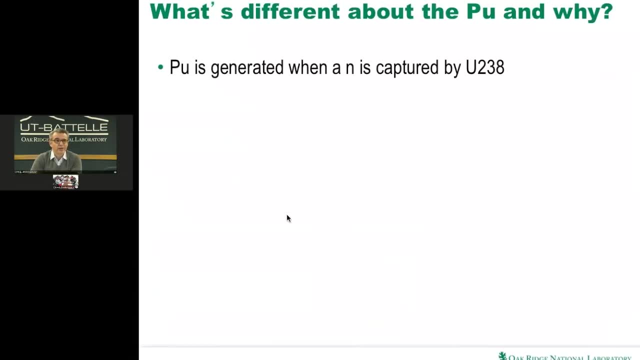 the reprocessed uranium can be economically competitive with buying uranium or fresh. So again, in France, there's a lot of, actually, that's already going on. They are recycling not only their plutonium, but also their reprocessed uranium. The thing is, though, not all plutonium is created equal. 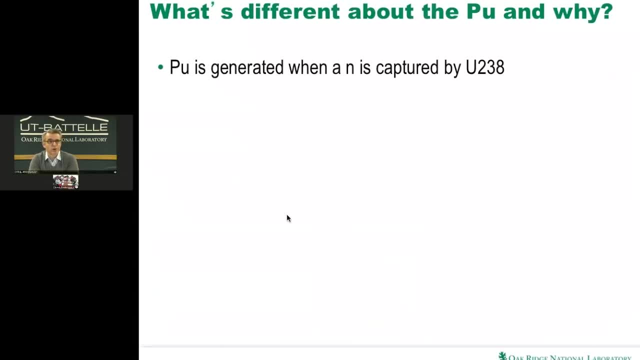 So you often hear people talk about weapons grade plutonium or bomb grade plutonium or civil grade plutonium and all these other things, And it is different And just want to give you a very quick explanation as to why it is different. So plutonium is generated in a reactor. 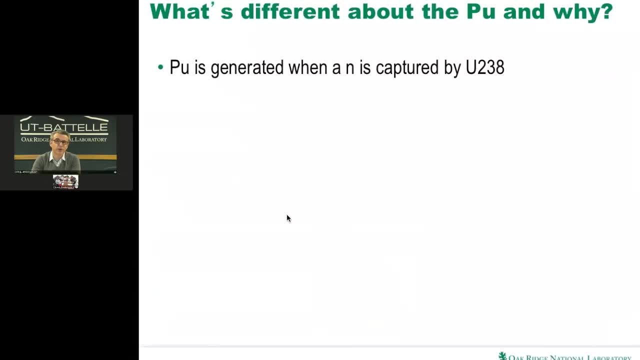 It's the only place it's generated. It's not natural. And it's captured. it's produced by a uranium 238 neutron capture. So uranium 238 captures a neutron, becomes a neptune 238.. In the case of plutonium, 239, 238.. 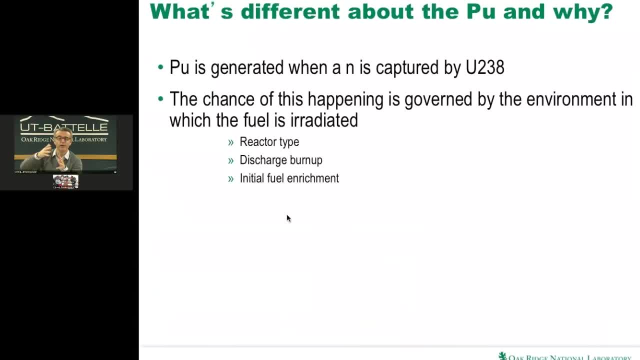 And then it can go up through that chain and it can capture the 238,, 239,, 240,, 241,, 242 and so on. So the chance of that happening, the chance of that neutron being captured at U238, well, is very much dependent on the reactor environment that it's in. And it also depends on how long the fuel is in the reactor for, because the longer it's in, the more chance of capturing a neutron and therefore the more plutonium is produced. But if you leave it in too long, then that plutonium begins to fission and then the plutonium composition turns over. 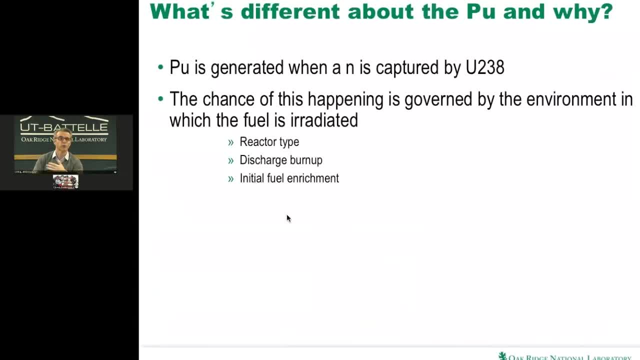 And also, depending on the initial enrichment, is it naturally enriched fuel that you originally put into that reactor? That also affects it, because you've got different amounts of U238. And the relevant abundance of all those plutonium isotopes is what's known as the plutonium vector. 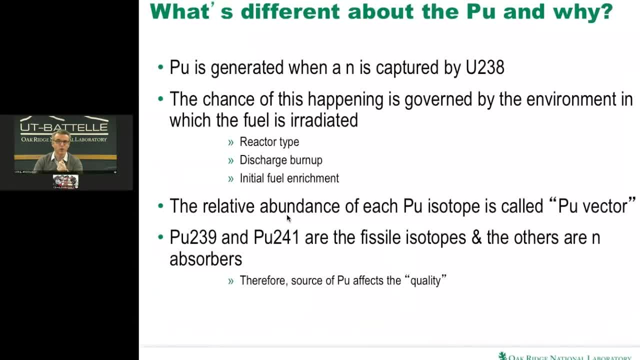 And the combination of the plut 239 and plut 241, which are the fissile isotopes, whereas all the even isotopes are neutron absorbers. that affects the plutonium quality. The quality is governed by how much fissile material we have. 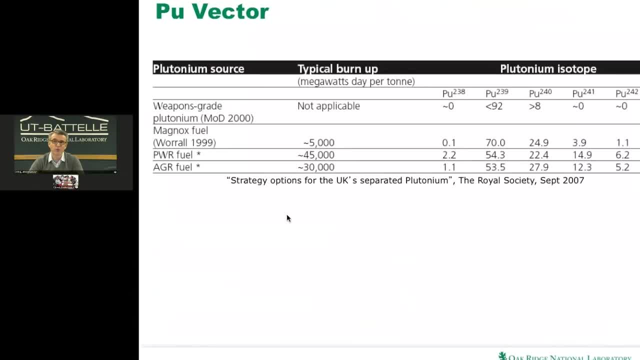 So just to illustrate that, if you look at weapons grade plutonium, it's pretty much all plutonium 239.. And again, all this material that's in this talk, including this slide, is unclassified, so don't worry about any information in there. I should have underlined that at the beginning. So the other thing as well is the weapons grade. plutonium majority is 239.. If you look at the Magnox fuel in the UK- you look again- it's quite a good fissile material because that used to be the source. 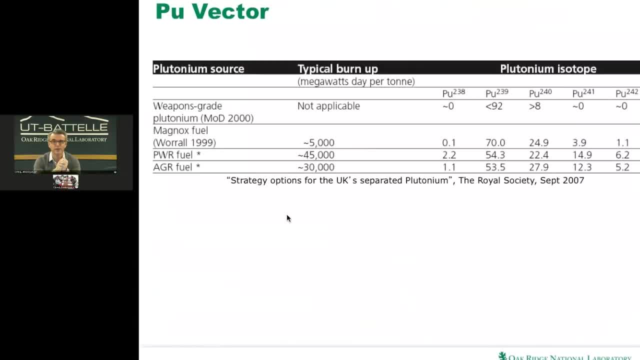 of the UK's plutonium for their bomb program. So again, it's a nice reactor that generate plutonium. And also you see how the commercial reactors like the pressurized water reactor or the advanced gas cool reactor, they notably affect the fissile quality. 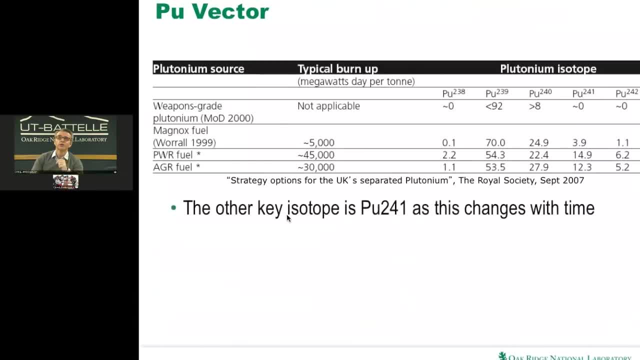 The 239 plus 241.. So why is that important? Well, the other thing you should also bear in mind is that the plutonium 241 concentration will also change with time, because plut 241 decays to americium 241 and americium 241 is no longer fissile. 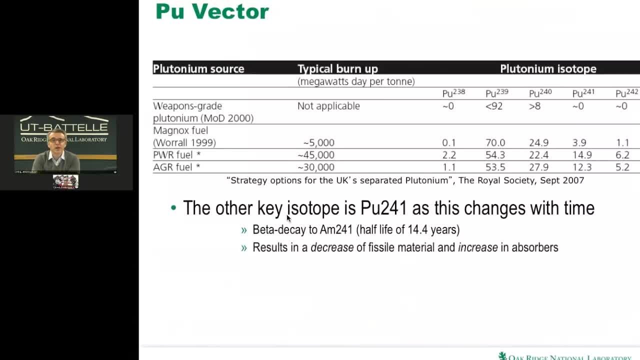 So you actually over time lose your fissile quality And also the americium 241,, unfortunately, is also a neutron absorber. So over time if you've made a strategic decision to separate plutonium to reuse, it actually makes more sense to use it earlier because you're going to be losing. 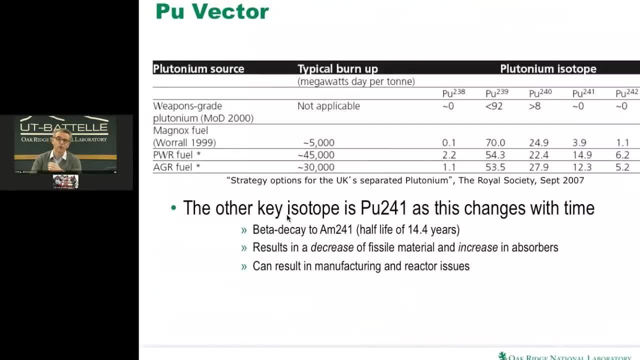 your fissile material over time. And unfortunately, the americium 241 is also a dose consideration, a dose issue, And so, again, if you're not careful, you can end up with a situation that you can't actually use it any longer. 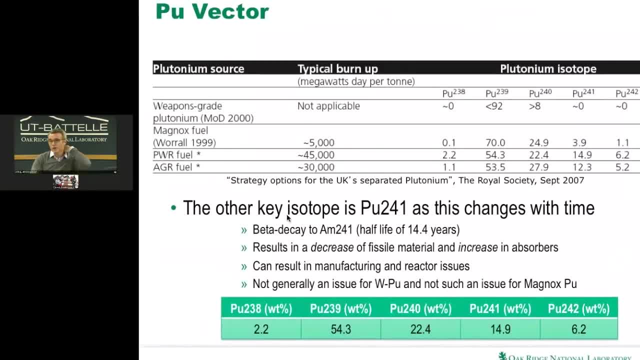 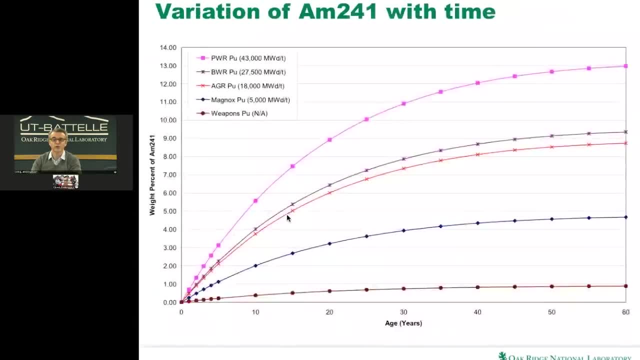 in your fuel fabrication plant. So typically these are just some kind of examples, as I said, the kind of typical concentrations you'll see, And this just shows you how, depending on your original plutonium that you've got, how much americium will build up over time and why it does or does not become. 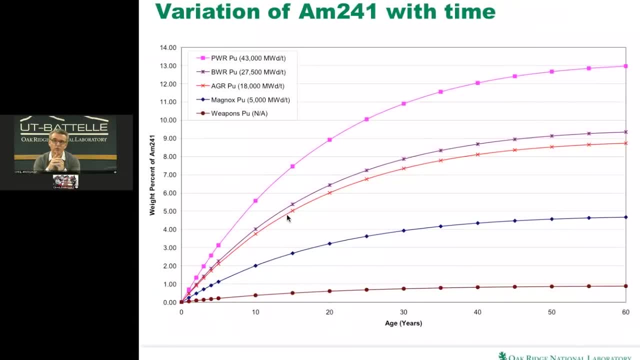 as a concern. So if you look at the second line from the bottom, which is the Magnox plutonium, the UK is able to store its plutonium for a long, long period of time without much concern about americium ingrowth And therefore making a strategic decision. 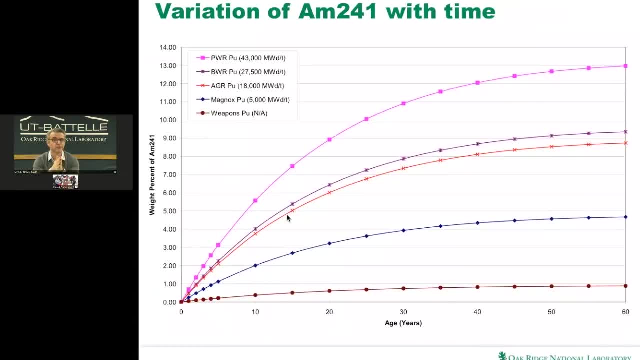 about recycling. plutonium is not such a tight timescale, Whereas if you're France, for example, and all your reactors are pressurized water reactors, then after only something like 10 years your americium ingrowth has got to typically 3,, 4, 5 percent. 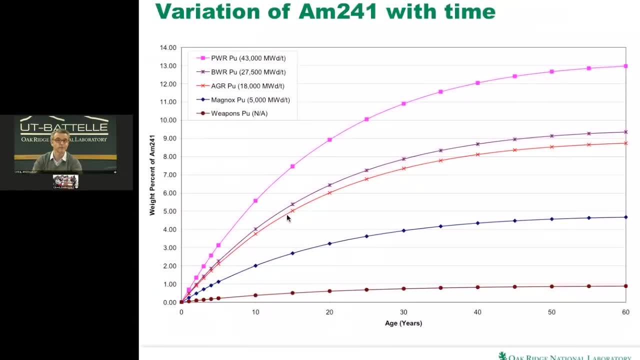 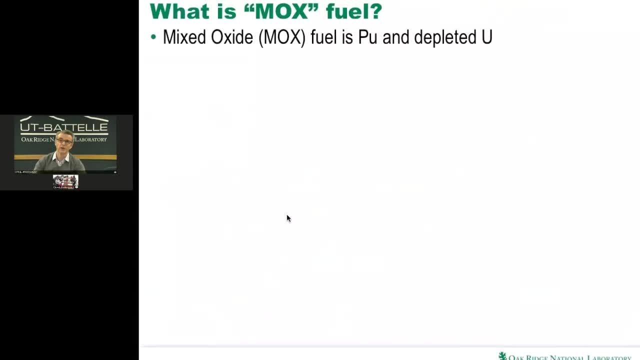 And that's certainly higher than fuel fabrication plants are able to tolerate. So you need to do something more quickly. What they do is they load it into what's known as MOX fuel- mixed oxide fuel- and that's a combination of plutonium which makes about 10 percent of the fuel. 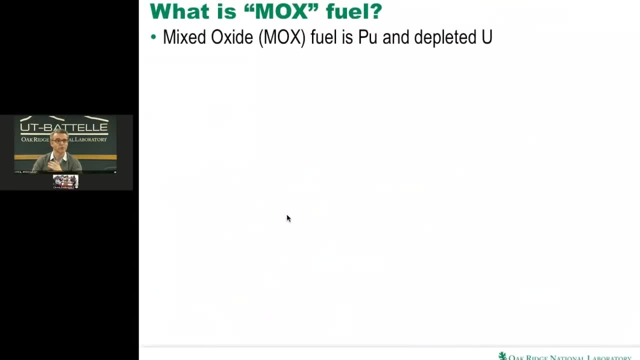 and the other 90 percent is depleted uranium, The material that, when we have enriched uranium, goes one way the other way. the depleted is what's the byproduct of the enrichment process. So, depending on how much energy we need to get out of our fuel, 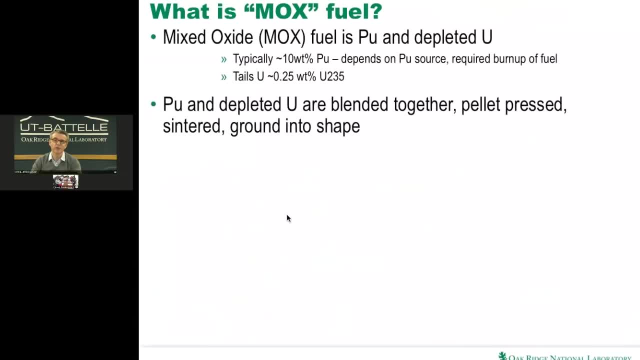 we increase plutonium content, tails uranium I mentioned is depleted uranium. We blend those together, we press them, we make it into new fuel and again, I'm not going into the details, Again just conscious of the time. But you just have to be careful with this plutonium as well. 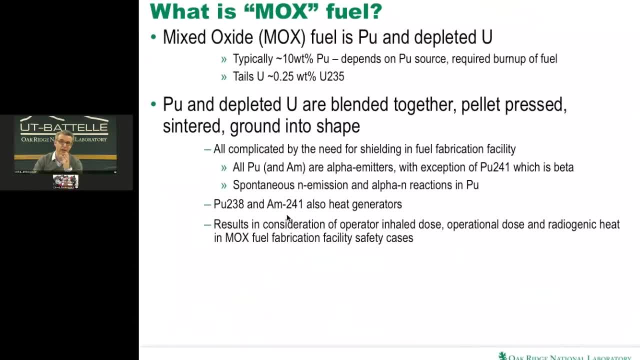 because it's also now with plutonium. they're heat generators. You have to be a little bit careful in terms of the fabrication process and so on. But the key point here really is that if you were to look at a fuel design, a fuel element that had plutonium fuel in it, 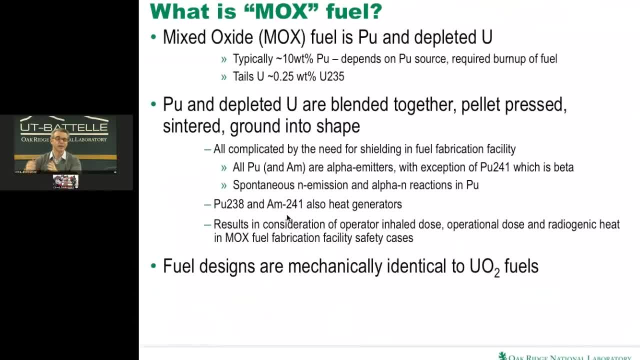 MOX fuel in it versus one that had uranium only in it. you couldn't tell any difference. They're actually identical mechanically. The only difference is, though, in a MOX fuel fabrication plant, because of the dose from the americium, because of the dose and the heat from the plutonium. 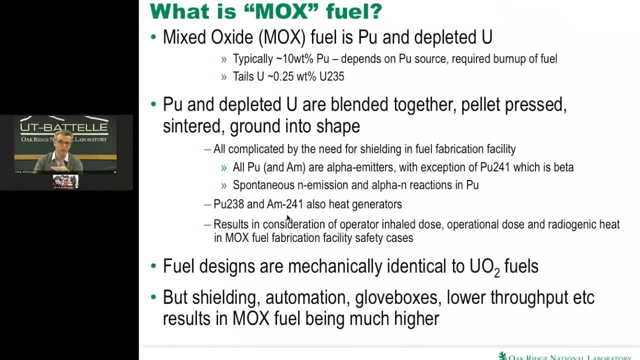 you need to make sure the shielding in place. glove boxes become incredibly important. there's a lot of automation in them, less hands on operations compared to the uranium facility, And all of that, plus all the additional security that's necessary and so forth, makes in fact. 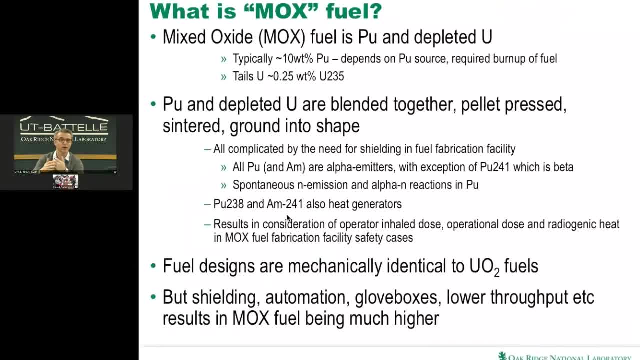 MOX fuel very much more expensive than uranium fuel And that's why, again, it doesn't seem to make sense today to go forward with the MOX fuel as on a commercial basis, unless you've already decided to separate out for a different reason. back to the things I said earlier. 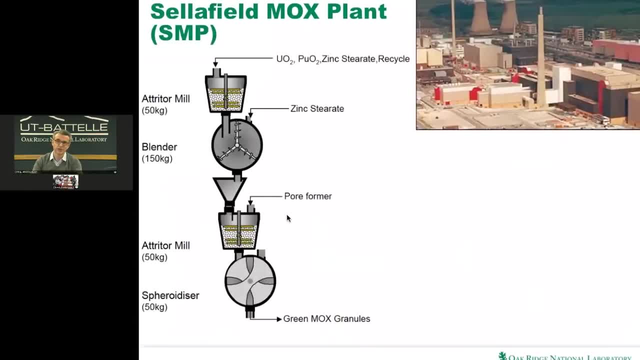 So again, this unfortunately is an old slide, because the Sellafield MOX plant is actually now closed. the UK government decided to close the facility, But on the photograph on the right hand side the red and black building on the right hand side is the end of the chemical separations. 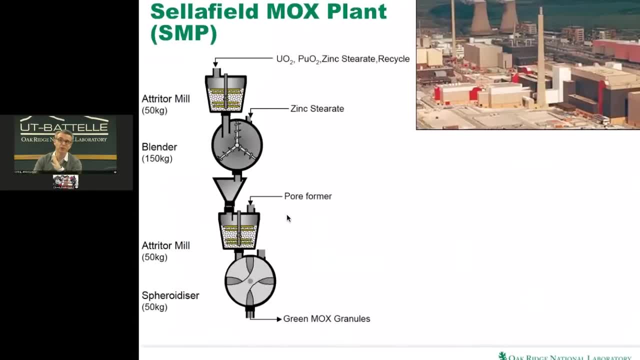 plant in Thorpe that I showed you the photograph earlier, and the building that comes out to the left is the Sellafield MOX plant. So the MOX fuel fabrication plant is almost inextricably linked to the reprocessing business, because the product that comes out of the reprocessing is plutonium. 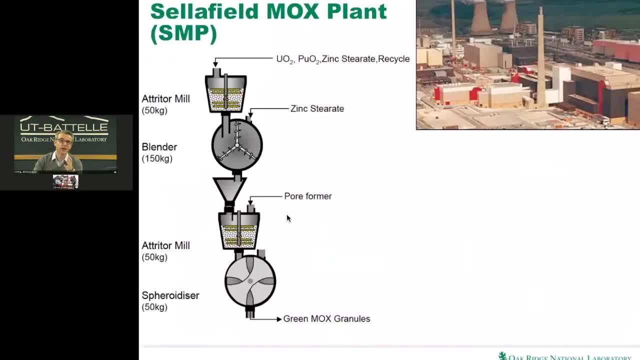 And that's the feed material straight into your fuel. So this is again. I'm not going to go into the details, but just to demonstrate the processes. you mix the uranium and the plutonium together, you kind of mill it together, and then you add pore formers and you produce pellets. 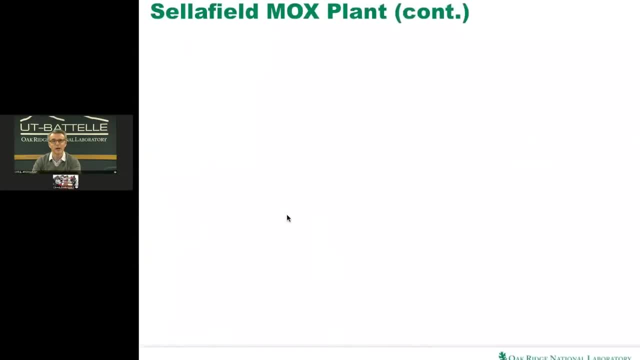 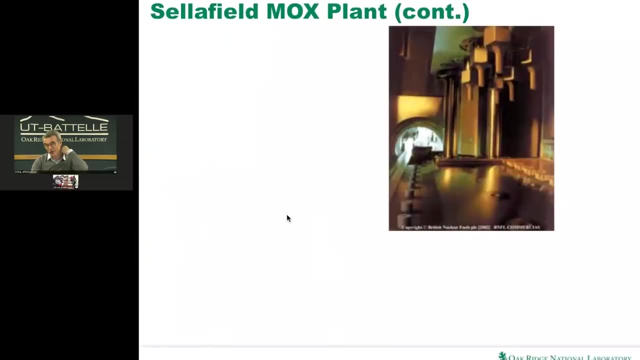 And again, this is just to show you some photographs of what these things look like. And again, I'm not going to spend time on this because, again, it's just some photographs to illustrate. But again, for those people who may not have seen what fuel pellets look like- bits of fuel pellets being pressed- 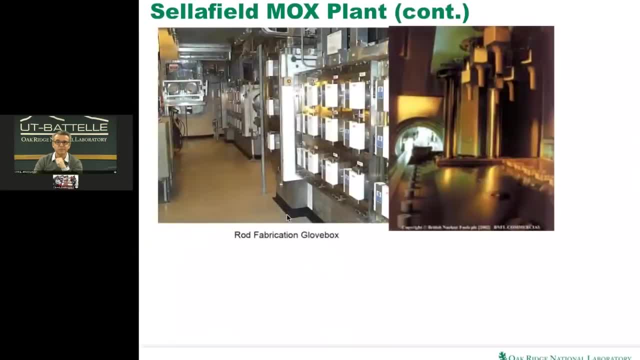 You're seeing the dyes on the right hand side that press those pellets And then, as I mentioned, everything's behind glove boxes. For anybody who's seen a fuel fabrication facility for uranium fuels, you don't see all this kind of glove boxes. 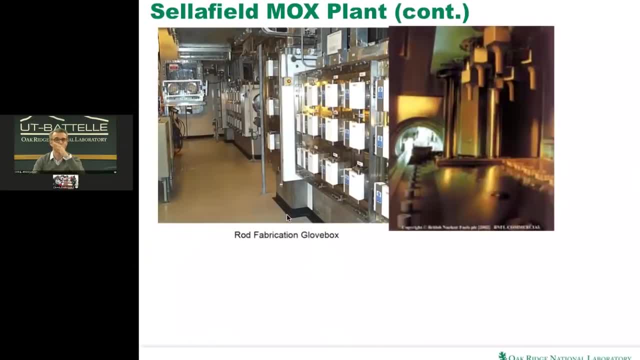 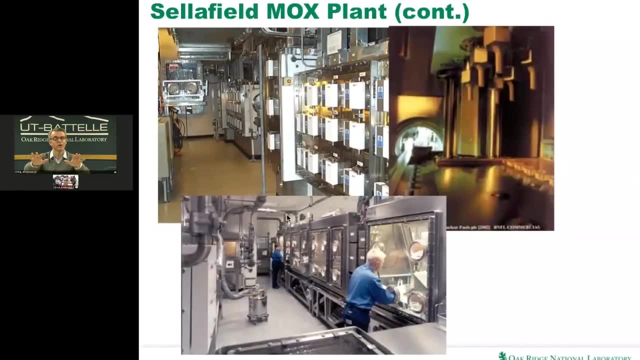 You can see things much more clearly as to what's going on. It's not all inside containment, as you've seen here. So again, you can see how much more the operations become difficult because of all the manual detachment that's needed. You need either remote handling or inside glove boxes and so on. 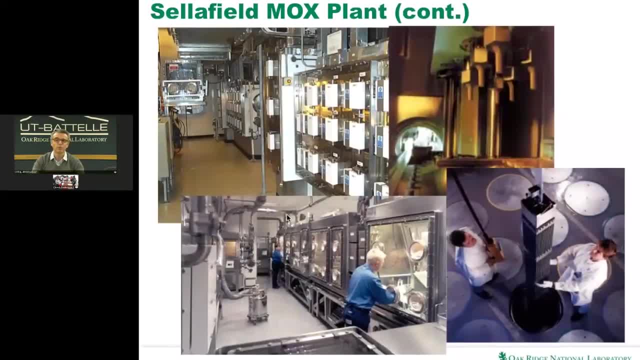 So things like maintenance become very difficult on these things. But once it's inside a fuel assembly, as I said, there's no difference And in fact more often than not you can handle that, Apart from it's a little bit. 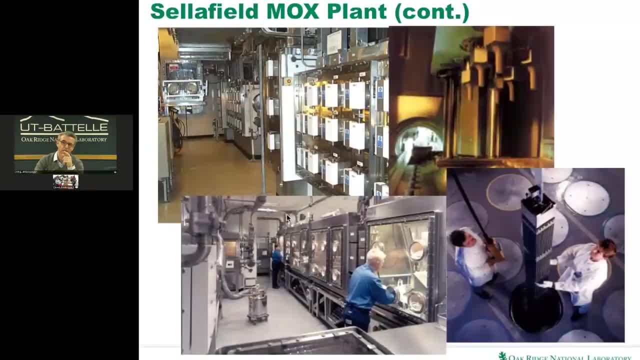 you'll feel it's a little bit warmer on the outside just because of the plutonium decay. The guy on the right hand side is wearing gloves. just to be clear, he's wearing gloves not because of concern about contaminating himself. It's concern about him contaminating the fuel assembly, because what we don't want 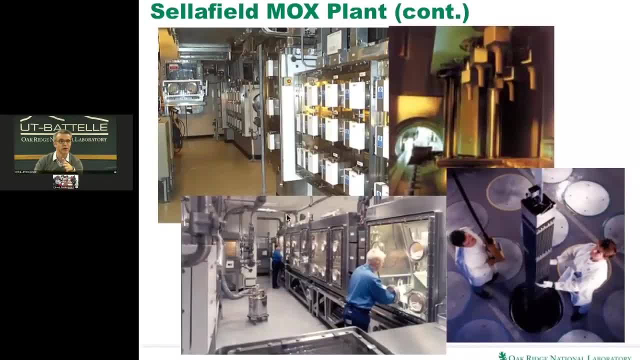 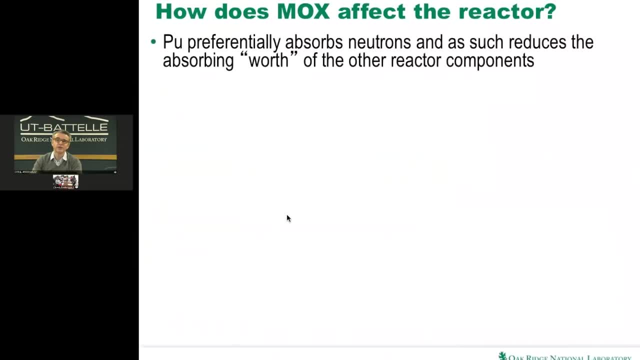 to do is people to leave greasy fingerprints all over a fuel assembly. It's going to go into a reactor because that can affect the reactor performance. so to protect the fuel assembly, not him. Again, I'm not going to go into the details. 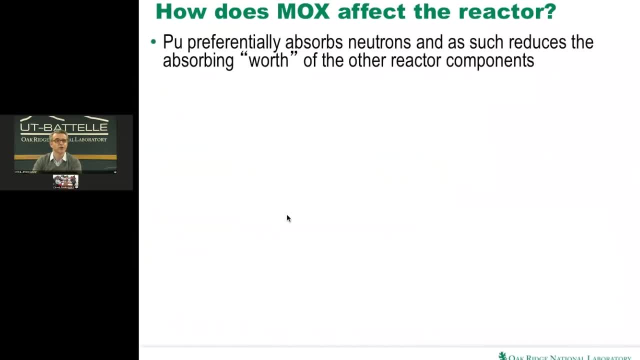 because this is more my background in reactor physics. That's why I threw these in there, because I find it quite interesting. But really the important thing is that MOX does actually have an impact on the reactor operations. It's not something that you can just load into a reactor without any consideration. 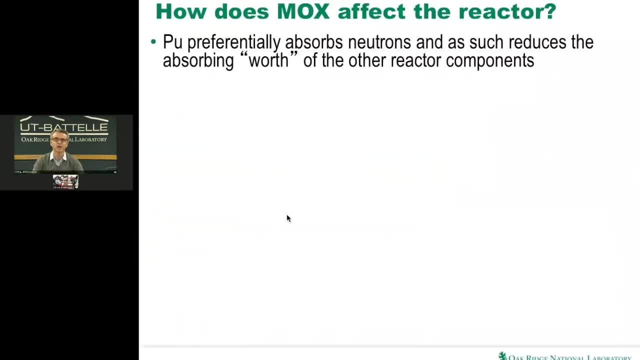 You have to do new safety analysis. There are limitations on what you can do And the reason being, unfortunately, is that plutonium preferentially absorbs neutrons, So you've just fissioned uranium and plutonium. You generate these, these neutrons that you want. 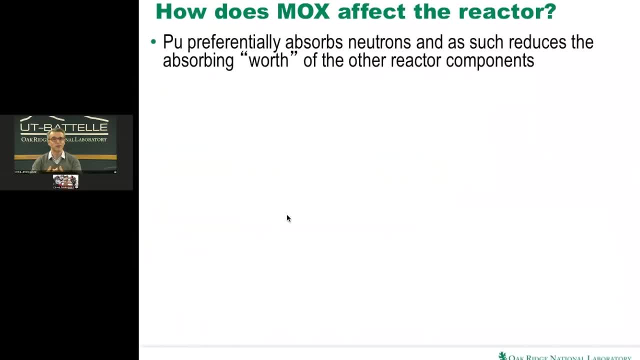 But unfortunately the plutonium itself preferentially absorbs those neutrons that you may need other materials such as the control rods and the shutdown systems of the reactor to utilise those neutrons. Unfortunately, what it means is they reduce the absorbing worth of control rods. 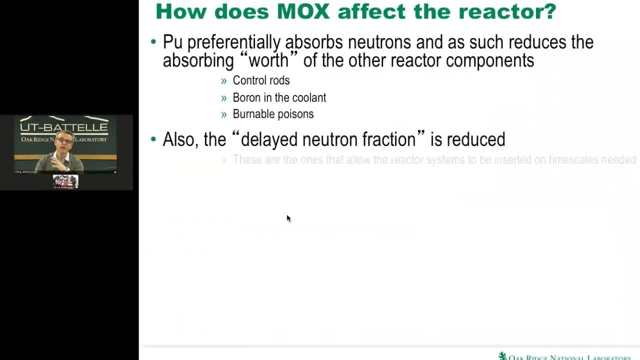 of the coolants, of the burnable poisons and so on, And again, I'm not going to go into this detail. This is just for your broader knowledge, in a sense- but also things like how you control the reactor using delayed neutrons. 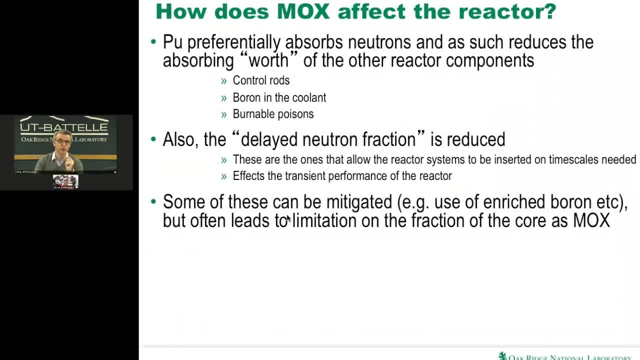 They're affected because the number of delayed neutrons is reduced. You can affect, you can limit, mitigate some of the effects. you can do things in reactor operations. you can do things in your safety analysis. you can put in extra systems. 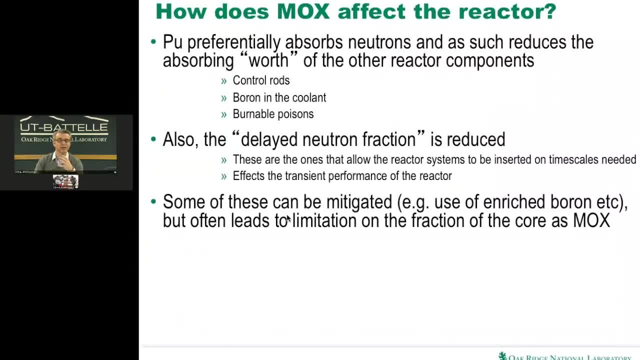 control systems, but generally what people do is they just simply limit the fraction of the fuel that's allowed in the reactor, But normally it will be. 100 percent of the reactor is uranium fuels, of course, But it tends to be. we don't load 100 percent of the reactor as MOX fuel. 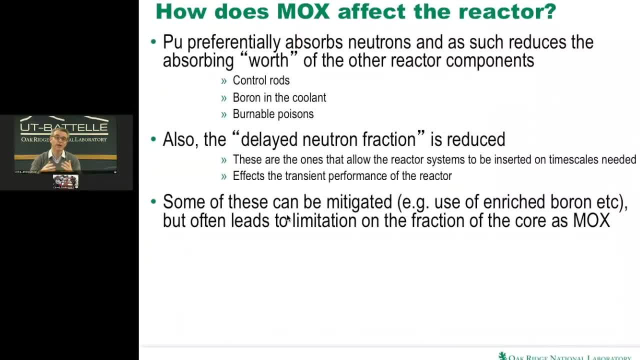 If you look in France and other places, typically one third of the reactor is loaded as MOX fuel and two thirds as uranium fuels. Again, the details aren't so important, but the fuel performance itself is also affected by the presence of plutonium. 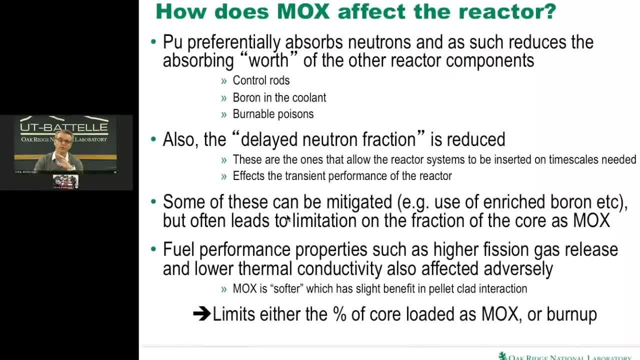 Again, I'm not going to go into the details, but the key takeaway again from all of this is that generally MOX fuel A costs more and B has an operational impact on the performance of your reactor that you have to mitigate against by a range of things. 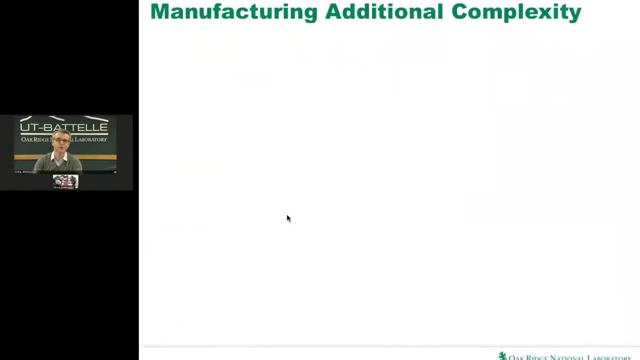 that I've listed here. That's the takeaway from this really is. it's not quite as just as simple as you use uranium fuel- And again I'm not going to go into the detail- but the manufacturing process is much more complex because usually in a uranium fuel assembly, 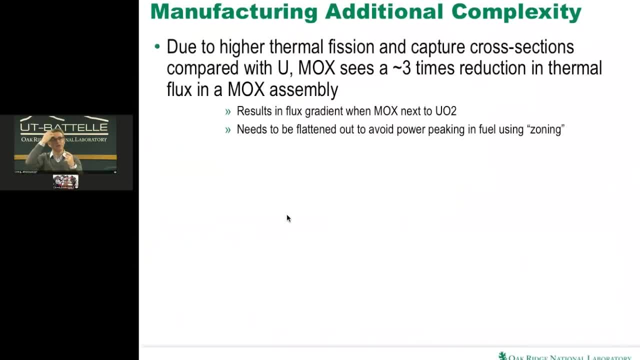 certainly for a PWR- we only have one enrichment. So what it means is you can manufacture all of your fuel rods with exactly the same same enrichment, same pellets, same everything, But unfortunately, with MOX fuel that's not the case. 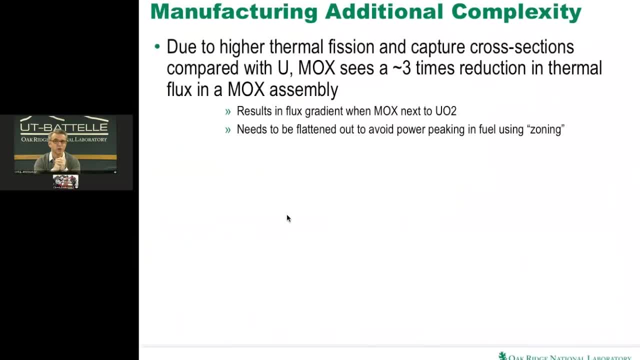 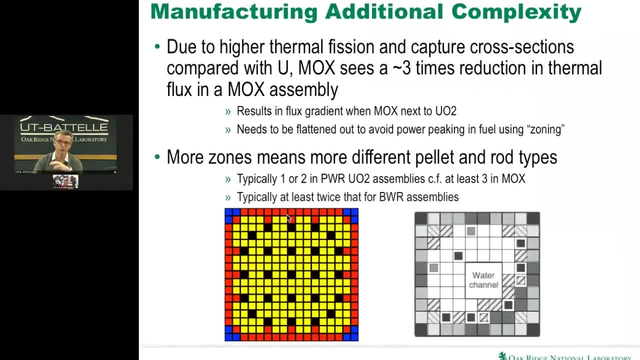 Because of the MOX and uranium kind of cohabiting in the reactor, you have to have a much more complicated plutonium distribution in your fuel. So again, I'm not going to go into that. This is just to illustrate the differences for PWR and BWR fuel assemblies. 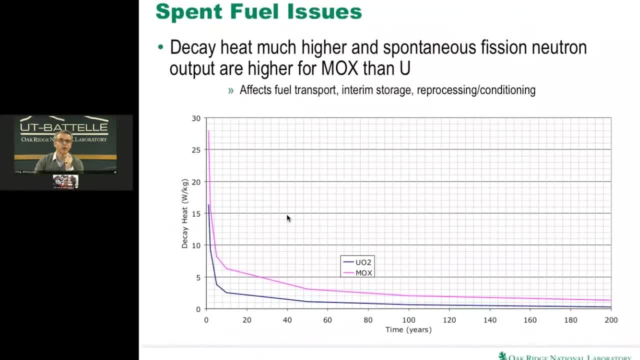 The one thing I would say, though, is that the plutonium, and therefore the MOX fuel, does have a much higher spontaneous fission neutron output than uranium, And because of that, has a much higher decay heat. And because of all the decay heat considerations, what you end up with is 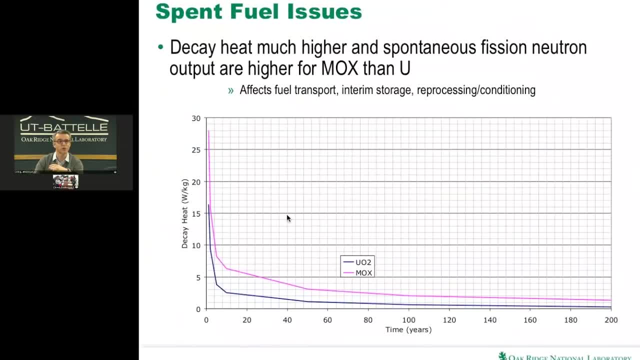 something like a factor of three or four more heat in a MOX fuel assembly than in the uranium fuel assembly. so that has significant implications on the spent fuel pools of the reactor, but also on your repository performance if you are considering putting MOX fuel in your repository. 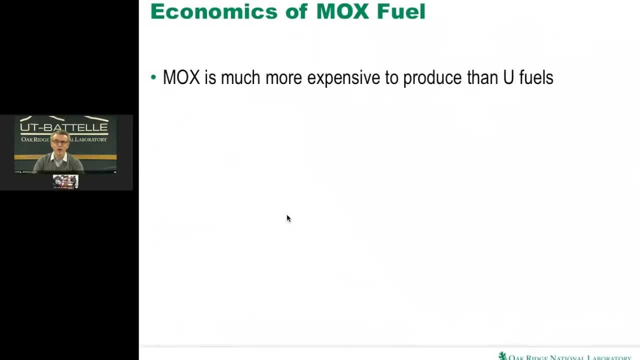 So again, there are spent fuel issues to be concerned with. I've already touched on this. if so, I won't spend time on this. but just to reiterate, MOX is much more expensive than uranium, typically two, three or four times. 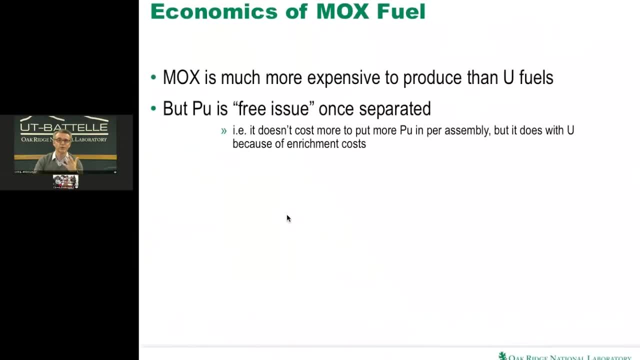 But if you've decided you want to go ahead with recycle for a whole range of other reasons- and plutonium is a free issue once it's separated- it does give you the benefit. because it's free, You can kind of load more and more and get more energy out of your fuel. 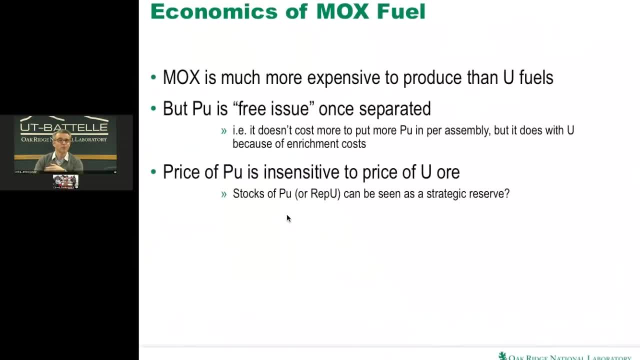 Also, the price of plutonium is insensitive to the price of uranium. So if you are sitting on a stockpile of plutonium like the UK and France, what it means is that if suddenly there's a surge to uranium, and oil prices for uranium spike, which they have done- 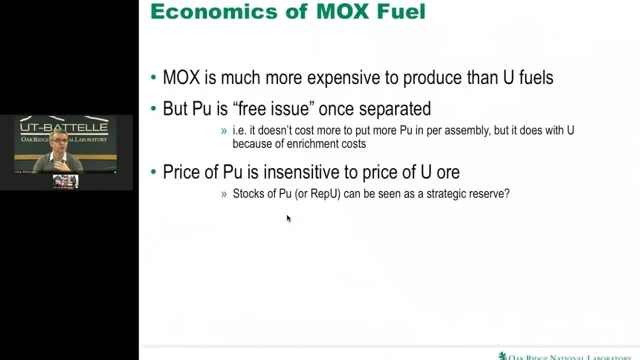 in the past. you can kind of offset those costs with a bit of a strategic reserve by reusing your plutonium or indeed your reprocessed uranium And again overall, as mentioned, reducing the volume on the repository and so on and the impact there. 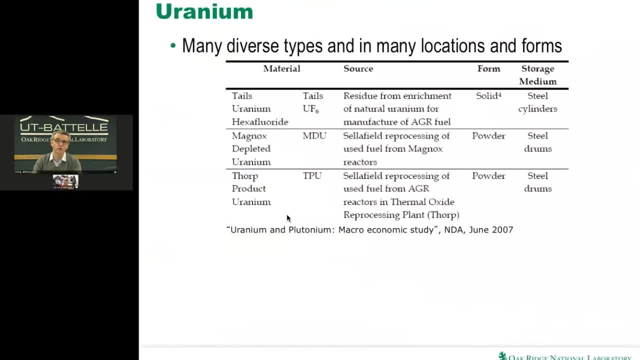 You can also reprocess the uranium. There's a lot of uranium around different parts of the world And again this is just to illustrate from a report from the Nuclear Decommissioning the NDA. there's a range of tails: uranium, depleted uranium, reprocessed uranium. 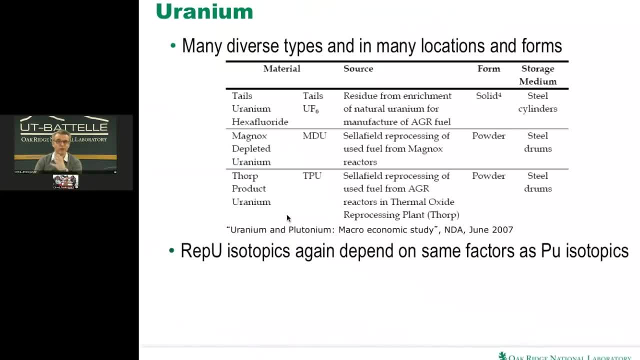 And again, the isotopics that you see in all of that fuel, in that reprocessed uranium, depends on a range of factors, exactly the same factors as the plutonium isotopics. And again, just an illustrative example, if you look at the uranium composition of the reprocessed uranium, 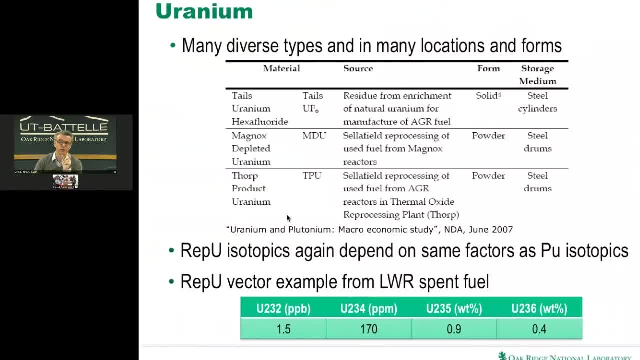 typically it's dominated by, you know, U-235 is left about 0.9 percent. You start with about four or five when you first put the fuel in the reactor. It's now fission depleted down to about 0.9.. 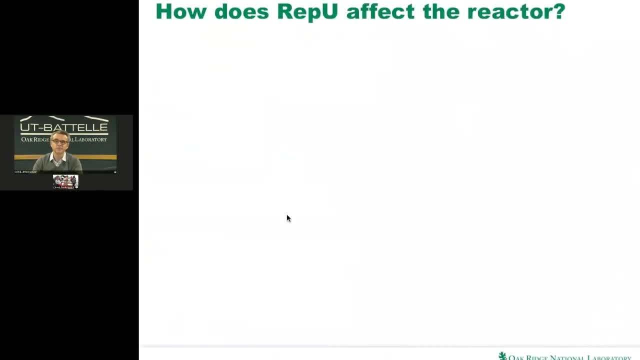 But you've also produced the other uranium isotopes. It really doesn't have a huge effect on the reactor itself, so it's quite useful, But you do have to be careful, because the U-234 and U-236 actually absorb neutrons. They don't contribute to the fission, So you need to over enrich the U-235 to compensate for that extra. And the other thing- this becomes of interest to the thorium fuel cycle also- is that the U-232 byproduct that comes from this has a quite significant 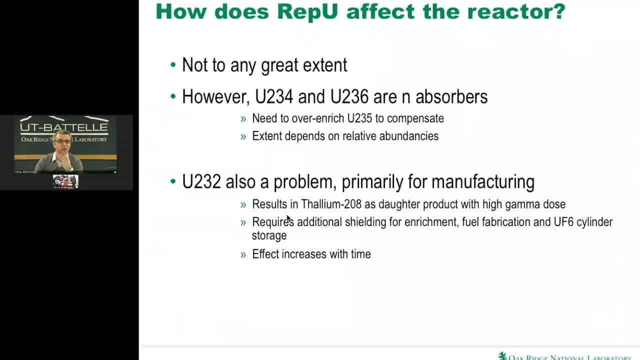 daughter product, thalim-208, that has a very high gamma dose- 2.6 MeV gamma- And so what that means is, if you're considering recycling uranium, you then need to think about the shielding implications on your fuel fabrication. 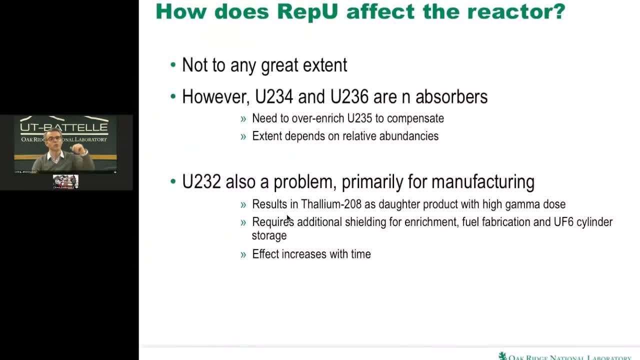 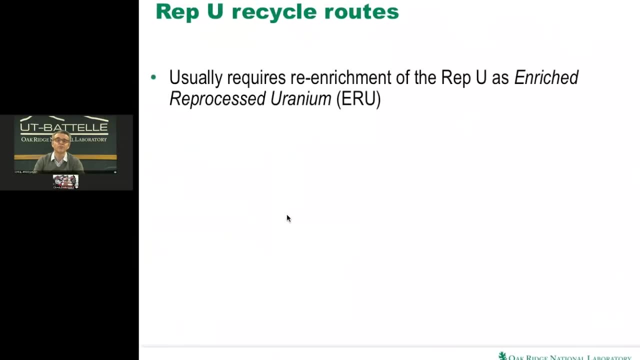 plants and that effect increases over time because over time you'll grow in more U-232.. And also, what it means is now that your enrichment plant and all of your standard uranium fuel cycle plants also have now been contaminated with these materials So you can recycle. it's known as enriched, reprocessed uranium. 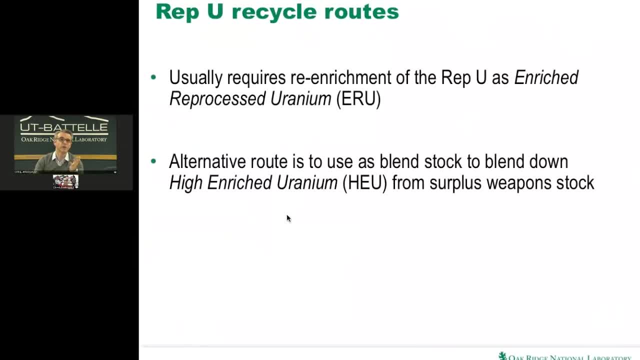 once you re-enrich it into a new product. there are other options to maybe use that material down, blending HEU from surplus weapons program, And in fact there's a program of work currently going on with Canada and also in South Korea, where they're. 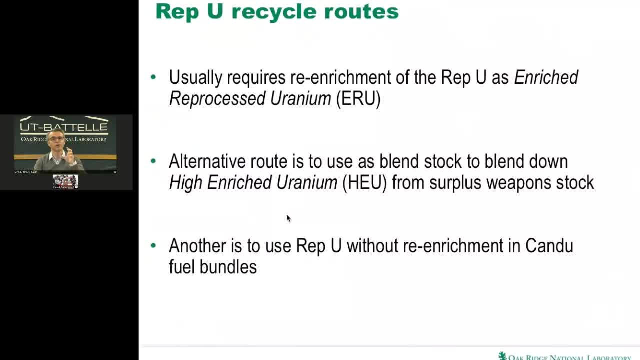 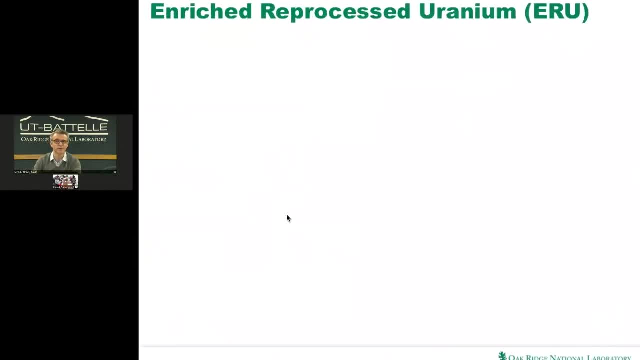 using the reprocessed uranium from light water reactors and are able to load that directly into a CANDU reactor, because CANDU reactors don't need enrichment, They just need a natural background. you know: 0.7% U-235. 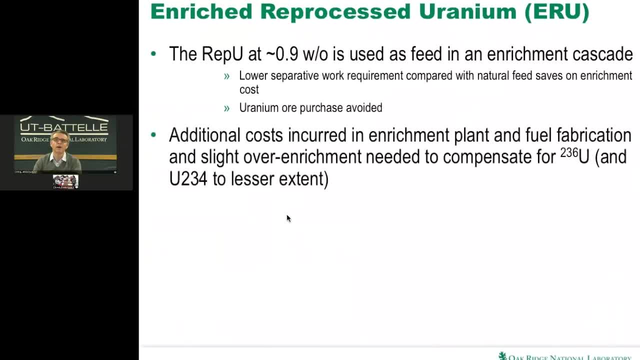 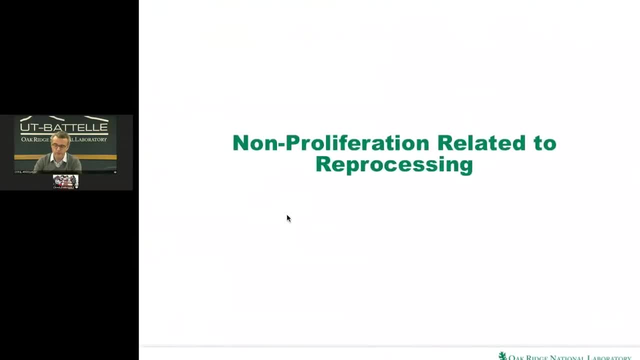 Again, not going to talk about this. this is just to illustrate some of the points I've already made about the additional costs and the violation of limits and so on, So I'm not going to go into this. it's probably more to detail than you need. 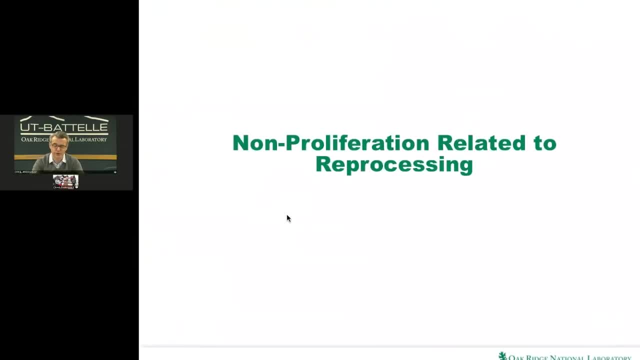 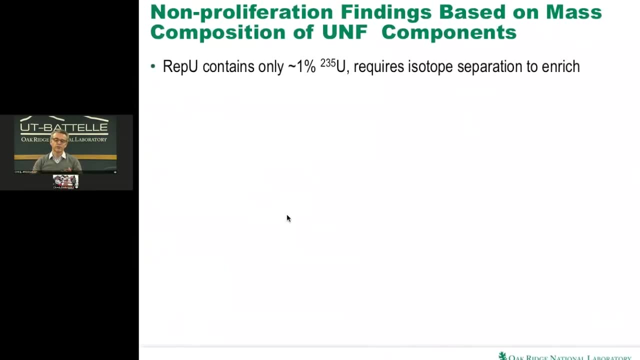 So just to come back to the reprocessing and kind of cover this from a non-proliferation and safeguards perspective, There are a whole range of, obviously, concerns with non-proliferation and safeguards. Usually it's about material attractiveness, So that's what we kind of focus on. 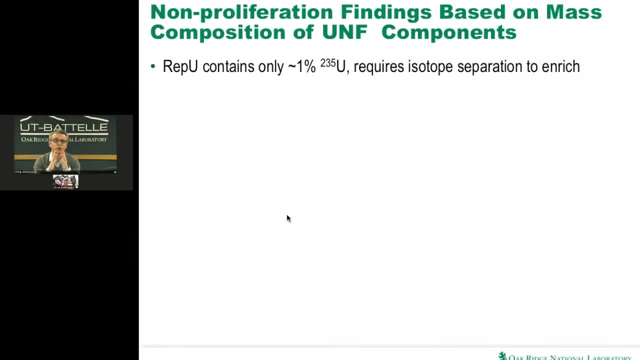 But you have to bear in mind that if you look at the reprocessed uranium that comes from recycling, as I said, the U-235 content now is very low, typically 1% or less of U-235. And you need isotope separation re-enrichment to take that any further. 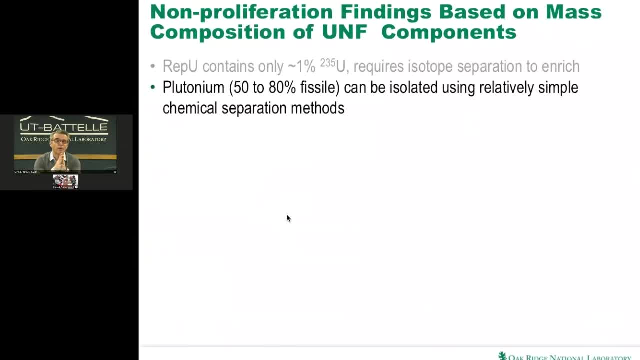 However, with the plutonium that comes from that, typically you've got about 50% to 80% fissile. And again, if you look at Chuck Bathke's work on the figure of merit and the material attractiveness, he demonstrates that that material, that plutonium quality, is still. 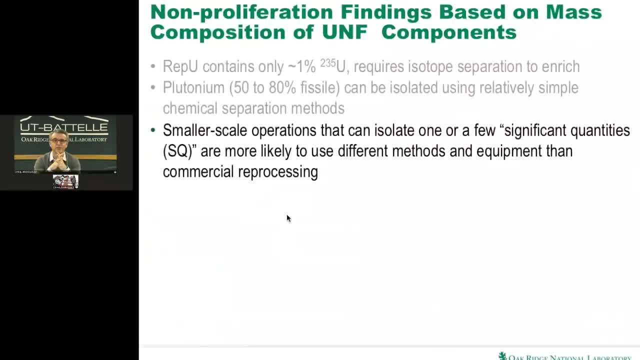 sufficient for a weapon still weaponisable, has material attractiveness. There are smaller scale operations other than commercial reprocessing that can be used to isolate just a few significant quantities And again, it's they're more likely to be used than commercial reprocessing plants. 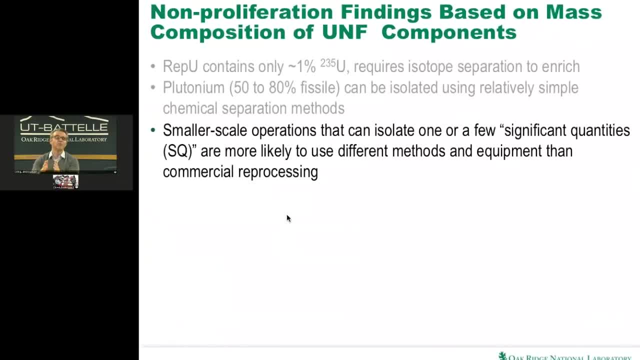 And again, that's just something to bear in mind. There's often a big difference between research programmes that are going on around the world and significant commercial reprocessing plants. So again, just bear in mind that the different techniques can be used depending on the application. 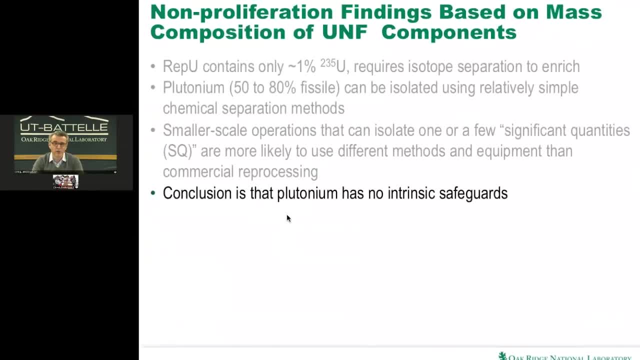 But the conclusion from all the studies in this Chuck Bathke one I keep alluding to, is that really plutonium has no intrinsic safeguards. because plutonium is plutonium, it can be used in a weapon. You therefore do need to have safeguards, but because you've got plutonium in all, 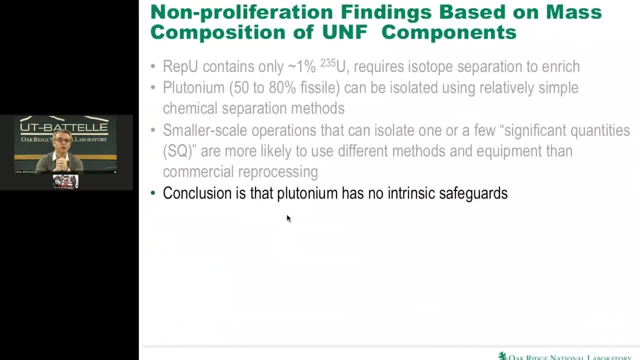 of the fuel cycles, irrespective if you're separating it or not, you still need safeguards. you still need safeguards and security for every single fuel cycle And again, guns, guards, gates and all the other things that go along with that And, as I said, since all fuel cycles. 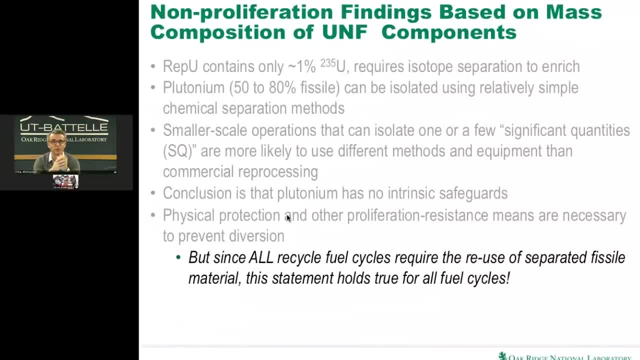 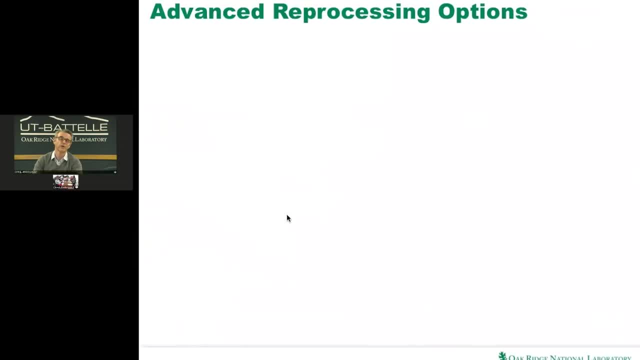 since all recycled fuel cycles and all fuel cycles end up with some form of separated fissile material, then it holds true for all fuel cycles. You need safeguards in all Fuel cycles, regardless of whether you reprocess or not. Just going back to what I said before, there are a range of options, though. 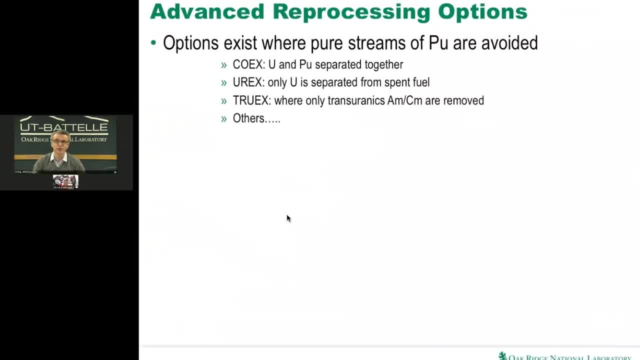 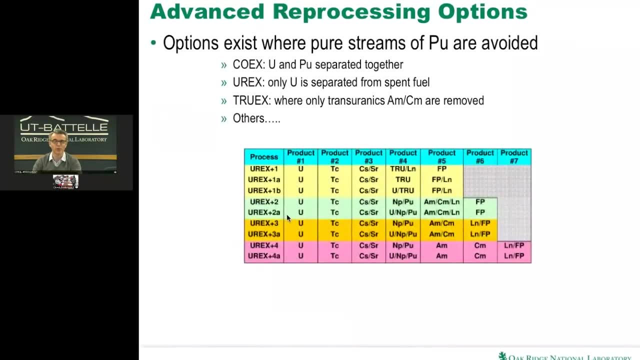 where people don't want to, for a variety of reasons, you know, safeguards reasons and so forth. they do not want people to have separated plutonium. So there are technologies to try and keep those together. And again, that's just to reiterate what I said earlier. just coming back to that, 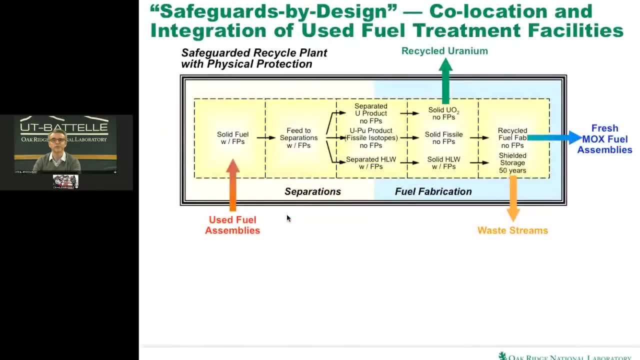 kind of full circle that these are some of those advanced techniques. But there is this concept called safeguards by design. so in a sense the chemical processing is a safeguards by design, by not separating materials into different streams and trying to keep everything together. 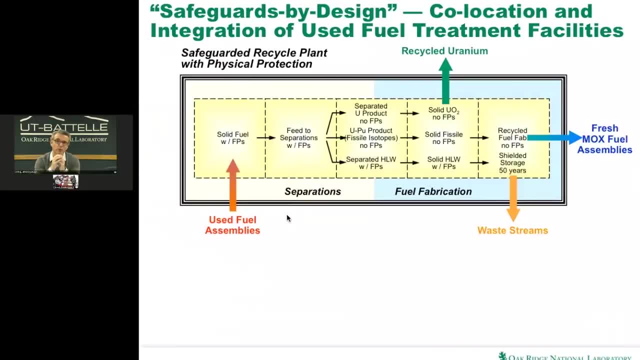 There is also a safeguards by design in this context, where if all of the processes where you could separate out and divert material, if all of those processes are kept in one facility, so that's everything from the time the spent fuel arrives to the time you shear. 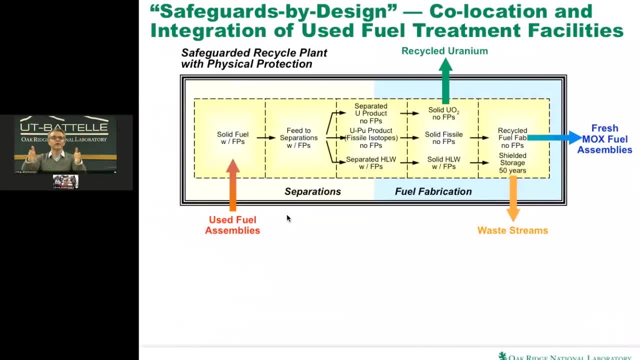 and then separate all the material and then make new fuel. if all of that is inside one controlled area, then literally from a safeguards perspective, all you need to be monitoring is how many spent fuel assemblies come in and how many spent so how many fresh new assemblies go out, and monitoring positions through all. 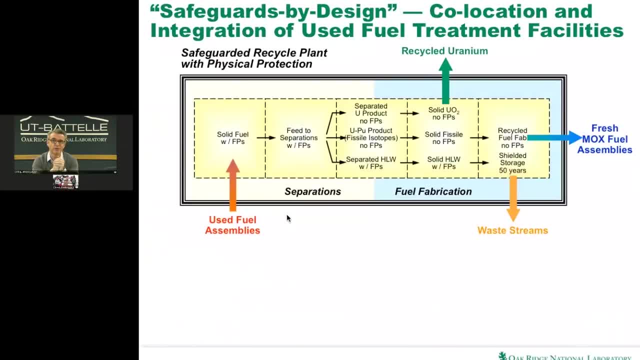 of that, then minimize the opportunity for diversion of that material. And that's what you just see here, this idea of colocation and integration of the separation streams and also the new fuel assemblies. So again, so material entry removal in the form of is large and heavy material fuel assembly. 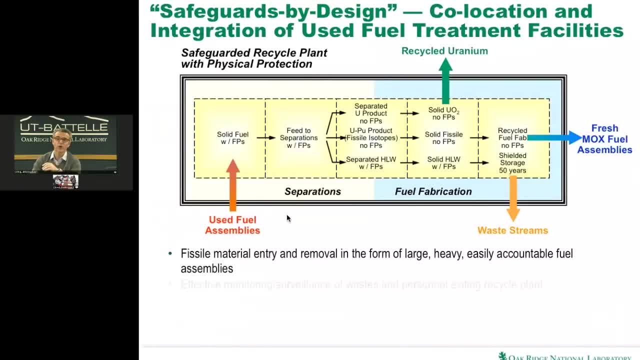 So it's kind of easy to account for, and be it hard to divert, those large assemblies. And then, as long as you are continually monitoring and surveying the wastes and the personnel exiting the recycle plant, it's easy for you to make sure that nothing's being diverted. 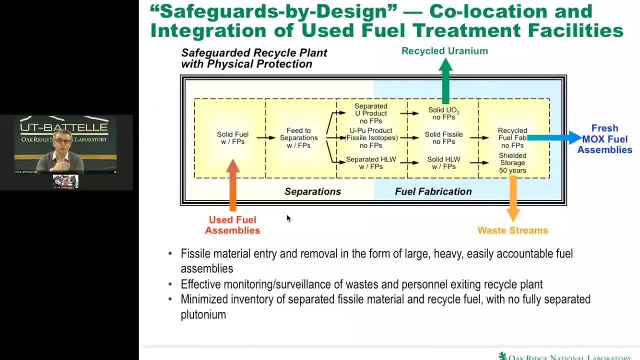 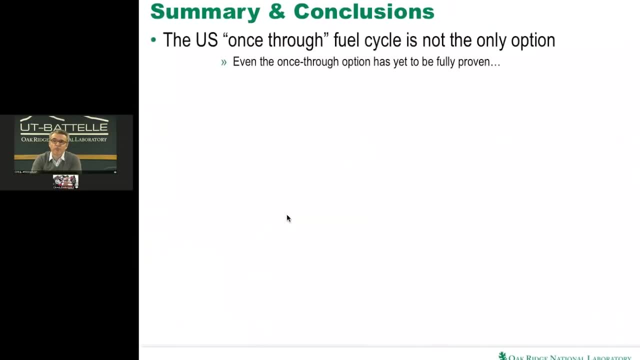 And then also you don't have fully separated plutonium. so all these potential risk elements you're avoiding by safeguards, by design, building that into the flow sheet that you start with. So to conclude, just a brief summary and conclusion: despite what people may think, the US one through fuel cycle is not the only option. 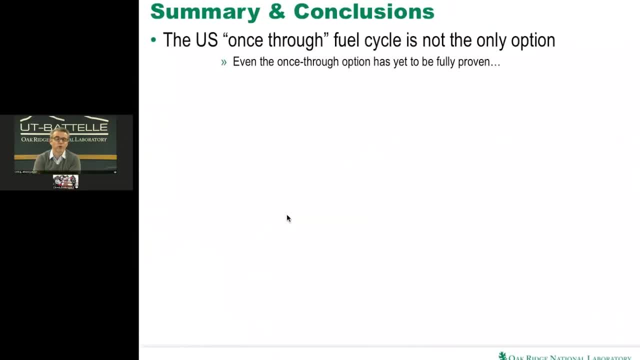 There are many other options out there. as I mentioned, many countries around the world, such as France, UK, South Korea, Japan, Germany, Belgium, many others, are doing other fuel cycles that involve separation, reprocessing and then recycle. Not everybody has taken that all the way. 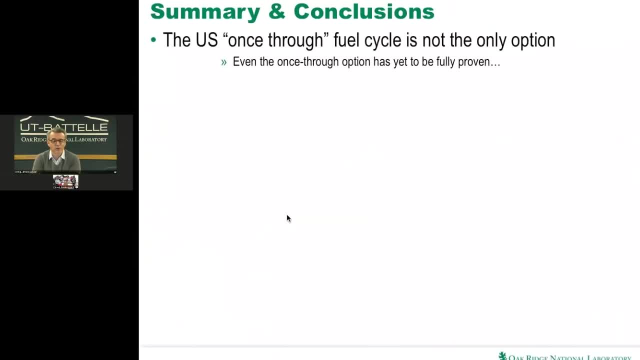 There's a way through to ultimate recycle in fast reactors. But that's the avenue, the direction that many people are going, including indeed the US, as I mentioned, looking at future fuel cycle options. But again, people often point to these advanced fuel cycles and say: well, 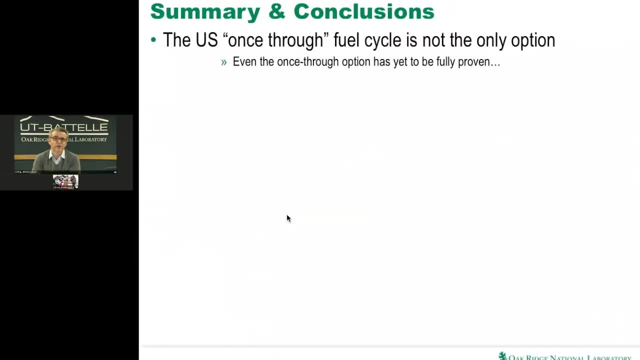 you're not able to demonstrate them, and that's true, And in fact, unfortunately, we're not yet able to also demonstrate the one through fuel cycle, because we haven't actually put any spent fuel in a repository. The closest people are Sweden and Finland. 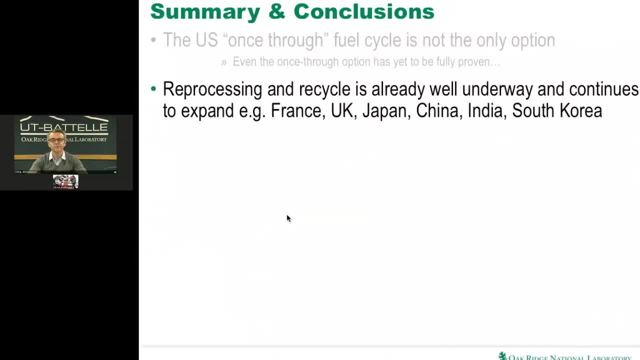 They're getting pretty close to doing that, but they're still not quite there yet. Something that I just wanted to mention in wrap up is that often people think that the US has a moratorium and is a ban on reprocessing because of the Carter. 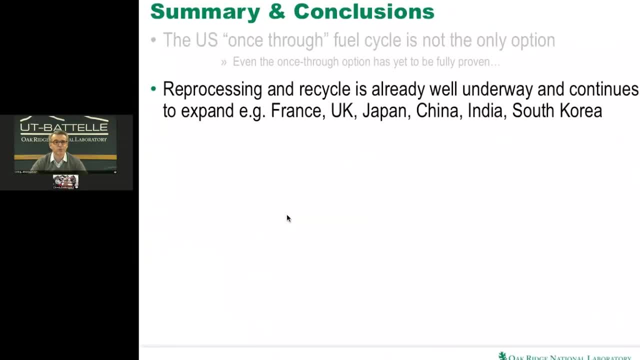 administration back in the 70s, but that's actually not true. That did happen, But in fact in 81, Reagan lifted that moratorium, And so reprocessing is actually not banned in the US. It's something that people either don't care to realize or don't follow the history. 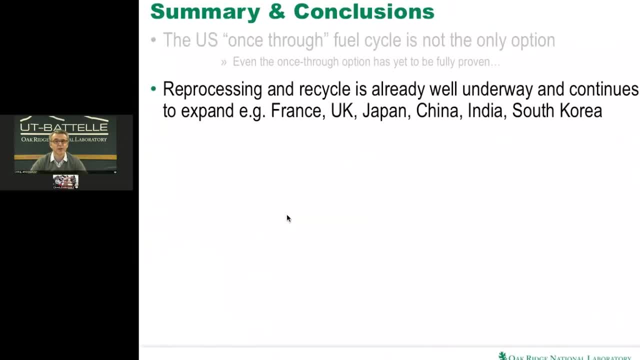 and read that part. But basically, reprocessing is not banned in the US. It just makes absolutely no commercial sense. That's the main reason. So the other thing as well is back to the Carter administration, though The idea was that if the US leads by example and doesn't reprocess, 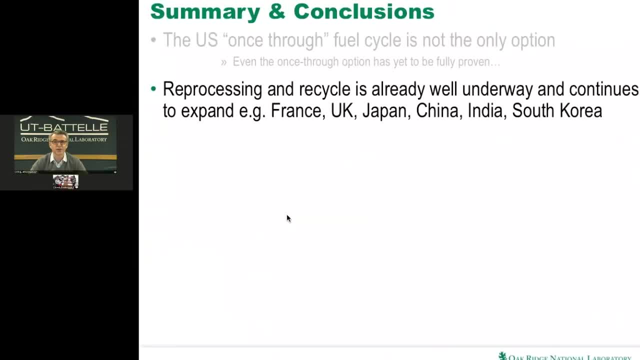 then nobody else in the world will reprocess. But, as my list there suggests, that didn't work out quite as expected because, despite the US not reprocessing, many, many other countries did reprocess And they are continuing to reprocess, And added to that list is China, India, South Korea. 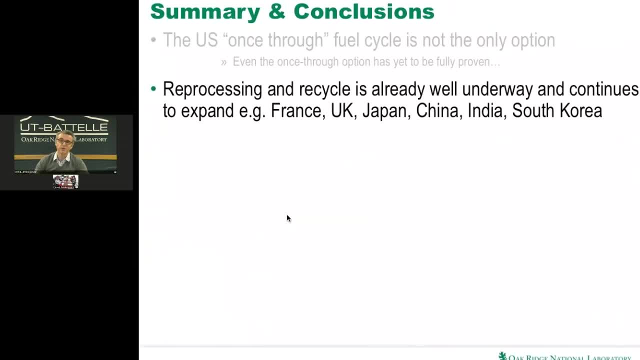 And that list is probably going to grow. So I think because of that there is potential that the US may think about reprocessing or future fuel cycles at least, because recognizing that as the world grows and energy demand grows, for nuclear at least, then it puts a new pressure on uranium ore and therefore it makes sense to recycle. 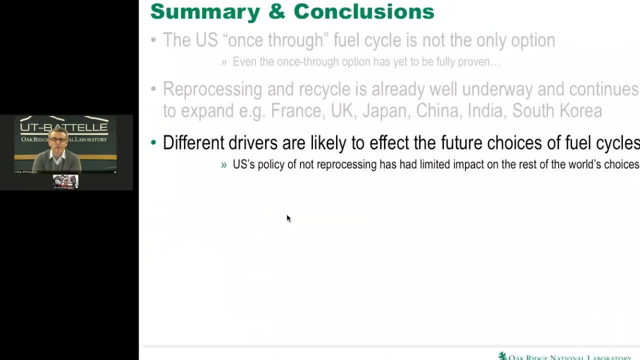 potentially, if the, if the economics is right, There are a huge range of different drivers that are likely to affect the future, the future's choices, As I mentioned. as I said, the US policy on not reprocessing has not limited the impact on the rest of the world's choices.